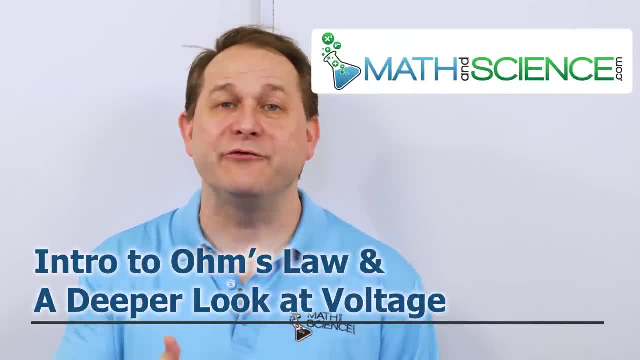 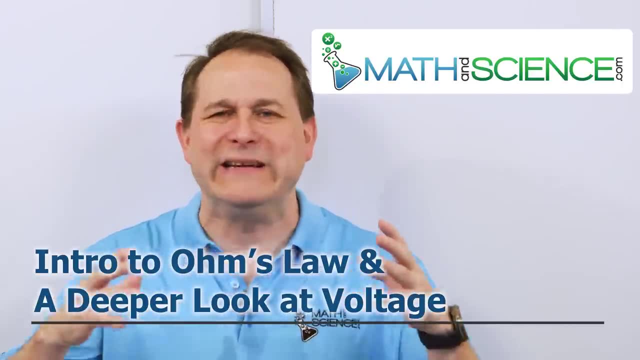 circuits. Hello, welcome back. Today we're going to have an introduction to Ohm's Law and also a deeper look into voltage. These two concepts are absolutely essential to do anything in circuits. That's what we're going to conquer today. I want to start out with a question. This is a large 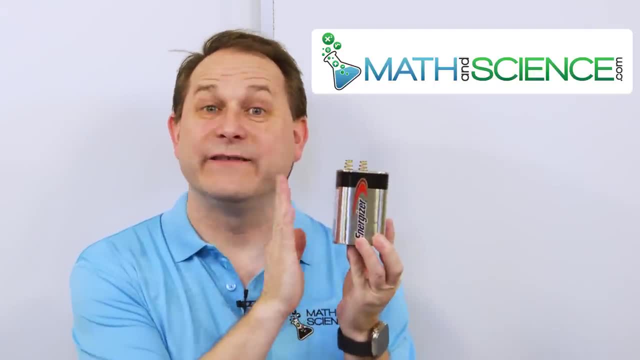 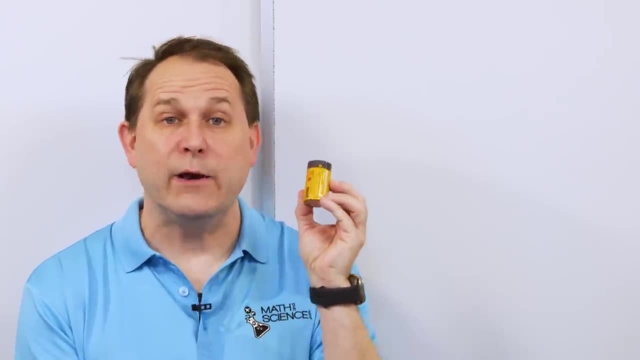 battery Some of you may or may not have ever had occasion to use. It's six volts. Six volts: that's the voltage for this battery. All right, this is a D size cell. It's a one and a half volt cell. right, This is a C size cell. You can see. 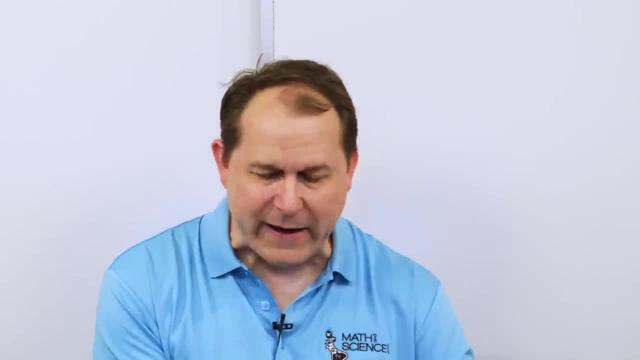 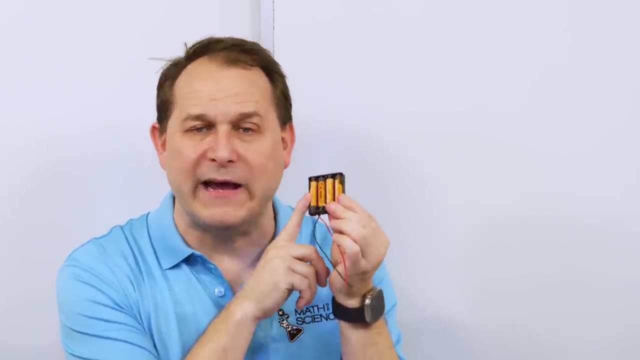 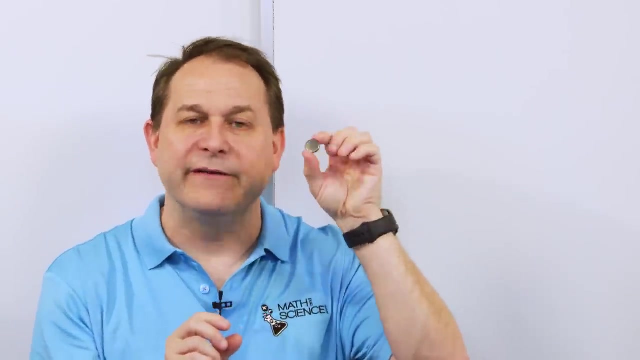 the difference. It's also one and a half volts. You see the pattern here. This is a double A cell: one and a half volts. This is four of these, what we call triple A cells, each of these one and a half volts. And these little bitty guys, these little tiny little flat batteries, three volts. 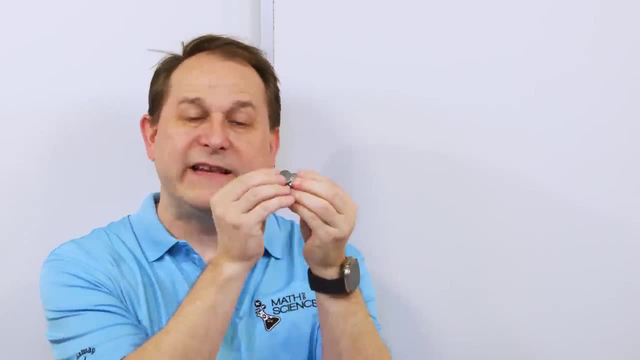 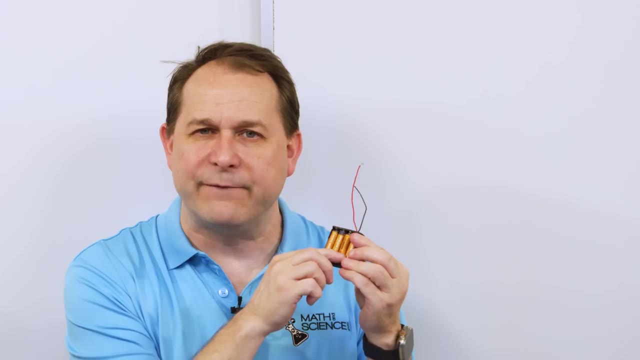 each. So if I put two of these three volts batteries together, I can get six volts, which is the same voltage as this. If I know that each one of these batteries is one and a half volts, if I stack them in the right way, I can add up to six. 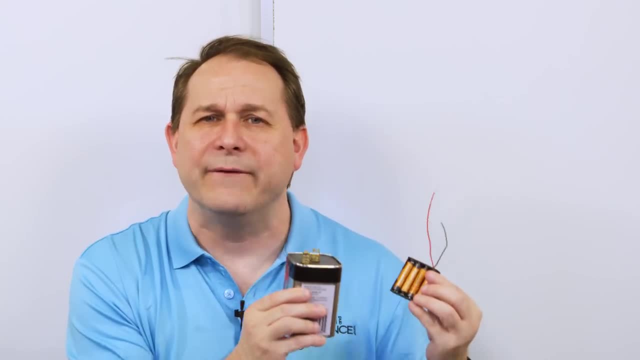 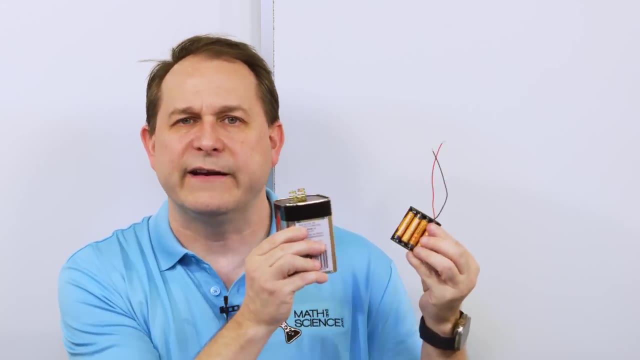 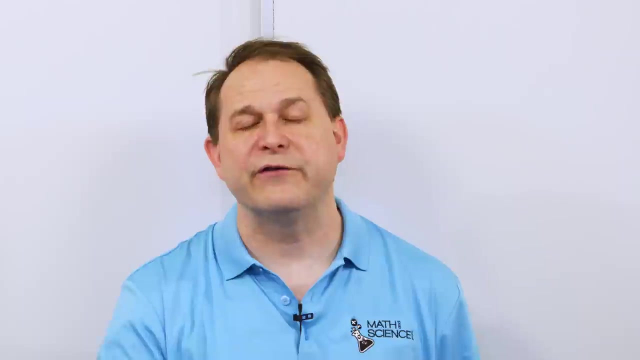 volts, the same voltage as this. Why do we have so many different size batteries that are really the same voltage? If this is six volts, and this is six volts, what is the difference between these two batteries? So, in order to answer this, today we're going to have to talk about the difference. 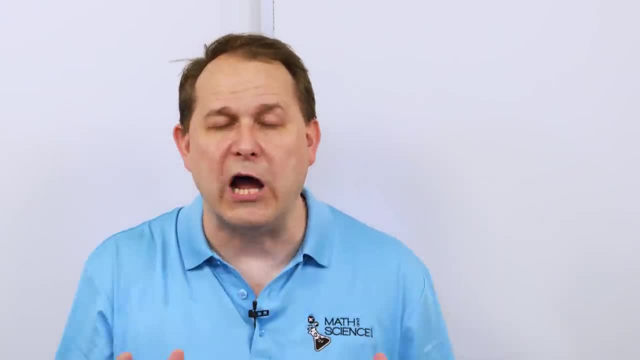 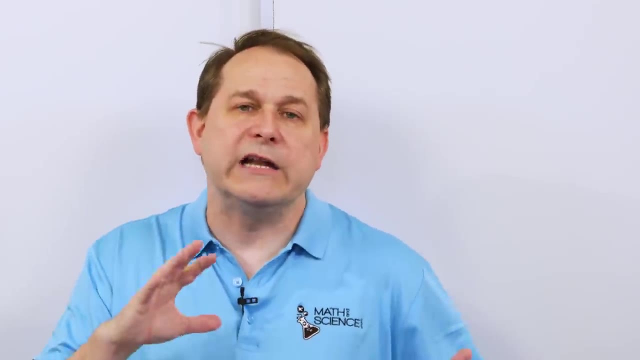 between these two batteries. In theory, we have what we call Ohm's law. It's the most fundamental equation and law that you have to master in order to understand electricity, But we're going to apply it. understand a deeper look into voltage using Ohm's law, And then we're going to use it. 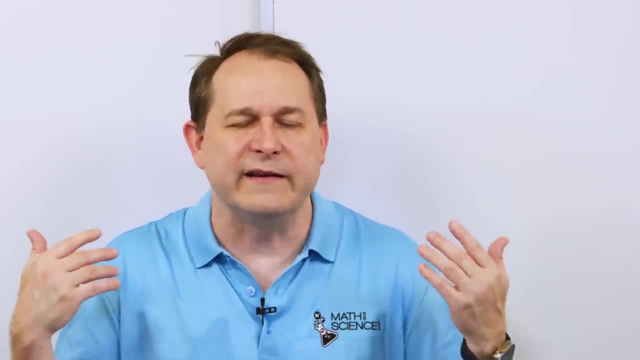 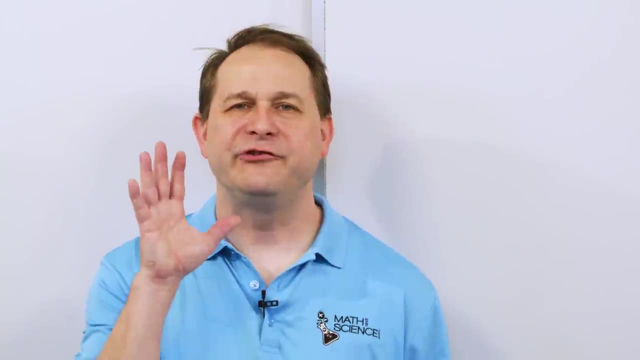 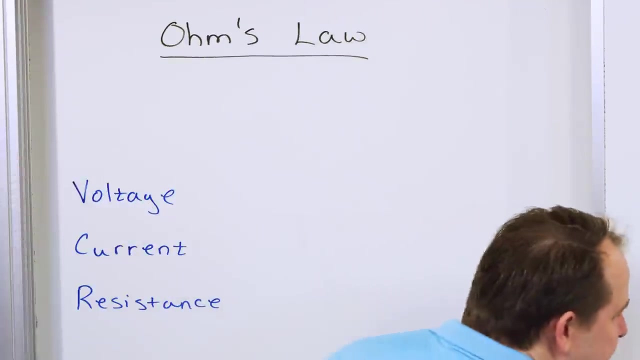 to try to understand the difference in these voltage sources. So this lesson is all about voltage sources- trying to understand voltage a little bit deeper. Let's get started right now. So let's jump right in by diving into Ohm's law. We're going to talk about Ohm's law a lot, but I need to introduce it here in order for us to make 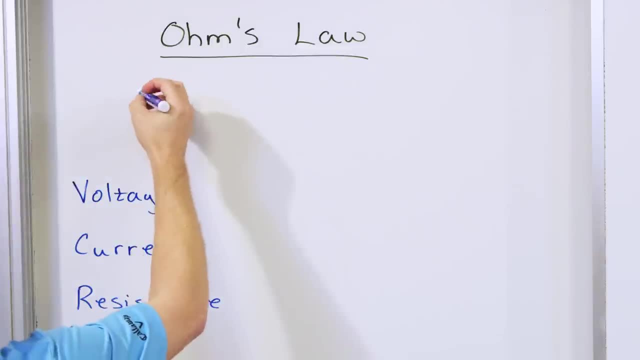 any progress at all. Ohm's law is a very simple algebraic equation. The three variables of interest are voltage, current and resistance, which we've talked about in the past, And Ohm's law states that the voltage across any passive circuit element- I'm going to talk about what a 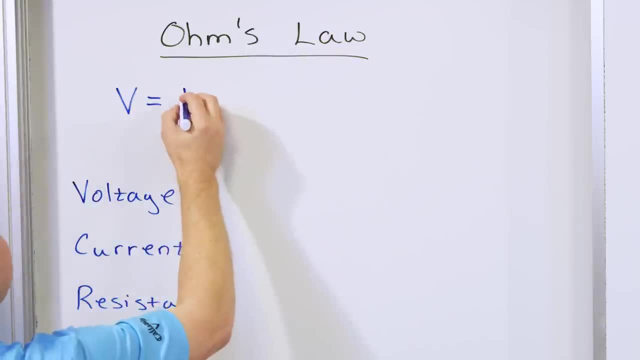 passive element means, in just a second, the voltage across it is equal to the current passing through, the electric current passing through that object multiplied by its resistance. Now this applies to all resistors. Right now we're going to basically be talking about resistances. 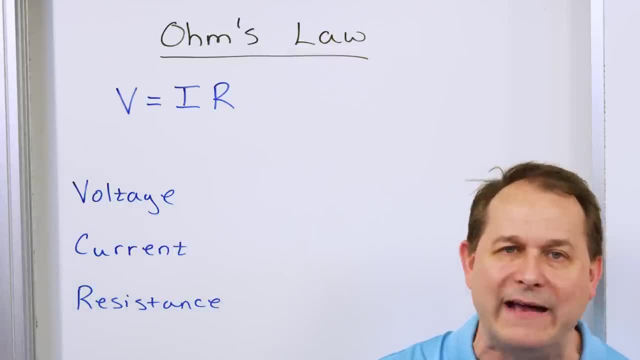 We have to modify it a little bit when we talk later about capacitors and inductors, and we have to totally change the discussion completely when we get to non-linear components, which are diodes and transistors. We have to kind of modify things later, But for now I want we to 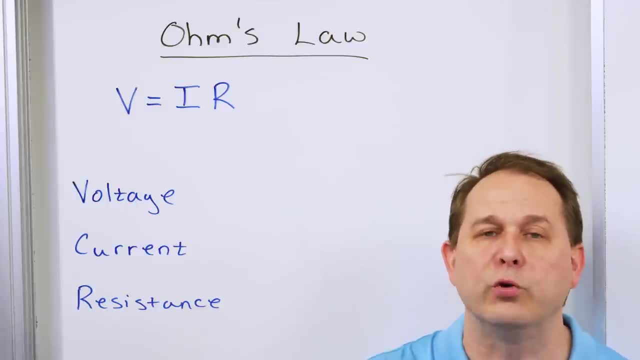 I want you to discuss Ohm's law with me in the context of only resistors. We have to learn resistors first. It's the easiest thing to understand. Now, if the voltage across a resistor is equal to the current flowing through the resistor times its resistance. this is an 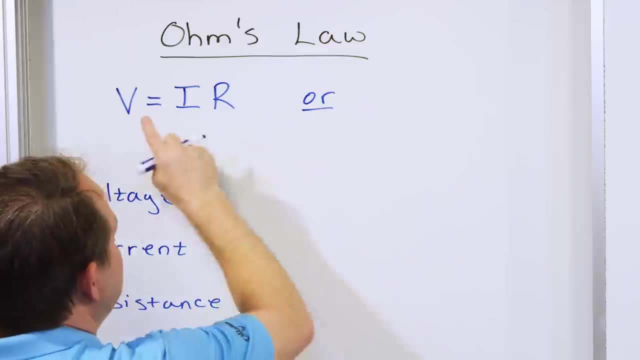 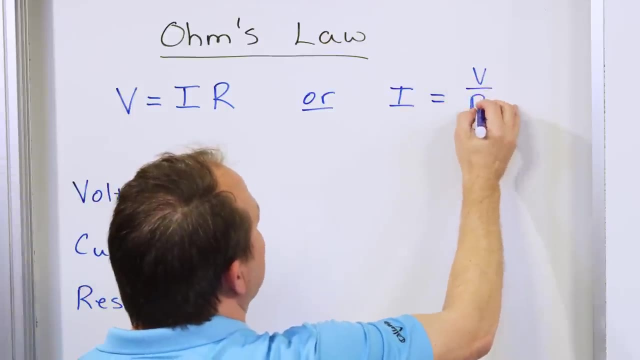 algebraic equation that you can solve for whatever variable you'd like. Another common way- or a very useful thing way to write it- is that the current at I is equal to V over R. Just take this equation, divide both sides by R and you'll be left with: I is equal to V over R, which is what we have here. 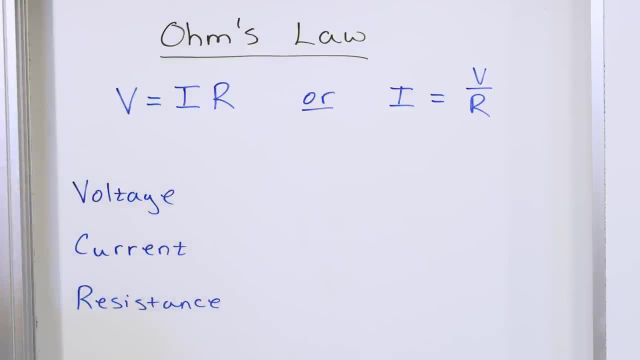 These two forms of Ohm's law are what you will typically see in books and they're exactly the same. It's not that one is better than the other. It's just like two sides of the same coin. It represents the same exact relation. All right Now. we mentioned in 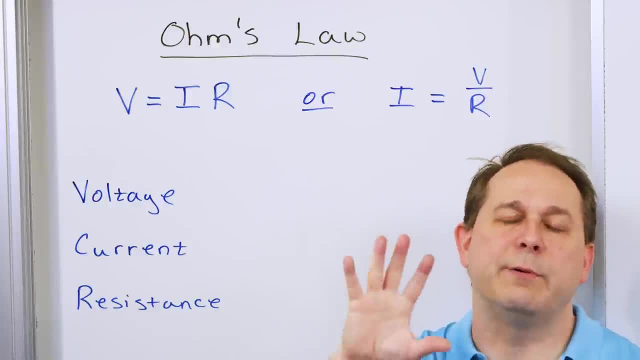 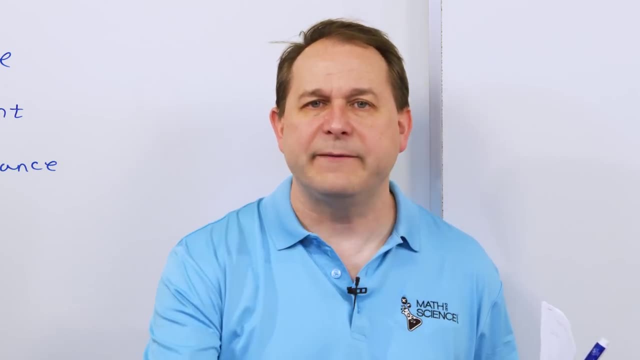 the introductory lesson that we have voltage, current and resistance, but we need to solidify it more. What does voltage mean? Voltage is the push in an electric circuit. This battery is providing a physical push to the electrons in the circuit. The push is coming from a chemical. 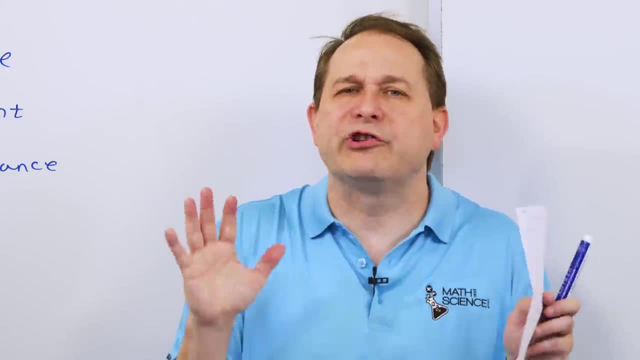 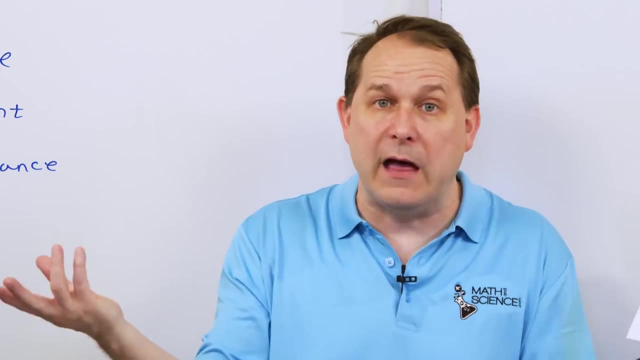 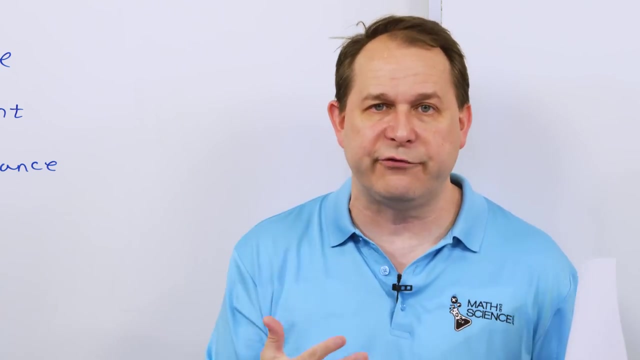 reaction. Ultimately, the push comes from what we call the electric field. you know from base science. You know two electrons repel each other. Light charges repel Either two protons or two electrons. they repel and opposites attract. That electric force, ultimately, is where all electricity. 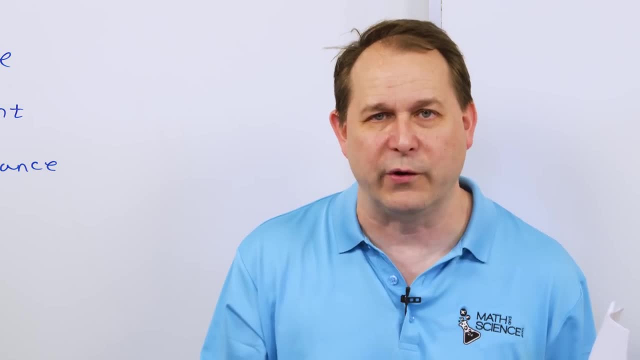 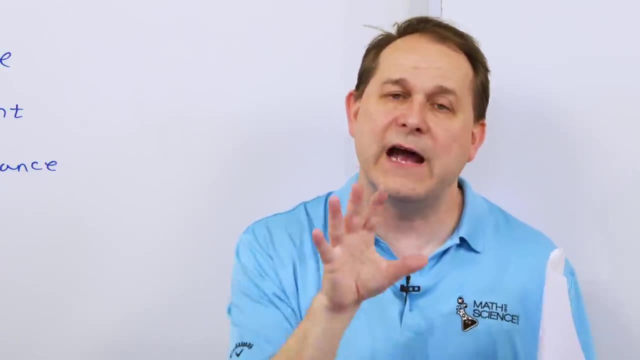 the force to push the electricity comes from. It comes from the electric force In a battery. it's coming from the chemical reaction that's wanting to push electrons out of the terminals and back around to the other side. We'll talk a little more about batteries. a whole lot in. 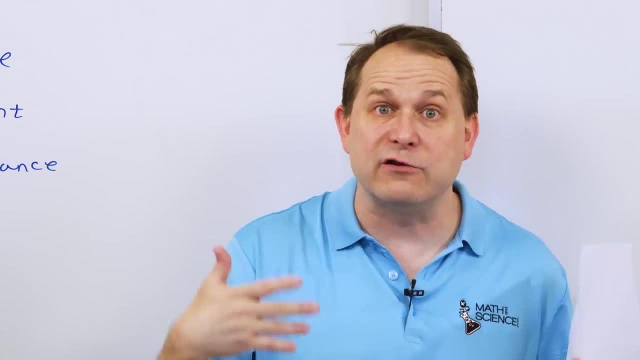 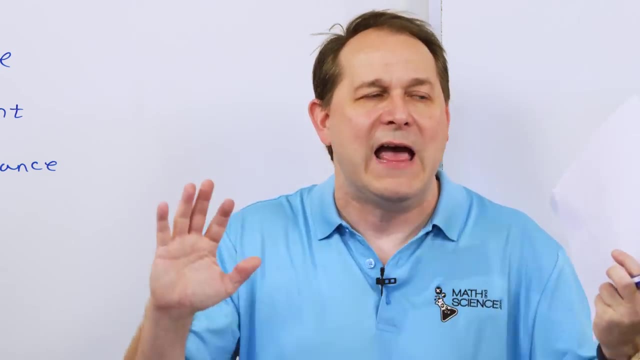 just a second. But of course we have electricity that's generated by nuclear power and other means. They're all generated various ways, but ultimately the voltage that comes out is the push. How much push do you have that's causing the electricity to flow? 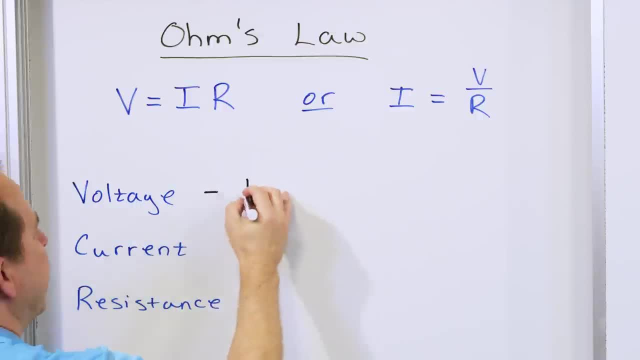 So when we talk about voltage, I want you to always replace it with the word push in your mind, if I can make this correct. Push, It's the push, right. The electric current itself is what is actually flowing. It's what we call the flow. We're going to talk about the definition of current, very 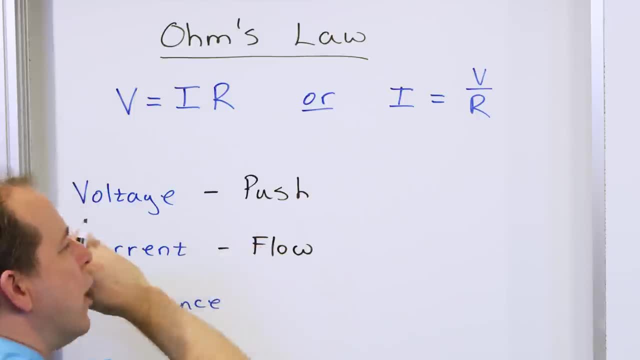 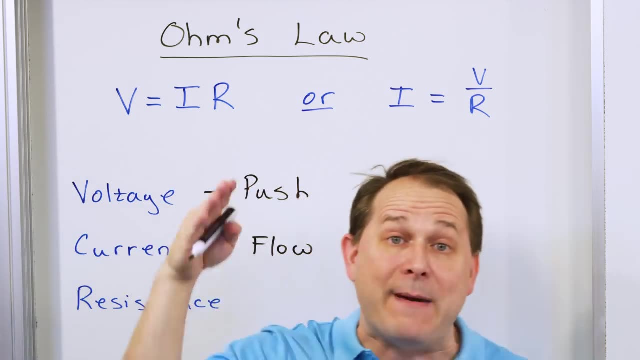 soon. It's literally how many electrons per second you can generate. It's literally how many electrons per second are flowing past a point. It's literally like the water flowing in a river, whereas the voltage is maybe the height of a mountain. When we talk about voltage, 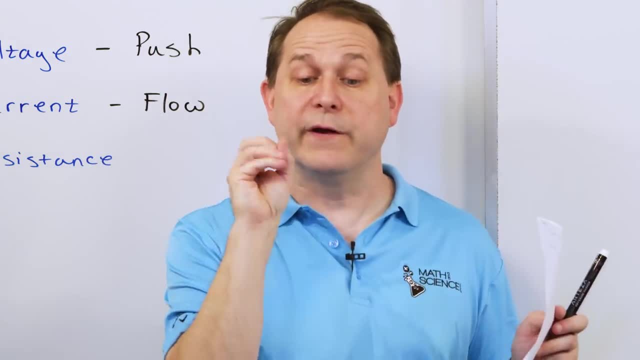 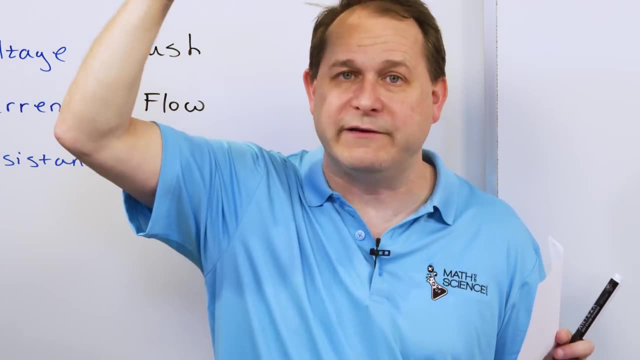 I want you to picture a mountain. You're standing on the mountain top and you can throw rocks off the mountain top because you're at a high potential. We call it potential energy above the ground in physics. When you throw the rock, it accelerates down the side of the mountain. 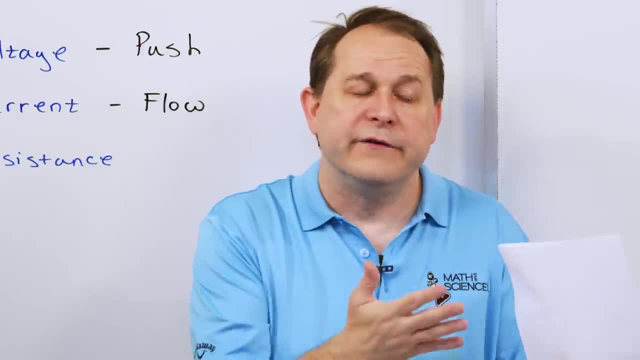 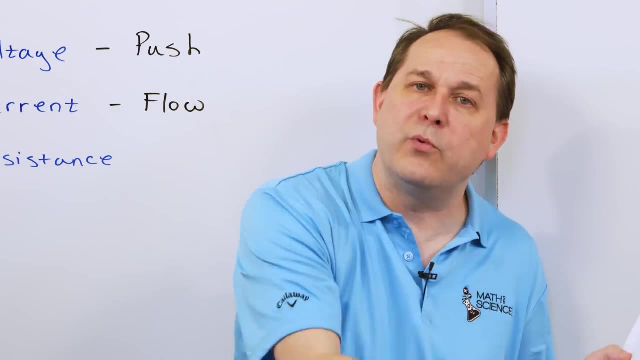 When it gets to the bottom of the mountain, it has no more potential anymore, so it eventually stops rolling right. When you have a battery, you're at the top of the mountain and it's pushing the electrons, But when they get it back around to the other side, 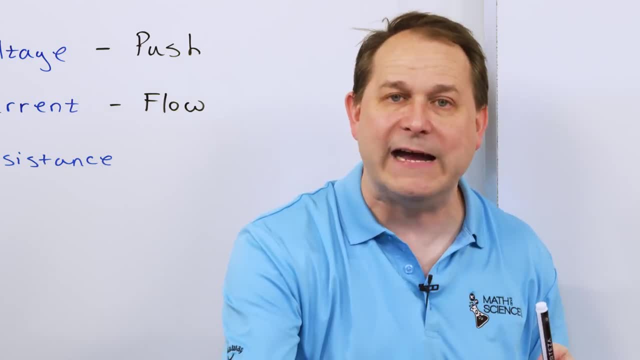 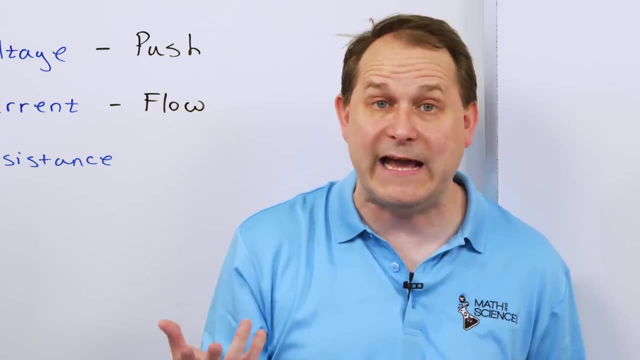 when they go out of one terminal and get back around going to the other side, then they have lost all of their potential energy and then they go back into the battery to be accelerated and pushed out the other side again. So it's very much like a mountain, The higher you. 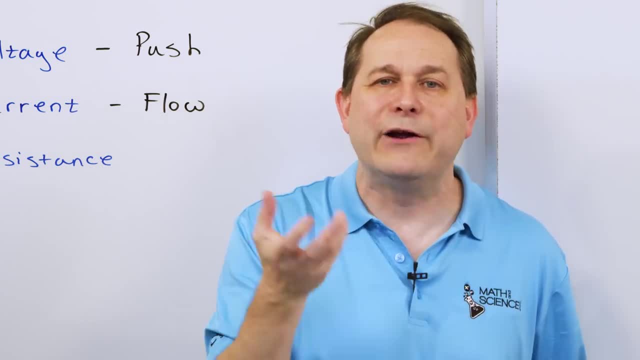 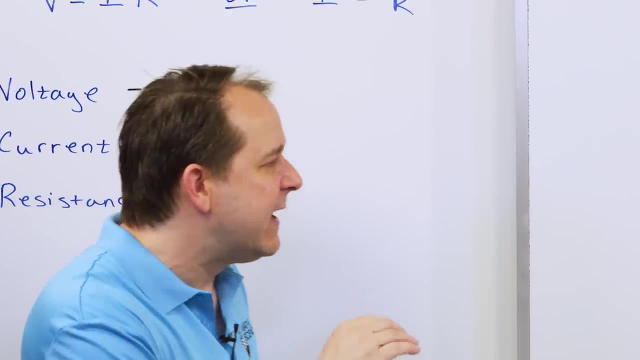 are above the ground, the more potential you have to do work, the higher the voltage in a battery. So if you're going to push at the top of the mountain, what is flowing is the actual electric current And if there are any obstacles in the way or resistors, in this case, we call it the 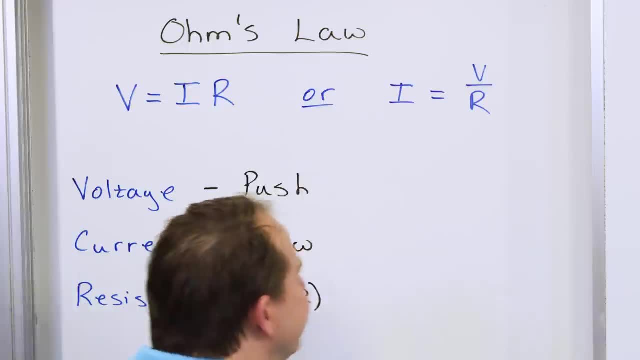 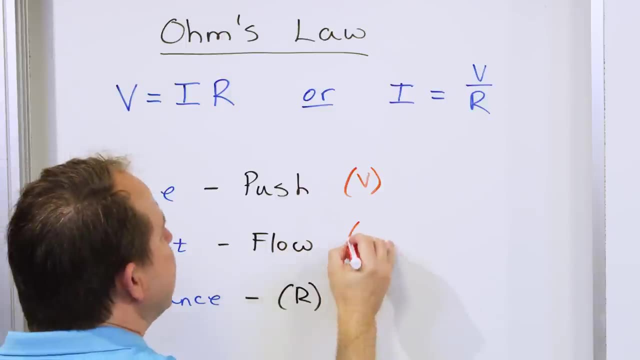 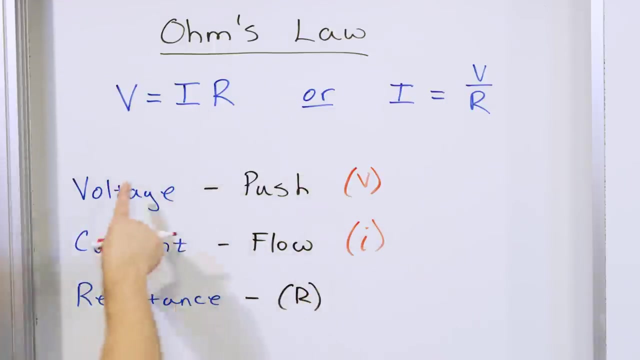 resistor, the resistance R. Now I want you to remember- we're going to go over units again- voltage: The voltage is in volts, of course, The current is I- You can use capital or lowercase i- And the resistance we usually call R. So V equals IR. That's these three variables, right? 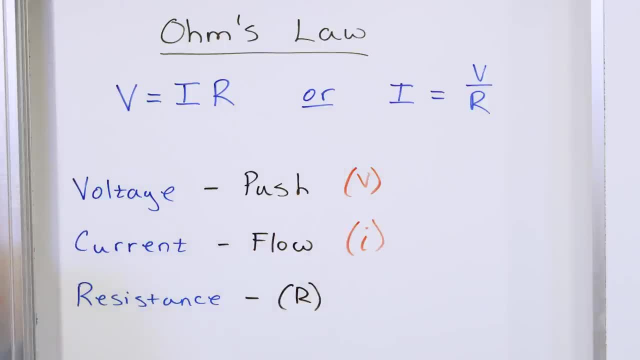 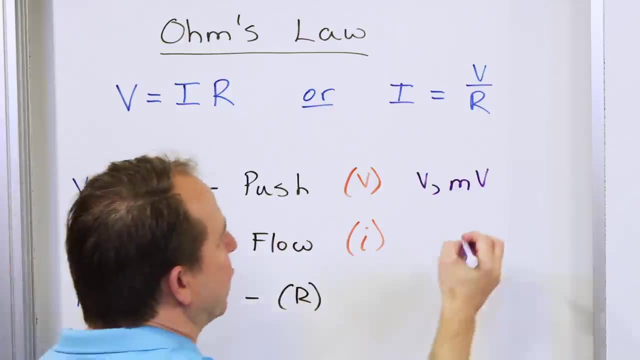 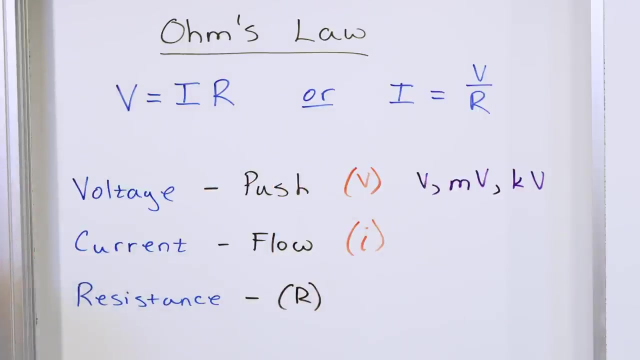 Right here. Now the base units of voltage are volts, But of course we might instead talk of millivolts, That's one one-thousandth of a volt. We might talk about kilovolts, which is thousands of volts, But it's just a modification of the basic unit of a volt. 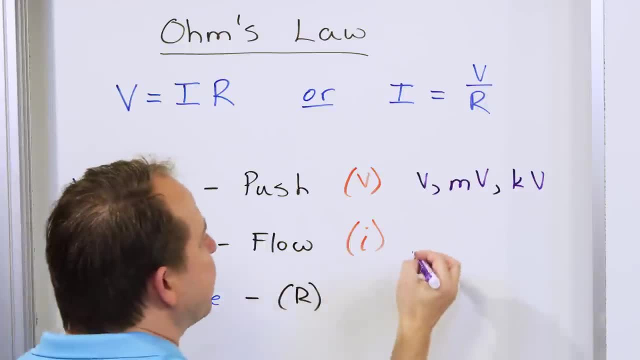 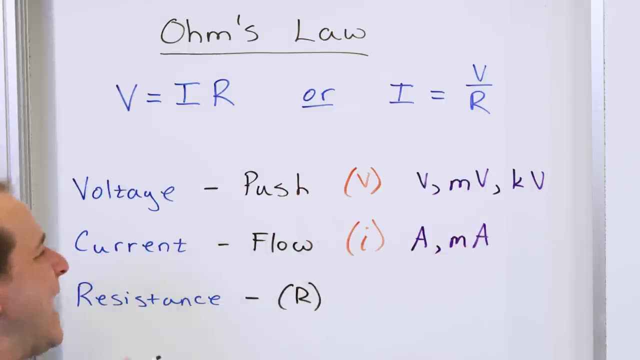 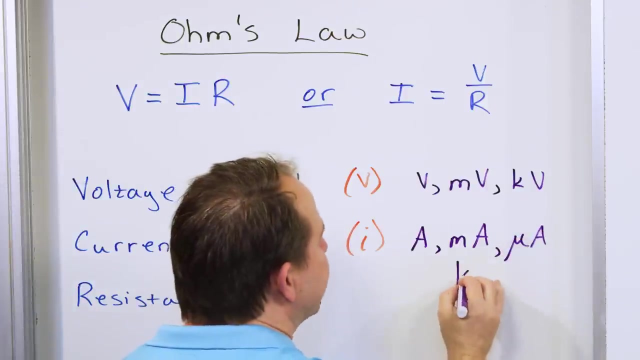 Same thing for current We might have. the base unit of current is called the ampere, which we abbreviate A, But we might instead talk about milliamps, which is thousandths of an amp. Right, We might talk about microamps, which is millions of an amp, And we might talk about. 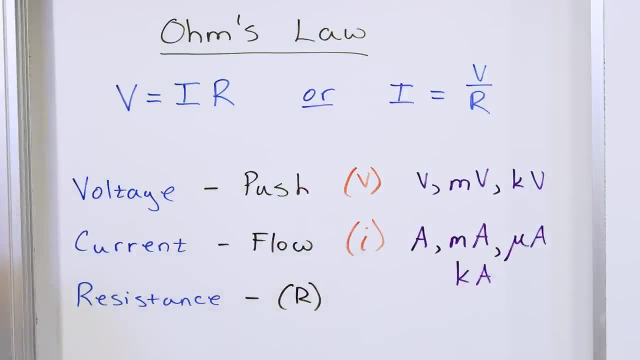 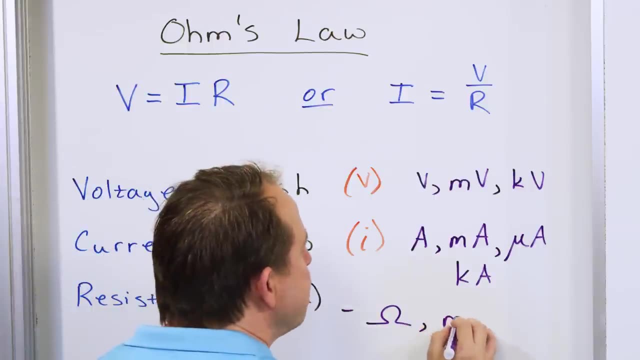 kiloamps, which is like thousands of an amp Right In terms of resistance. we might talk about ohms. We use the symbol omega for ohms, But we might modify it. We might talk about milliohms. We might. 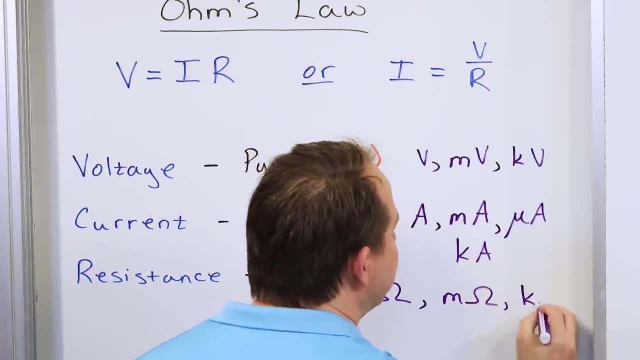 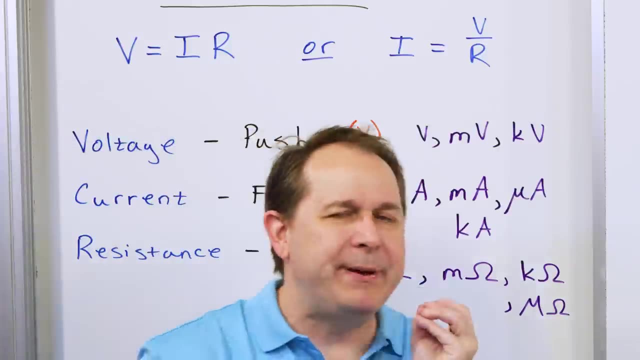 talk about microohms and nanoohms and so on, But it's more common to talk about kiloohms or even megaohms. All right Now, this is all stuff we've talked about in the past, But it bears repeating. 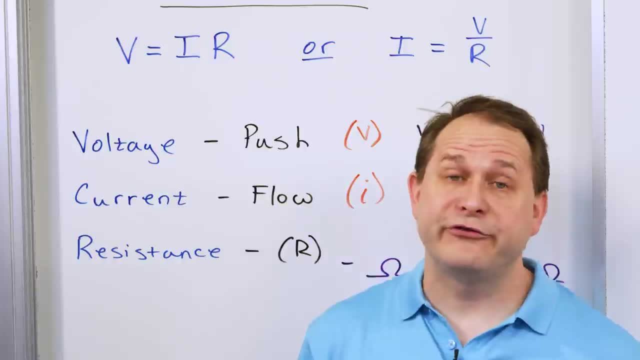 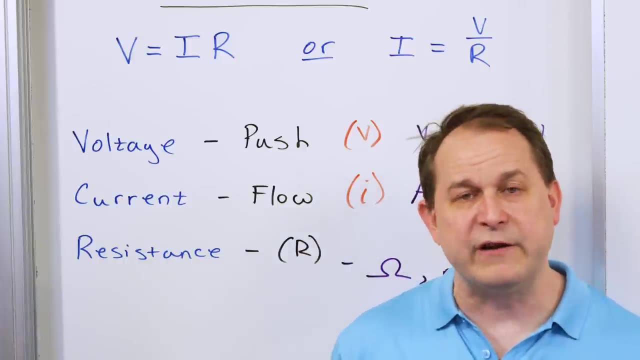 because you have to understand the definitions When we talk about a circuit. if somebody tells you, hey, that circuit has a million volts of electricity flowing through you, you know that this person does not know what they're talking about, Because voltage does not flow. What do? 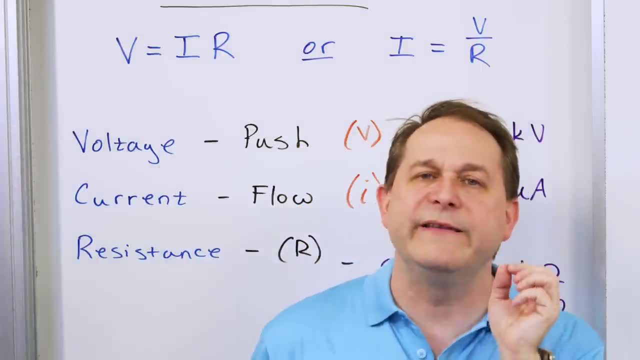 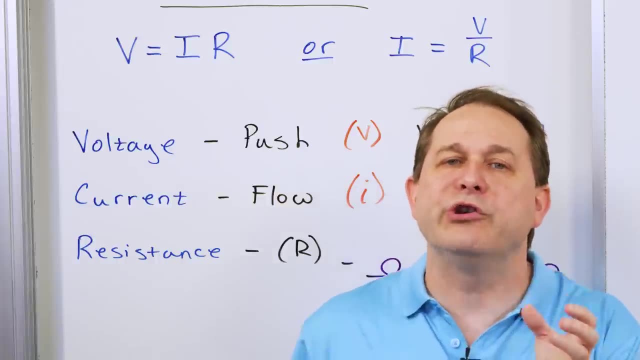 we say flows, The current flows. The current is the only thing that flows. It's literally the electric flow of charges in a closed path. The current flows, but the push required to start the flow or to continue the flow is the voltage. And if there are, 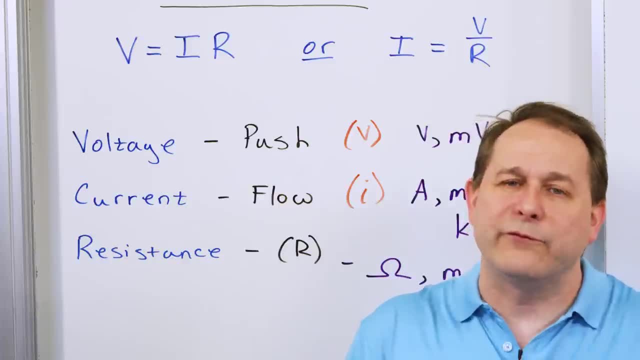 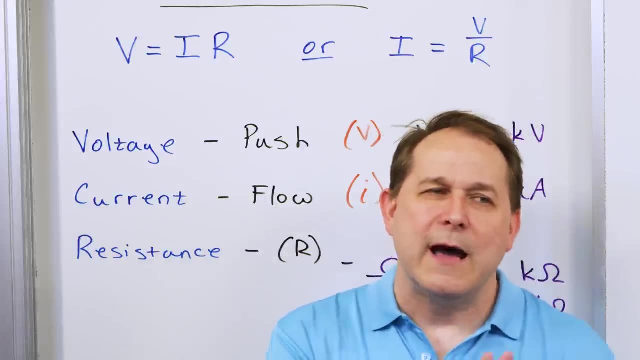 any resistors in the way it tends to reduce the amount of current. That's why it's called the resistance All right, And the interplay between these three variables we call ohm's law. Now we want to learn about all of these things in practical detail. We want to build some circuits. 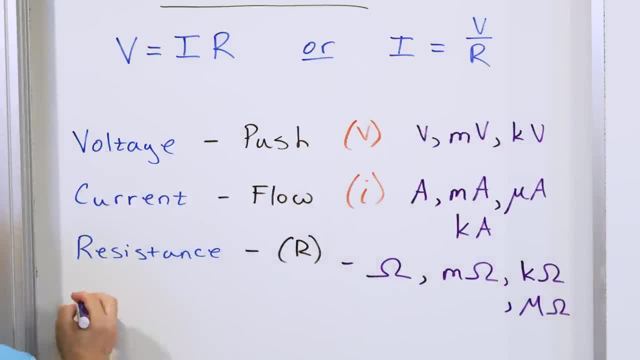 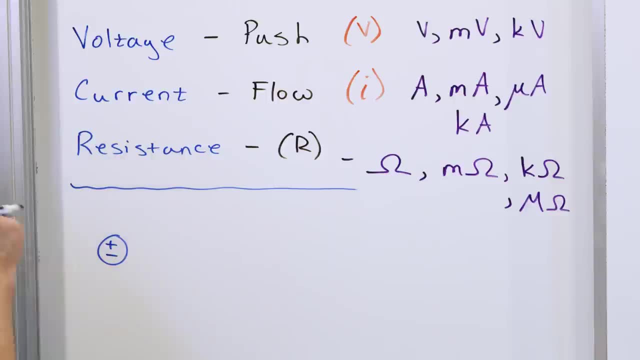 So let's take a theoretical circuit, the absolute simplest circuit that I could possibly think of. Right, We're going to have a voltage source. There's many symbols for a voltage source. I'm going to write it like this: plus, minus, And we're going to say that this voltage 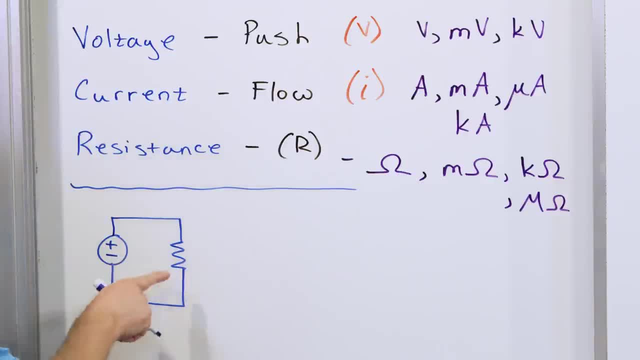 source is connected directly in the path with a resistor. This is a symbol for a resistor And in this case I'm going to say that this voltage has a voltage of one volt and the resistance has a resistance of 10 ohms. Now I want to ask you if I take a one volt. 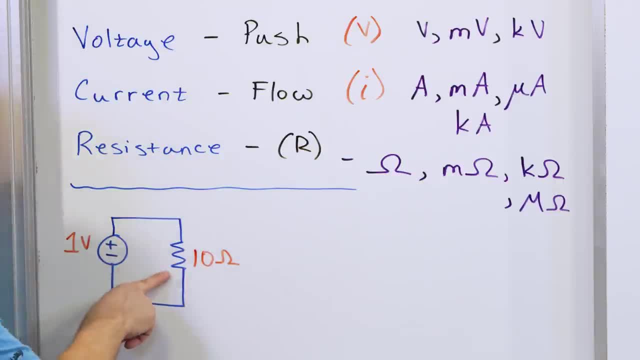 source and I connect it directly in the path with a single element, which is a 10 ohm resistor. how much electric current will flow? We know that there will be current flowing here, going around to the other side. Remember, we know the electrons are coming out of the negative side. We 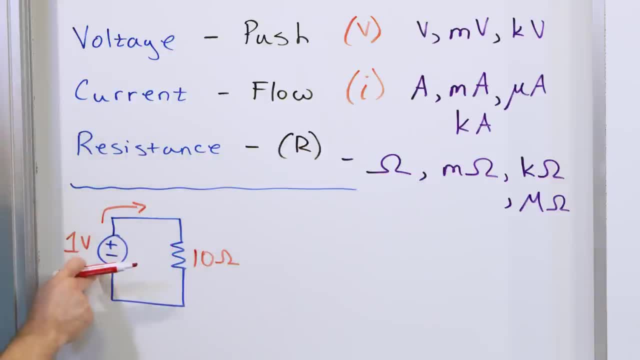 know that, but we talked about in the last lesson that, algebraically, since electrons are negative and they are coming out this side, mathematically it's the same thing as talking about the opposite current. We call the whole current coming out of the positive side and going this way. 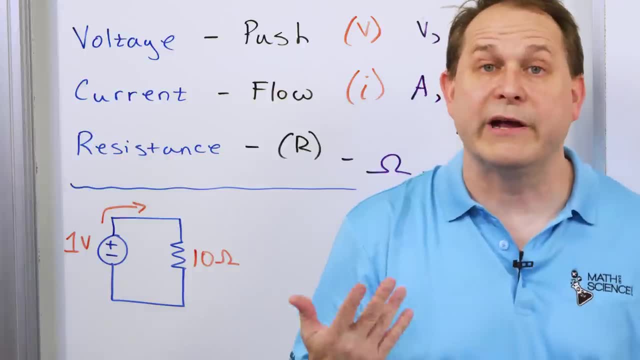 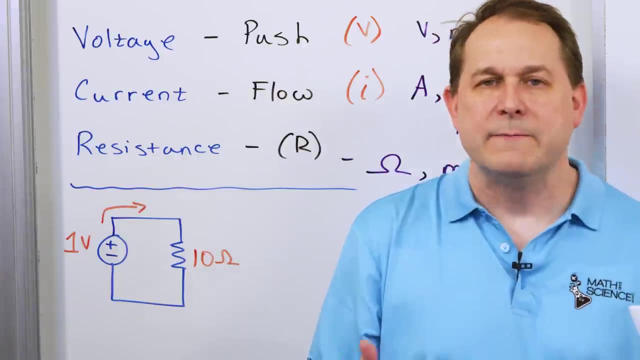 Now, I don't care personally what you do, but when you take electrical engineering classes, we always talk about the positive current flow. It makes the equation simpler because there are no negative signs. But if you want to think about electron flow, that's fine. I'm just. 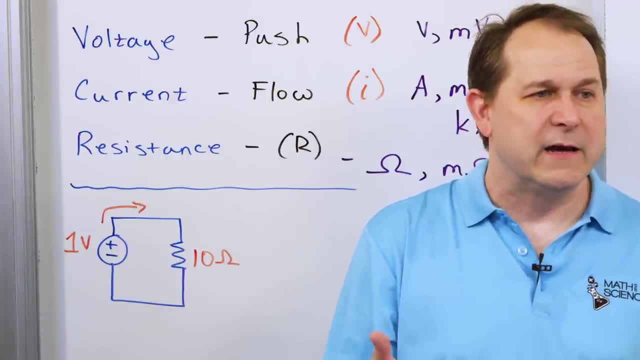 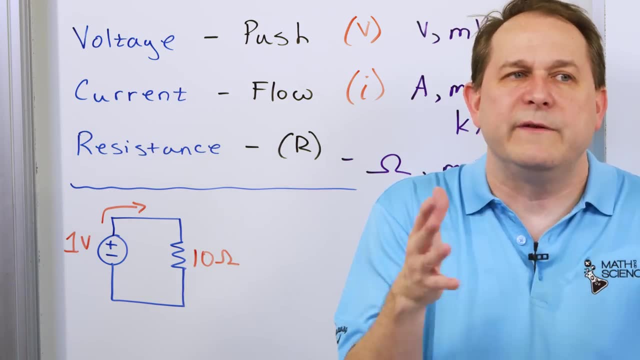 telling you that they're mathematically the same thing. It's like positive 3 is the same as negative, negative 3. Put two negatives together, you still get a positive 3.. You can write it different ways, but it's the same thing. So this is our circuit. How do we determine the current? 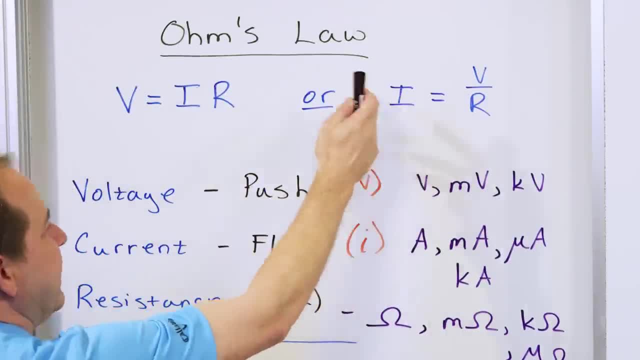 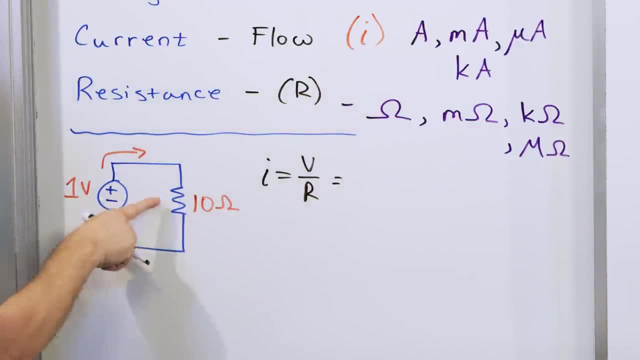 flow, We go up to Ohm's law. You can use either form you want, but we're trying to find the current. so we can say that I is equal to V over R, But we know that the voltage across this resistance is one volt, And we know that this resistance is one volt And we know that this. 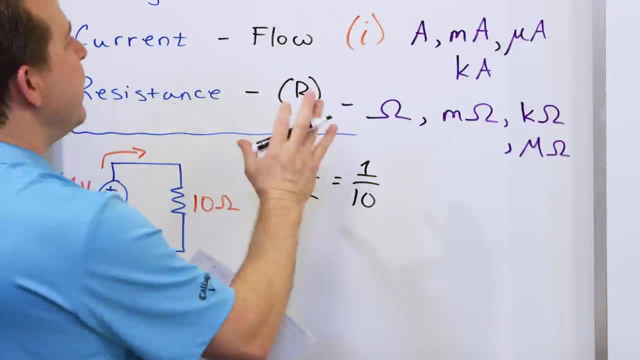 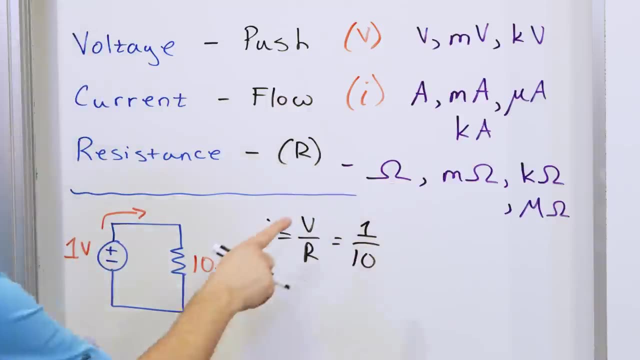 resistance is 10 ohms. Now we're working in the base units. We know that the base units are voltage in volts and then amps is the base unit and ohms is the base unit of resistance. So if I know, I've put a unit of volts in here and I know I've put a base unit of ohms here. 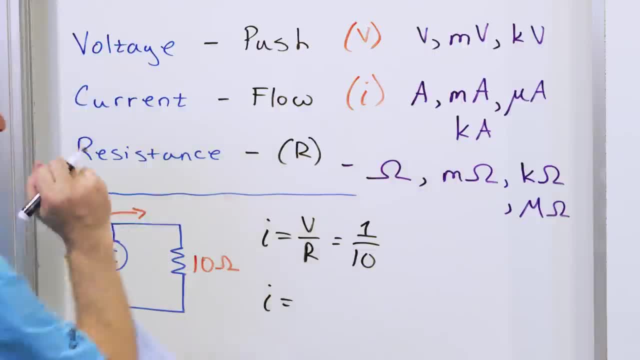 then I know that the current, I calculate is going to be in the base unit of amps. So what's 1 over 10? It's 1 10th or 0.1 amps. So what we expect is we expect if we connect a. 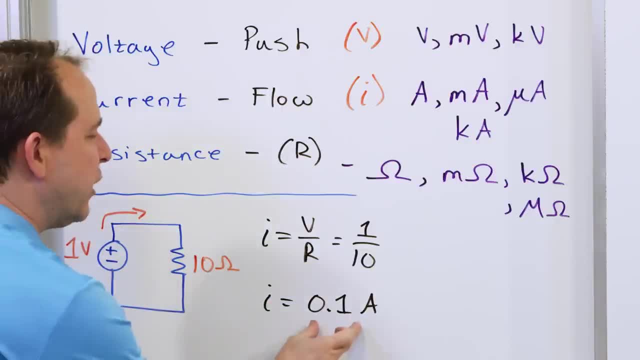 1-volt source directly to the current. we're going to get a current of 0.1 ohms. So what we expect is, across a 10-ohm resistor, that there should be a current flow of 0.1 amps, which is 1 10th of an amp. 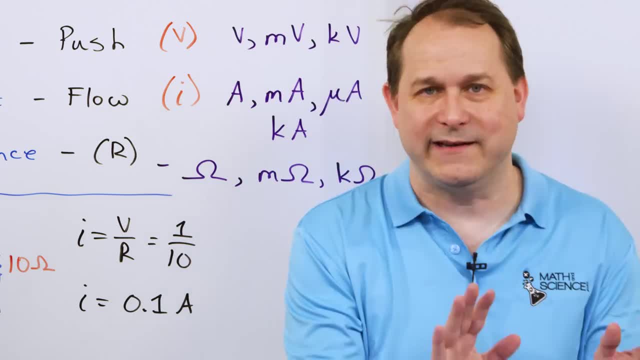 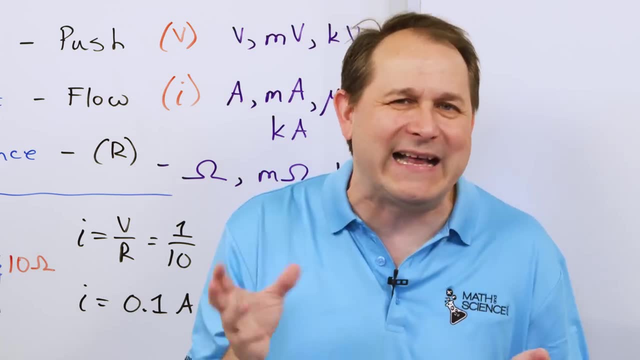 So here is where we have to go: from theory to reality. In reality, you're not going to be able to get exactly what you write down on the board because your voltage source is not going to be exactly at 1 volt, Your resistance is not going to be exactly at 10 ohms, And the measurement 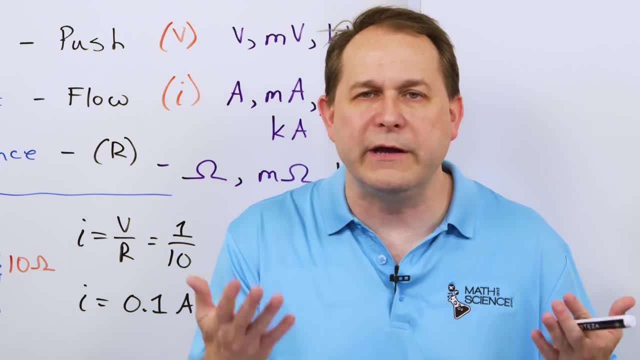 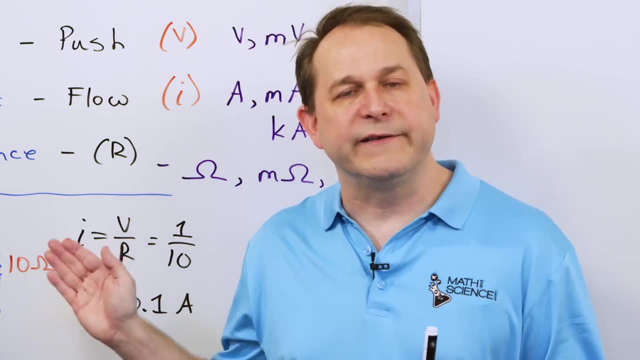 apparatus, whatever measurement apparatus you're going to use- an ohmmeter or voltmeter or whatever- is not going to be infinitely accurate, But you should still be able to convince yourself that you're getting something close enough to this, that we're representing reality. So, what we're going to do, we're not going to use batteries. 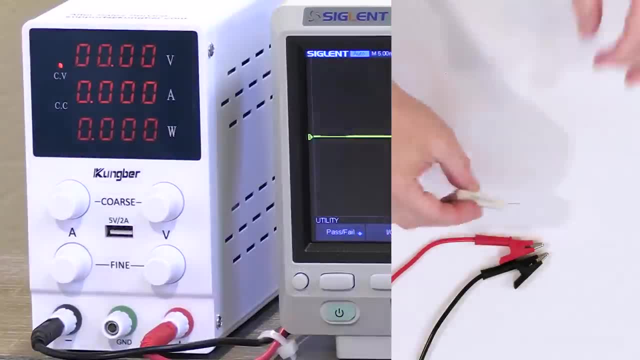 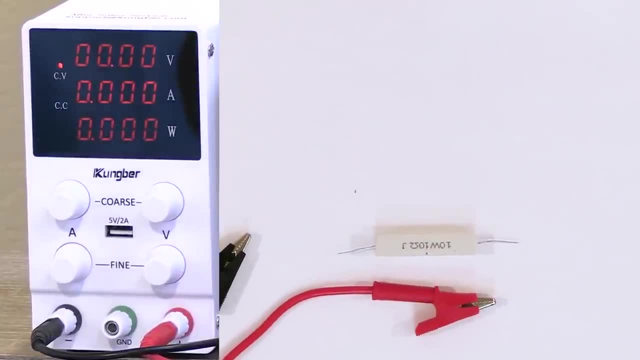 yet We're going to use my voltage source right here and we're going to connect it across this resistor. Now, this resistor is a physically large resistor. In the last lesson I worked with resistors that were very, very small. We're going to have a whole lesson on resistors and 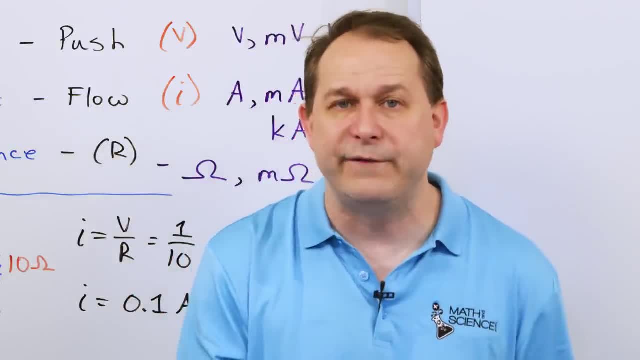 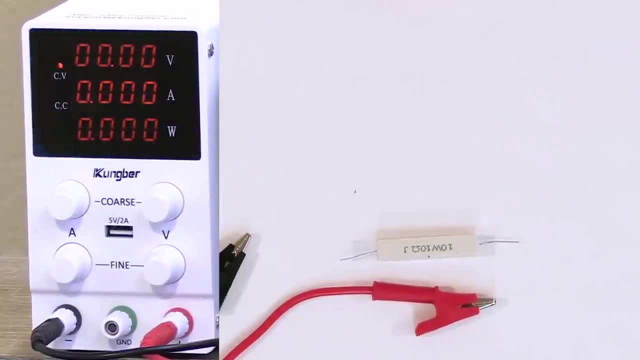 resistance very soon. But just know that the reason I'm using this very large resistor physically. notice it says 10 ohms printed on here and it says 10 watts. The W is watt. We haven't talked about power yet. 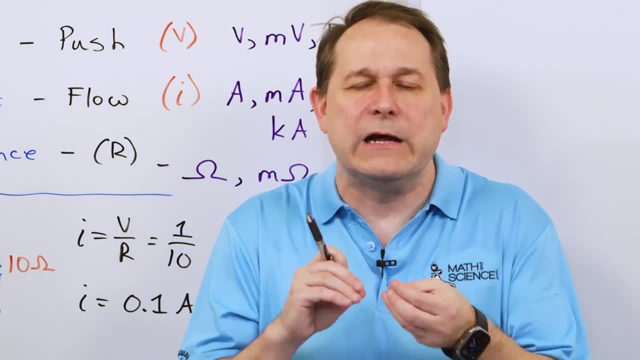 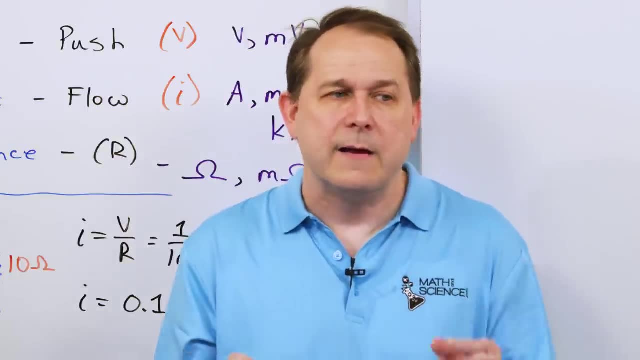 but this resistor is physically large so that it can absorb a lot of heat without burning itself up. I wanted to use a large one because I don't want to burn up my resistors teaching you these concepts. But the larger the resistance, the larger physically the resistor is in general. 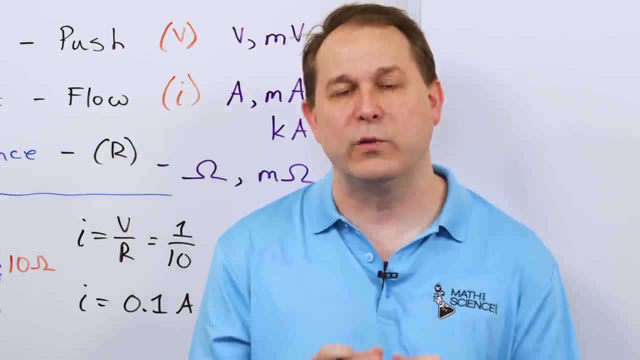 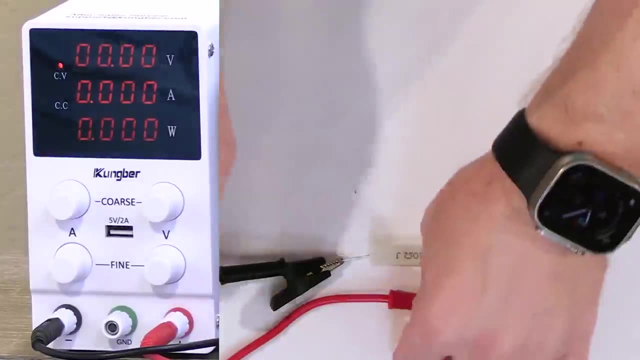 the more power that it can take, the more heat it can dissipate without burning itself out. All right, So what we're going to do is connect one side. These are coming straight out of my over here, which I can control very carefully. In a minute we'll be using batteries. 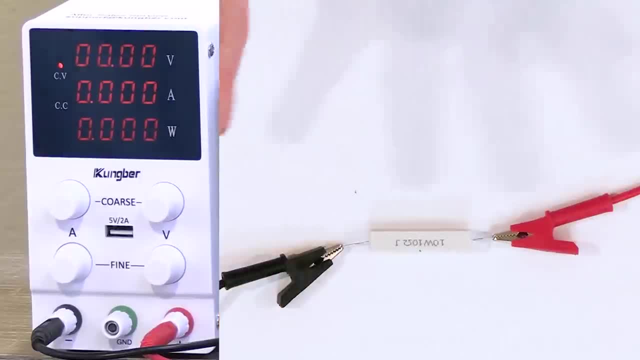 but right now I want to use my digital source here, And so all we have is literally a single circuit element, a single resistor coming straight connected to our voltage source. Now I want to dial this thing up so that it goes up to one volt, So I will increase the current. 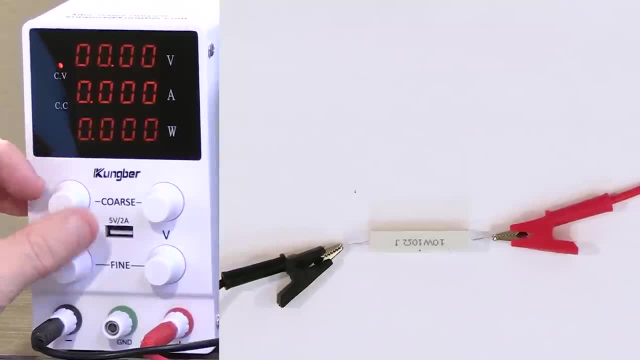 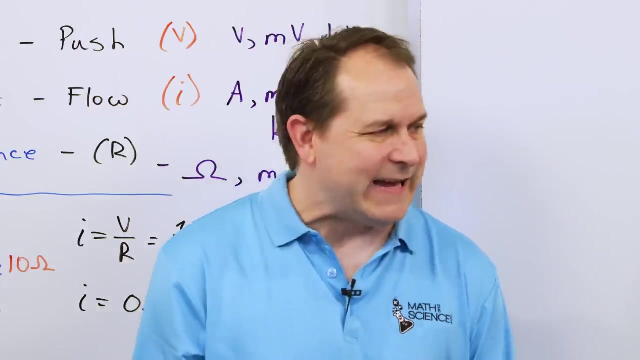 the voltage from my source here. Whoops, I'm turning the wrong knob. I will increase my voltage source and try to get it. I'm going to use the fine knob to get it as close as I can to one volt. Right now it's 1.01 volt. There's 1.00 volts, So we said when there was one volt. 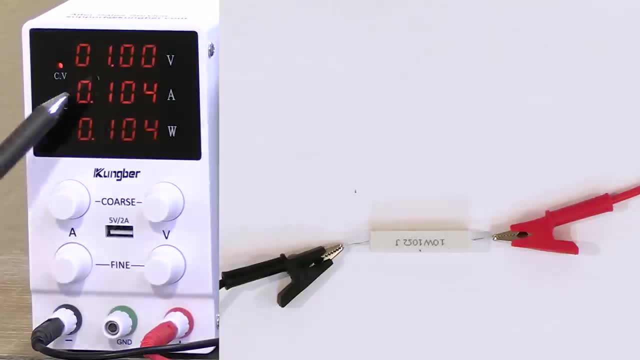 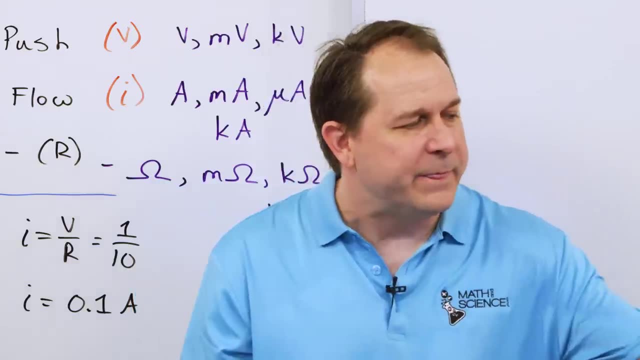 across a 10 ohm resistor, we should get 0.1 amps And notice that we have 0.104 amps. So this is what I'm saying. It's not exactly 0.1 amps, but that's just because there's a little play in the knob. 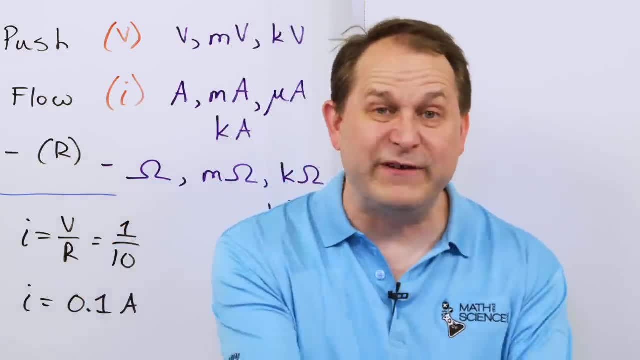 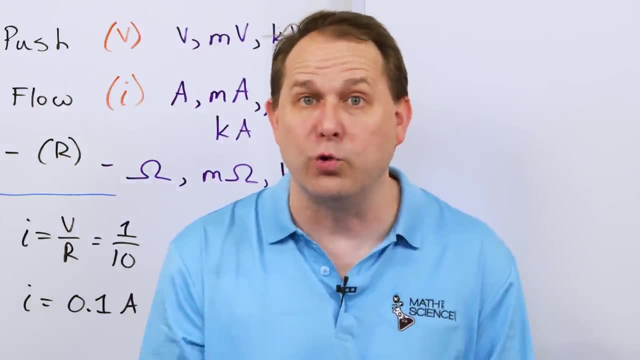 here. There's a little bit of inaccuracy in the display, There's a little bit of resistance in the wires connecting everything together And also this resistor is not exactly 0.1 volts. It's a 0.810 ohm resistor. but notice that we get exactly what we predict: 0.1 amps. 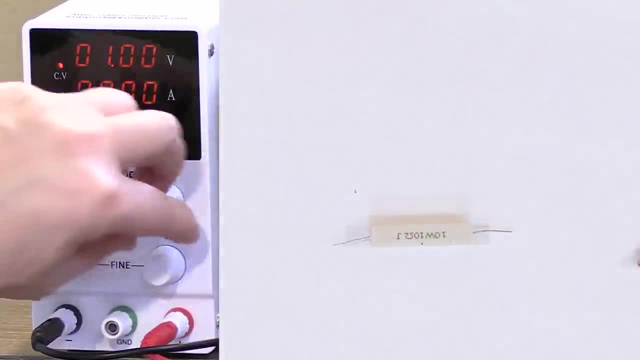 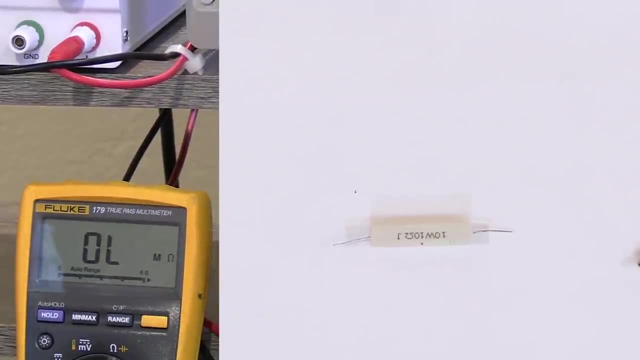 Let's, just for giggles, disconnect it from here. I'll turn my voltage down and I'm going to turn my meter on over here. This is a. you can measure voltage, you can measure current and so on with this. And just for giggles, let's go ahead and measure the resistance of this resistor here. 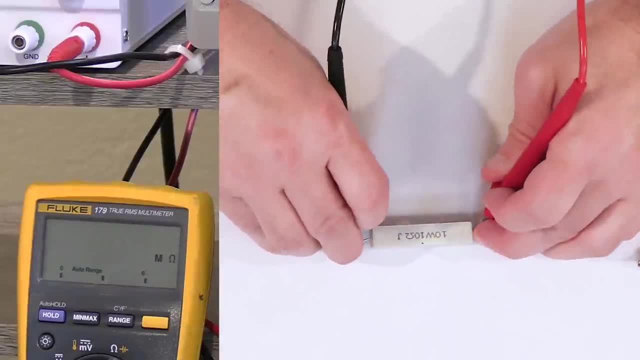 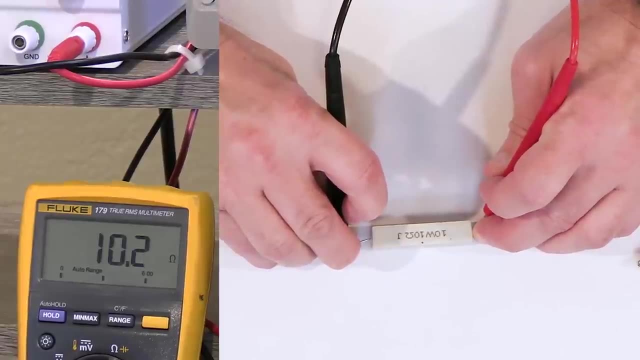 So all I'll do is I'll connect to each side here and we'll measure and see what it says. We'll give a nice good contact pressure and see what it comes up with. And we see right here 10.2 ohms. So it's not exactly 10 ohms. That's one thing I told you. 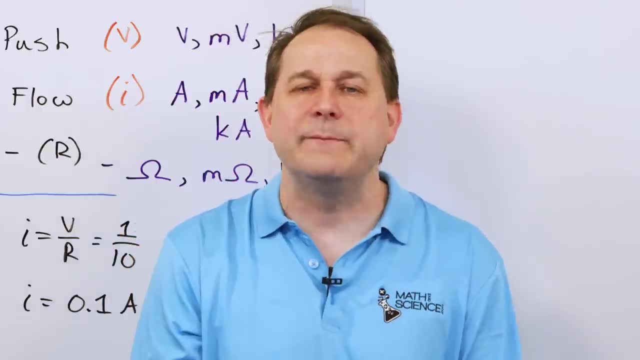 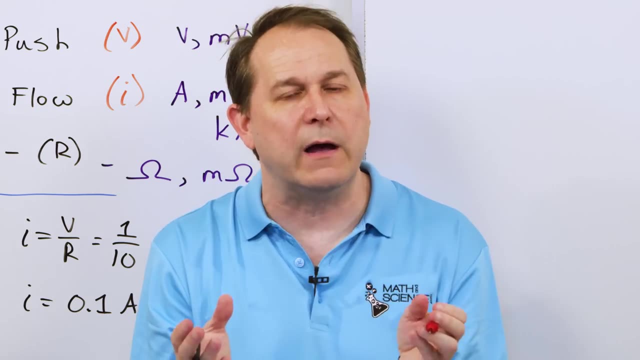 The resistor has a certain tolerance to it. They can't make them infinitely accurate, Okay. And also, when I touch the resistor with these probe tips, that introduces a little contact resistance as well. So in the real world, with circuits, you calculate based on your desired. 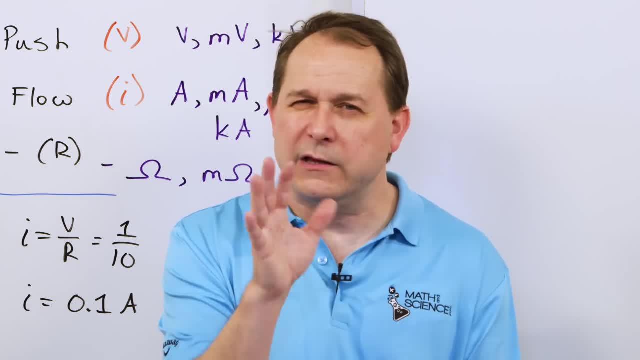 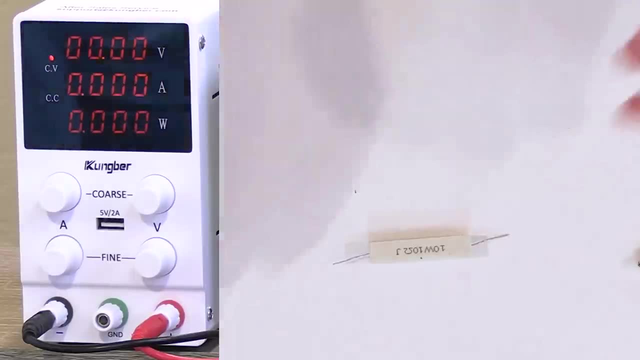 values, but you know, in real life the real values will be a little bit different than what you calculate, just because in the real world it's not perfect. All right, So let's go back And let's reconnect. I got my voltage all the way down, so I'll reconnect my circuit here. 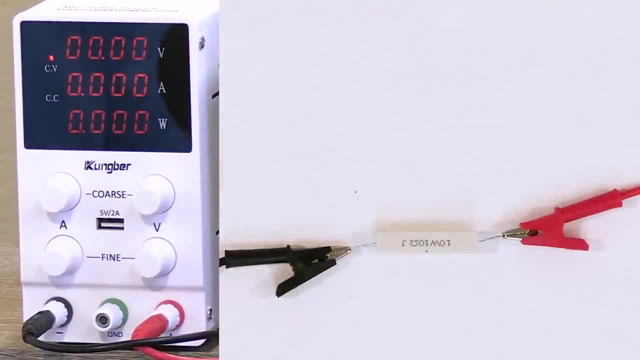 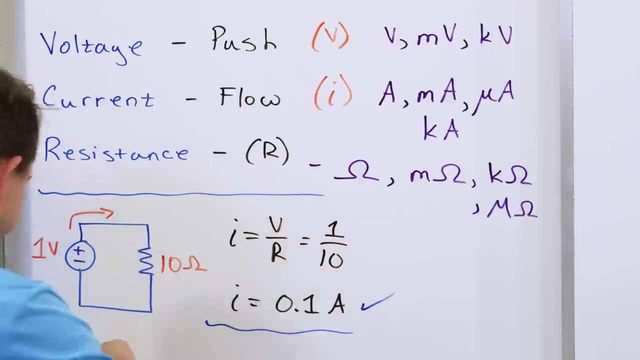 So we verified that when we put one volt across this, we we got the 0.1 amps out. So that's correct. Ohm's law is validated. right Now, what we're going to do is play with this a little bit more, right? So we're going to go up to two volts. So what if I put two volts across this? 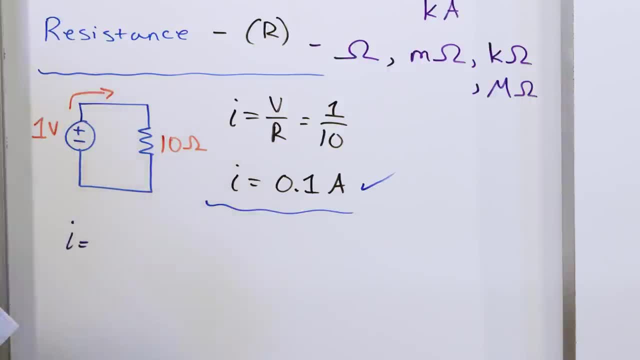 So I changed the one volt to two volts. I can erase this if you want and put a two there, But if I put this and replaced it with two volts, it would be: i is equal to two volts. So then I'd to V over R, but the voltage would not be two volts and the resistance would still be 10 ohms. 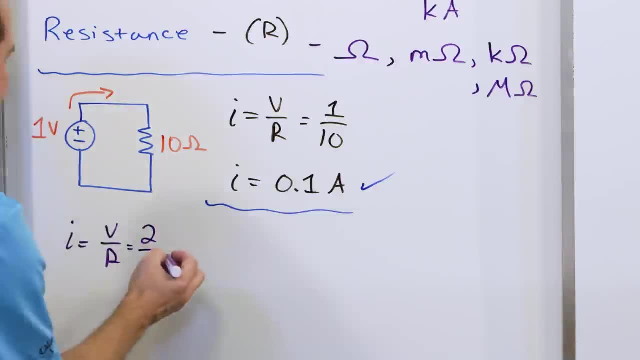 So I'm working in the base units of voltage and amps, And so what I'm going to get is the current. in this case, two over 10 is going to get me 0.2 amps. Now let's go over here and see if that's. 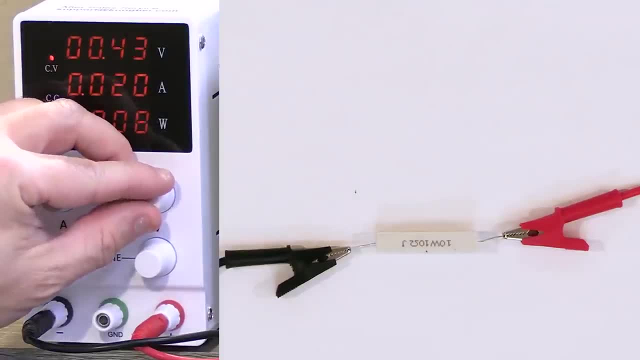 what we get. We haven't changed anything. We're going to now increase this thing to, instead of 0.1 volt, we're going to go up to two volts and I've overshot, So I'm going to go down. It's kind. 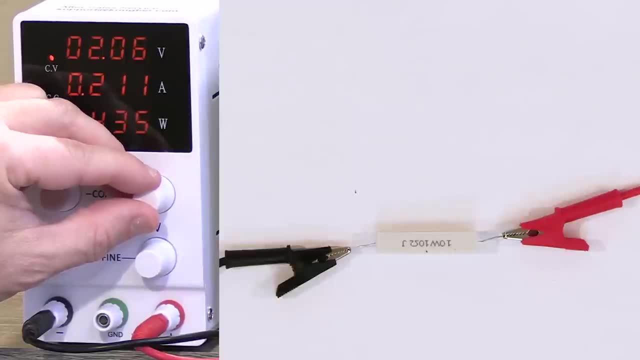 of hard to get it exact, So I'm going to try to go very, very slow, and it looks like I've overshot again. So I'm going to go down and I'm going to use the fine knob to go up to two volts. 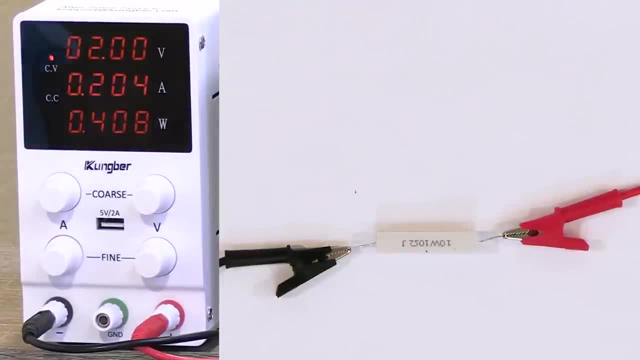 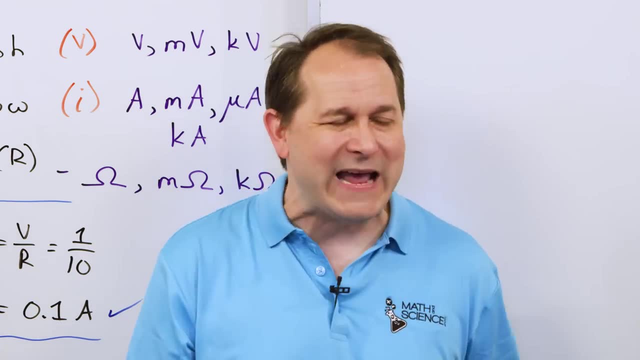 What do I get? 0.204 volts, Again. I mean amps, Again not exact, but it's close enough that we know that what we're predicting with Ohm's law is matching reality. This is a nice device because 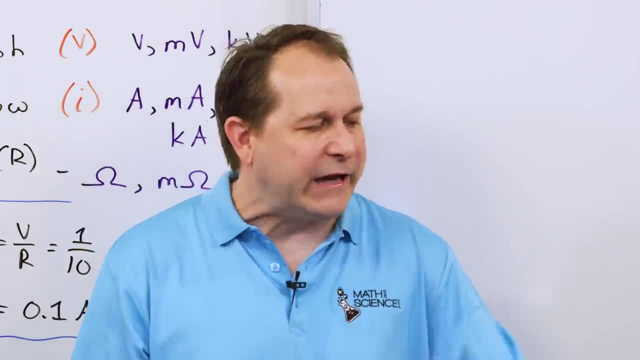 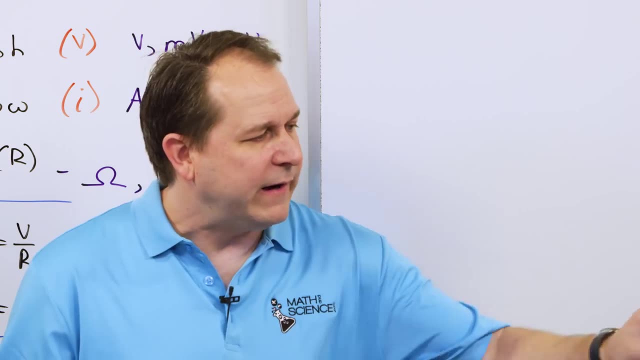 this voltage source also tells me how much current is flowing. I could use this meter to, of course, hook into the circuit and measure the same thing, but it's just too easy to use the source that I have All right, So let me turn it off. I don't want to dissipate any power for 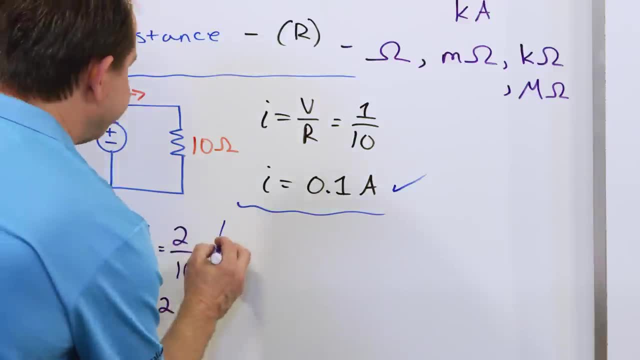 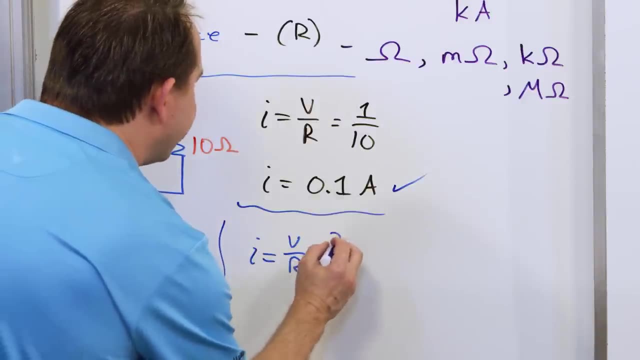 no reason. Let's predict what's going to happen. Let's do a couple more. Let's say it's three volts, I is equal to V over R. Let's say I change this thing to three volts. So three volts and 10. 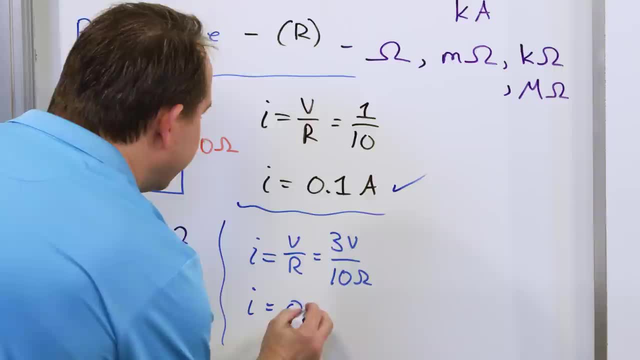 ohms. So three over 10 is 0.3, 0.3 amps, And we're going to check that. We know that this one's correct And I'm going to go ahead and calculate the last one. So I'm going to go ahead and 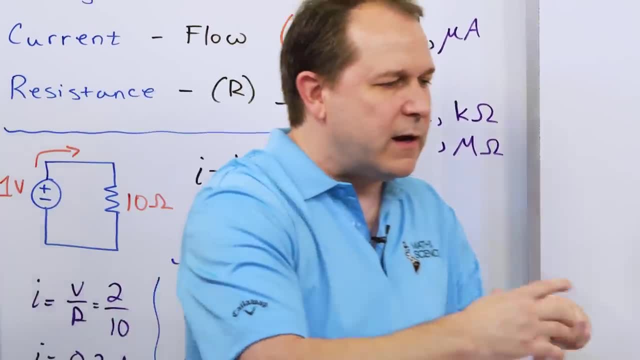 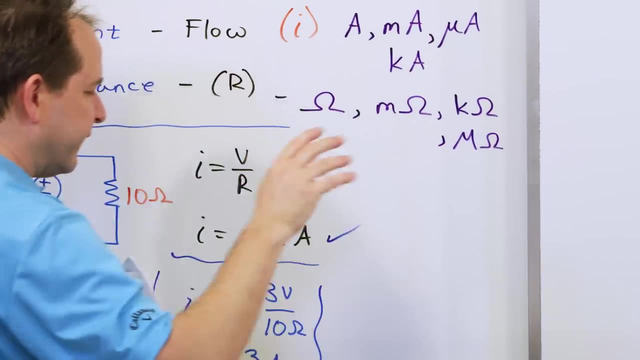 calculate the last one. Again, I'm working my way up to six volts because, remember, I have this six volt battery. I'm going to start playing around with the six volt battery soon, So I want to show you what happens when we get up to six volts. So when I use the battery, we'll see the 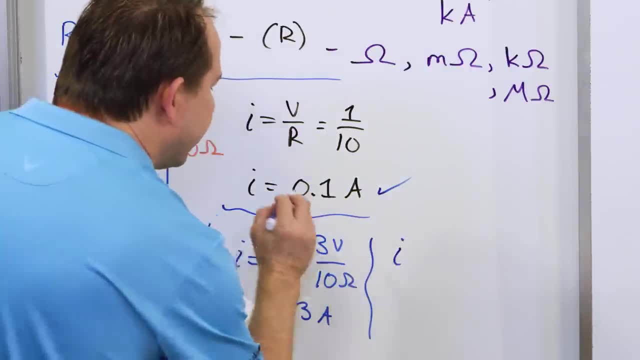 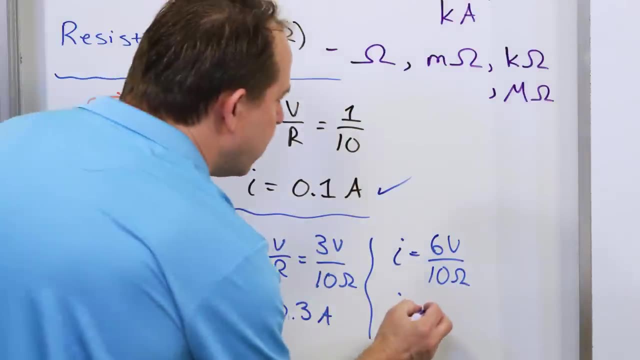 difference. right, If there is a difference, So let's change it from three volts to six volts and 10 ohms, And so when you get six over 10, 0.6 amps, So we have two of them to check. 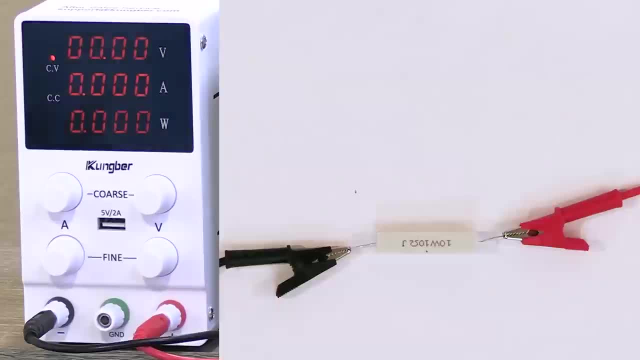 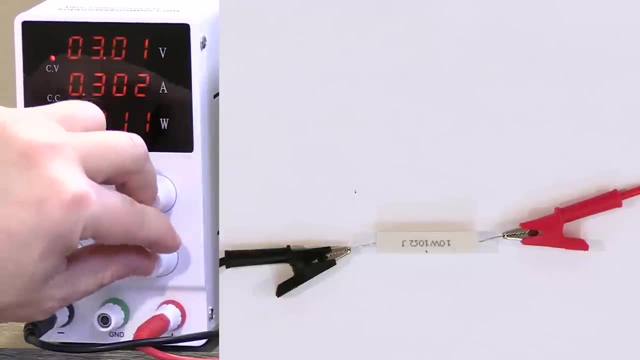 three volts and six volts And let's just see what we get. So we'll go up to three volts and I've overshot. So I'll go down very, very close and I'll go three. So at three volts I get 0.302 amps. So according to Ohm's law, that's what I predicted. 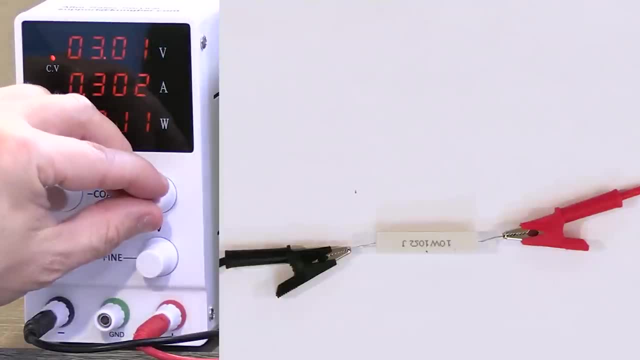 that that's correct. And then I'm going to go up to six volts. There's five volts and there's 6.06.. So I'm going to go down a little bit right here with the fine knob. I'm going to go down to six. 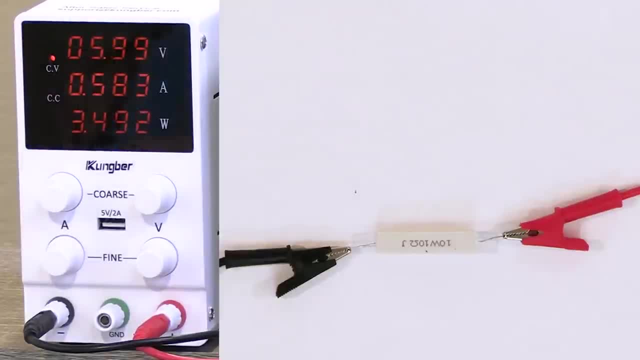 volts. What do I get? 0.583, right, Which is 0.583.. So I'm going to go down a little bit right here, very, very close. If you round it up to this now, you have to ask yourself: oh, why is it different? 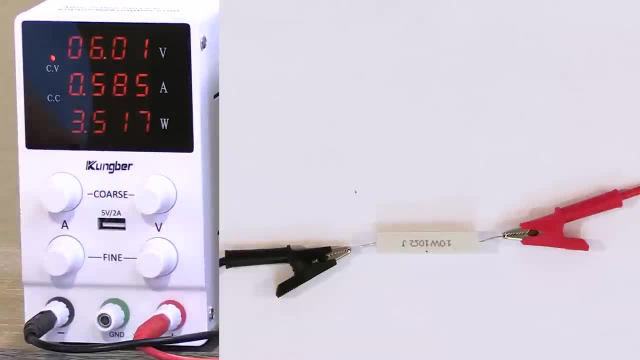 What's wrong with that? What am I doing wrong? Well, there are there are. this wire is not a perfect resistor, right? So this is the difference between theory and reality. It's not a perfect conductor. This wire, even though it's made of copper, actually has a very small resistance. 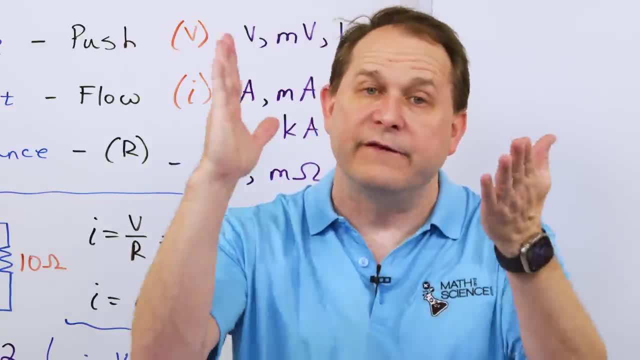 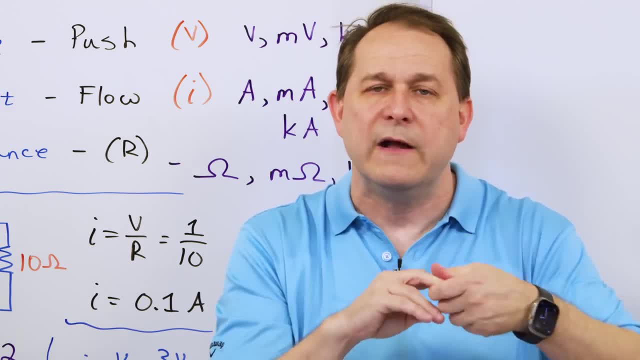 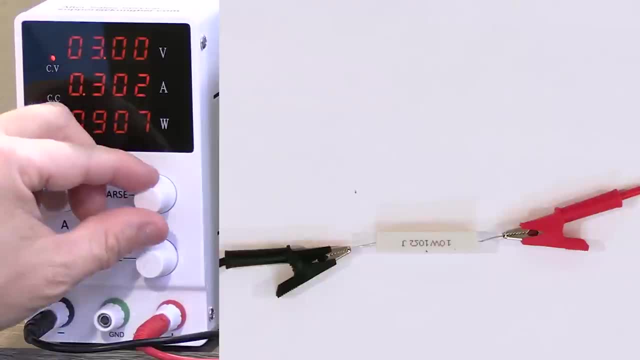 volts. it was pretty close to act. It was very close to accurate 0.3 amps. When I get to four volts, let's go down to four volts. We expect 0.4.. Let me go up just a little bit. We expect 0.4. 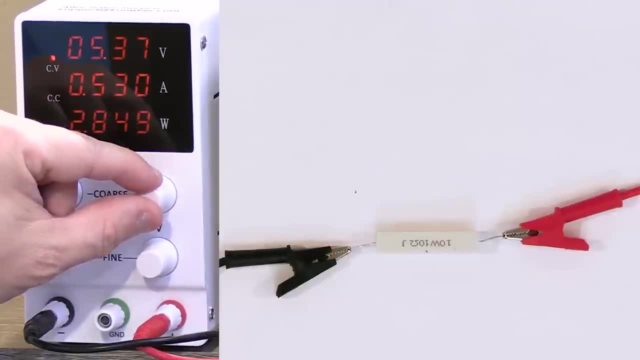 amps. Notice, it's very close, but not quite. And then when I get to five volts it's a little bit different, right, You can see the difference there, And when I get it to six volts it starts to be amplified enough. where it's different here, Okay, 0.584 amps So, but we still know that as 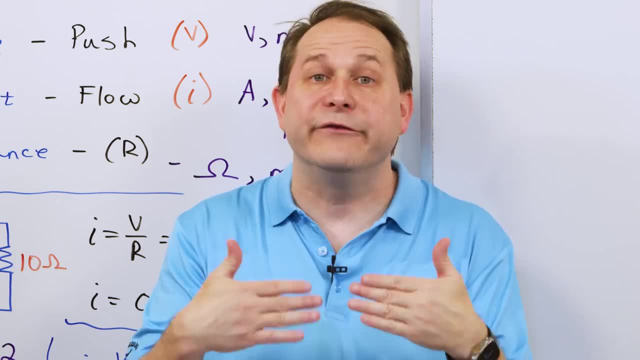 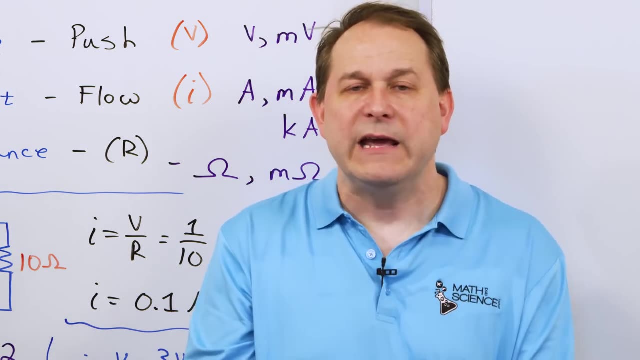 we increase the voltage, the electric current in the circuit seems to go up by a, not by an equal amount, but by a proportional amount. The reason I'm doing this is to show you that when we have linear components in the circuit- and what I mean by linear components basically- 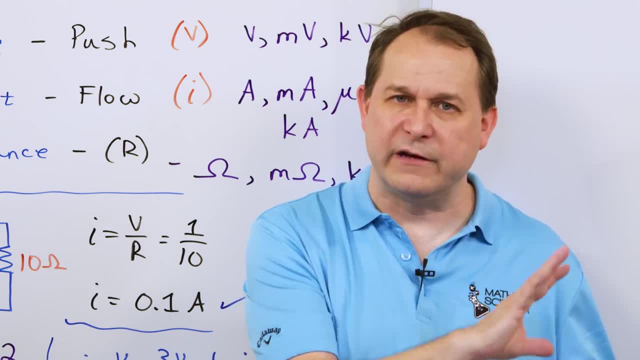 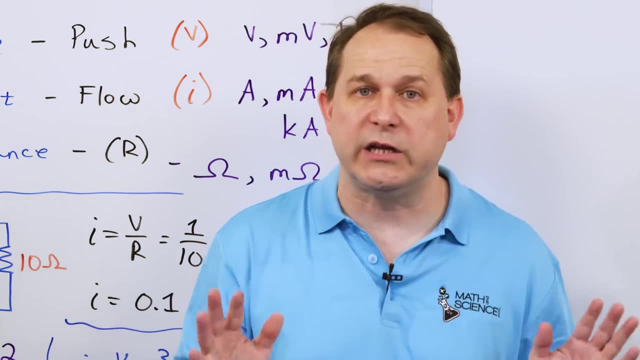 is in this case resistors. We'll talk about capacitors and inductors later. but we have nonlinear components. We're going to talk about later diodes and transistors that amplify things. Those are nonlinear components. The current and the voltage relationship in a transistor is not 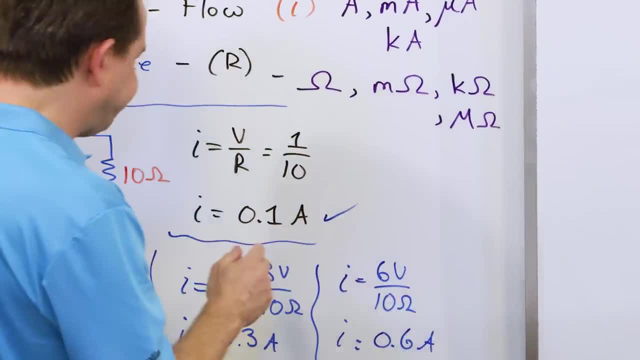 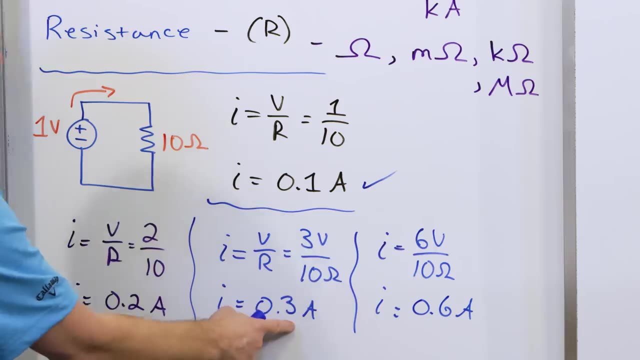 linear like this In this case, when I started over here, when I started at one volt, I got 0.1 amps, two volts, 0.2 amps, three volts, 0.3 amps, six volts, 0.6 amps, even though it wasn't exactly. 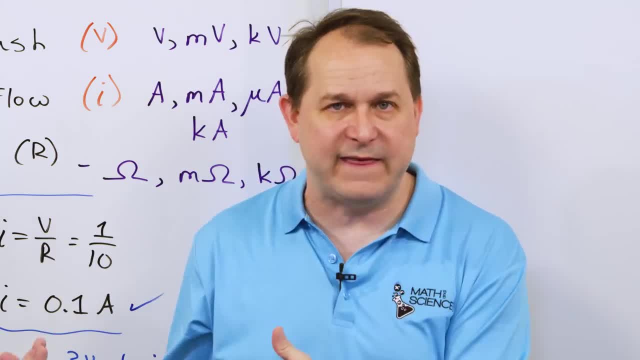 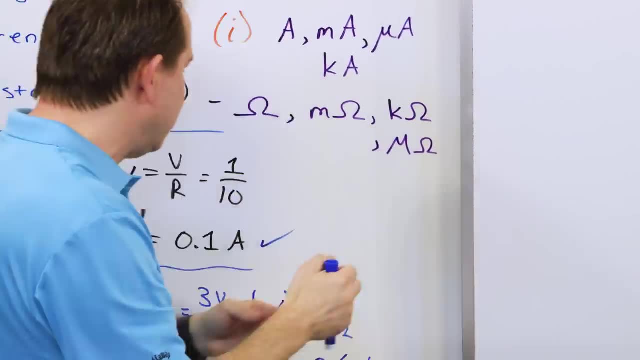 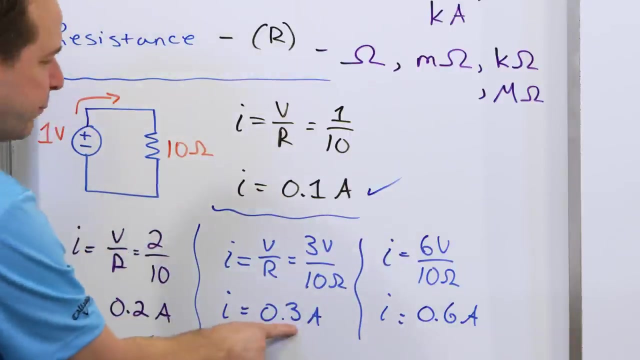 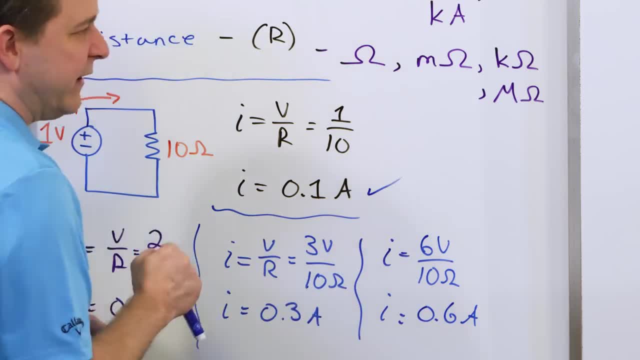 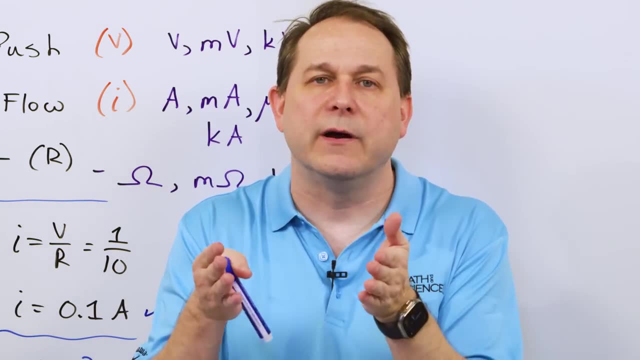 here to here. 0.3 amps actually went three volts and we increased 0.3 amps. So they they increase with lockstep from one another. The current and the voltage through a linear element like this increases linearly. As you increase the voltage, the current goes up by a, proportionally by a. 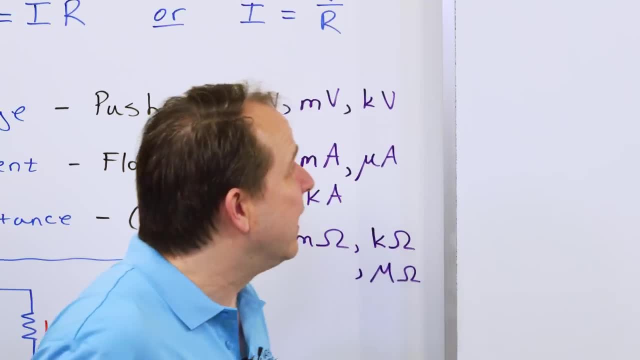 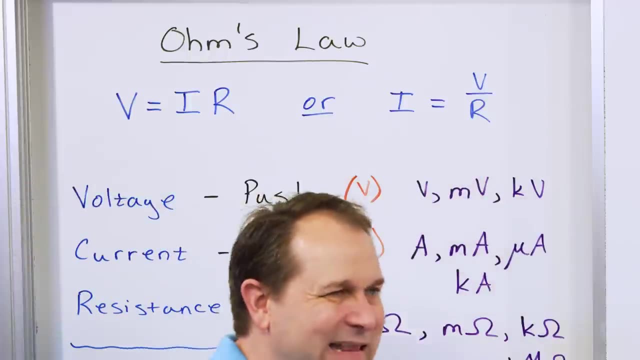 proportional amount right. And the reason it's like that is because if you go back and look at Ohm's law, I is equal to V over R. This relationship is a linear relationship. What do I mean by a linear relationship? Remember back to algebra class right In high school. you spent a lot of 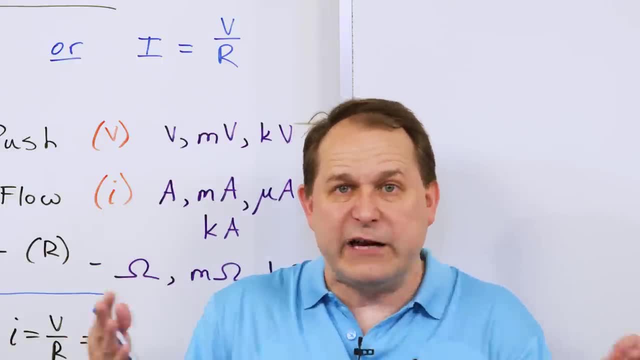 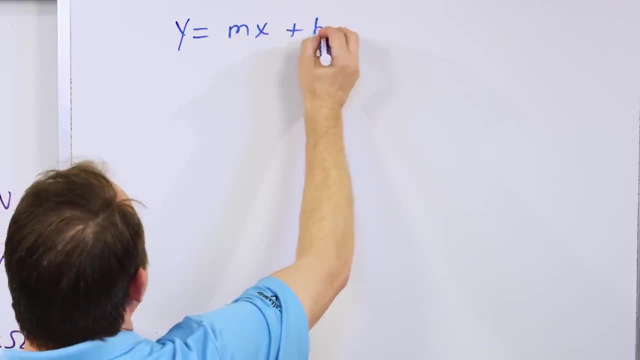 time. everyone spends a lot of time graphing lines. We say: this is an equation of a line. What does the equation of a line look like? right Y equals M times 0.2 amps. Right Right X plus B. And you learn in algebra class that this is the thing called the Y intercept And 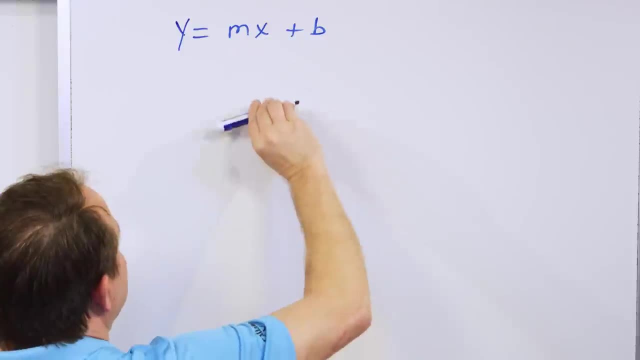 this is the thing called the slope, And this slope tells you how steep the graph is. But basically, if you can put any equation into this form, you know it's going to form a straight line. We call that a linear relationship. But what is Ohm's law? I equals V over R, If I say that I. 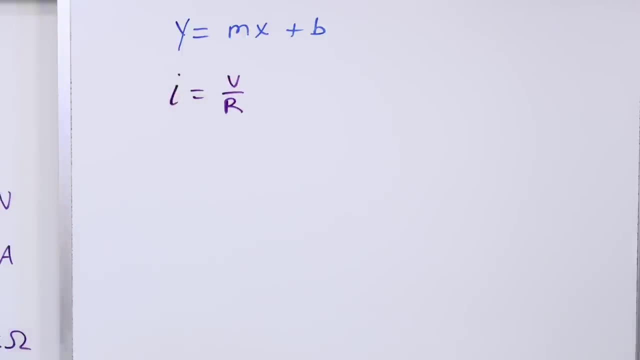 is equal to V over R. you say, well, wait a minute, that doesn't look like that. But then you say, okay, notice that the resistor was constant. That never changed. All I changed was a voltage and I measured the current. So I can write this as: instead of like this, I can write this as 1 over R. 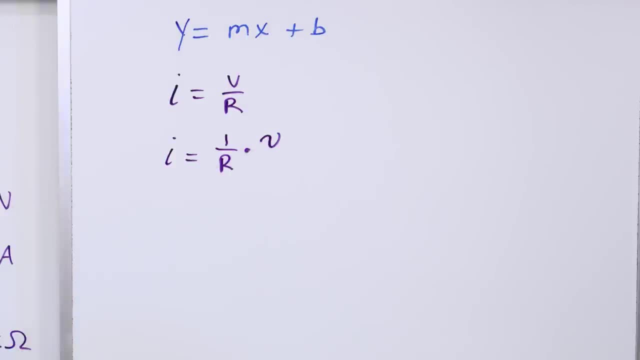 multiplied by V. Think about how we multiply fractions. If I make this V over 1, then you have V multiplied. you get a V on the top and an R on the bottom. So I don't need to write it like that, I can just leave it like this. But then what happens if I say, okay, I'll just change the Y? 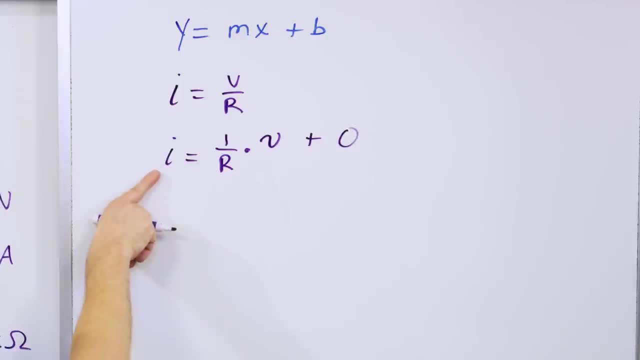 intercept to be 0. Then this equation, the equation for the current through a resistor, is a line. And it's a line because we can then say that the slope of this line is just 1 over the resistance, If you think of it. 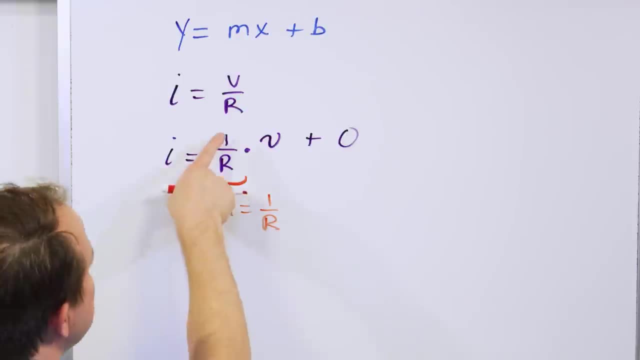 that way that this is just a constant right, Because the resistor was 10 Ohms, So this is just a constant number: 1 over 10, right, And this is the slope of the line. Then it's: I equals MX plus. 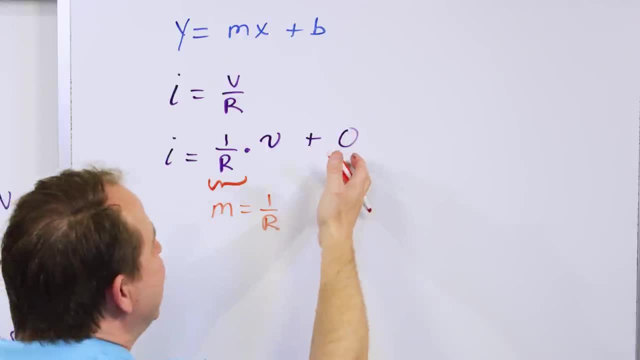 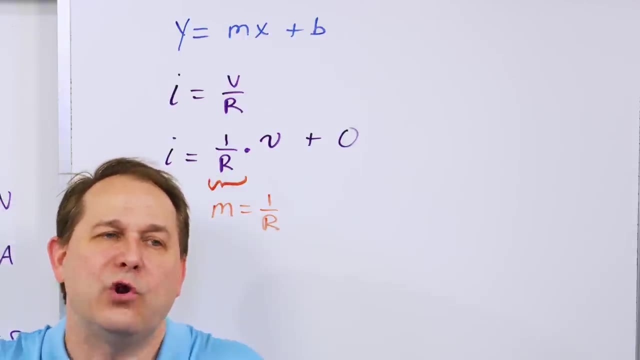 B, where the Y intercept is 0. And the reason it's 0 is because when you drive it with 0 voltage you get 0 current. So of course the line has to go through the origin, because if you don't put, 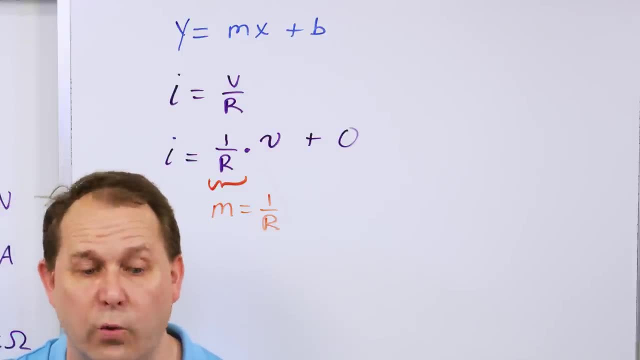 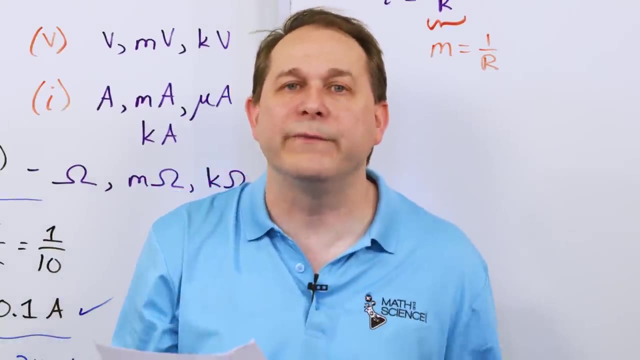 any voltage in, you don't get anything out. That just means the line goes through the origin. So I don't want to graph it and draw, but you get the idea. I just wanted to show you that it behaves linearly, because Ohm's law is the equation of a line. That's all I wanted to get across to you. 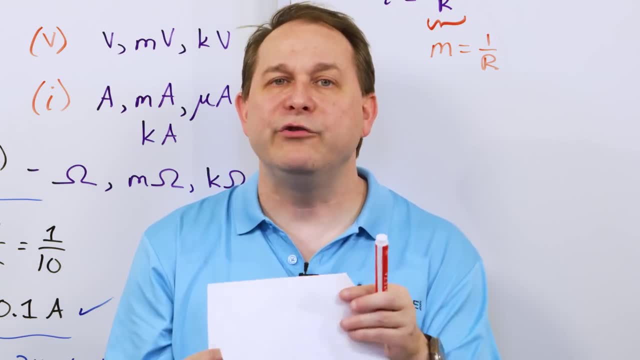 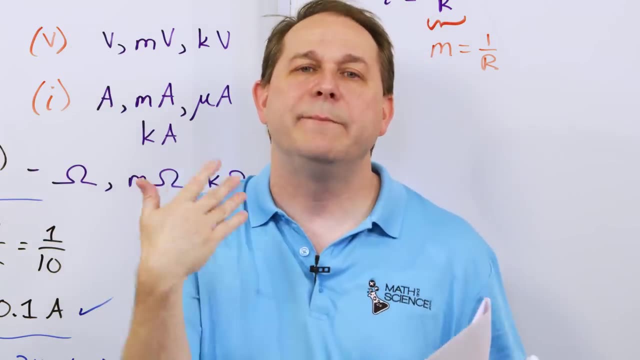 so that you understand it And just as a preview, when we get to transistors and diodes later, the current voltage relationship will not be a line. It will be a nonlinear type of deal because of the way those devices are constructed And because of that you can. you can amplify. 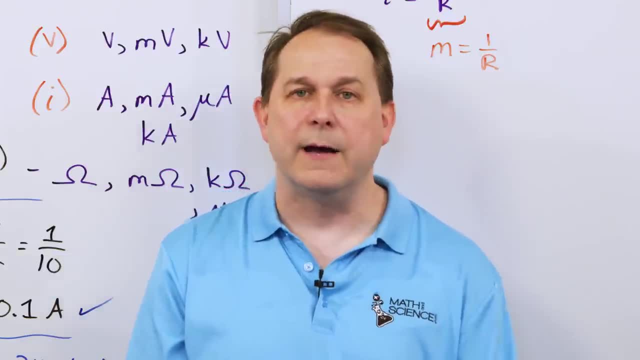 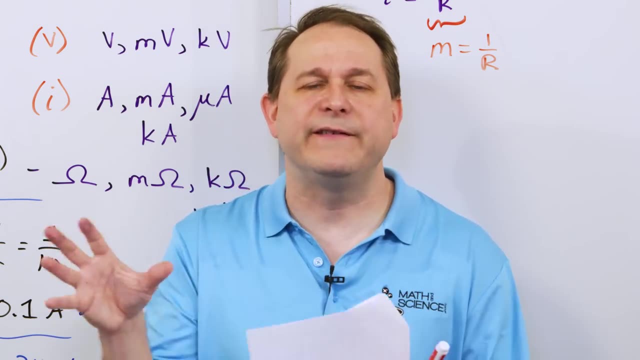 things. That's one of the main uses for transistors. We'll get to that much, much later. All right, Now we need to transition ourselves to talking about the batteries. Why do we have all these different size batteries If they're all about the similar voltage range? All right Now. 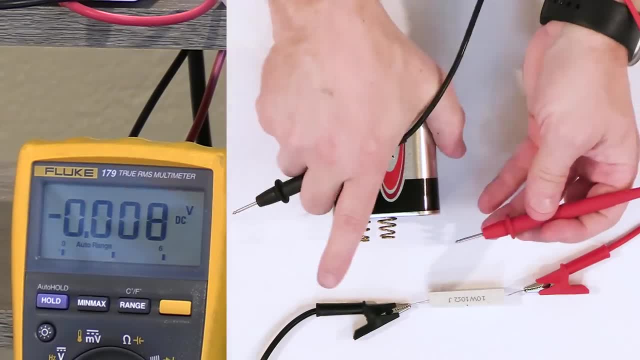 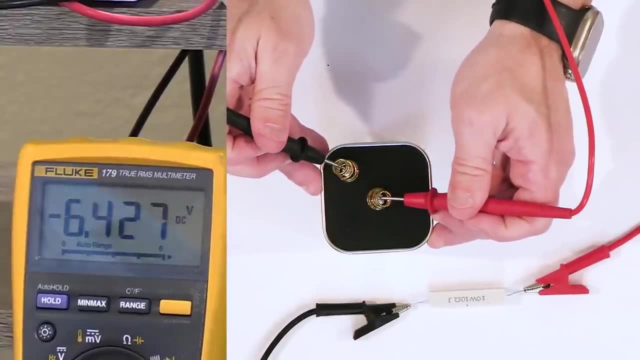 I told you to take my word for it earlier. Now I want to actually show you. this is a six volt battery. It's printed right on the side here And if I connect my volt meter across the two terminals and measure the voltage, I get a negative because I've got them flipped around. 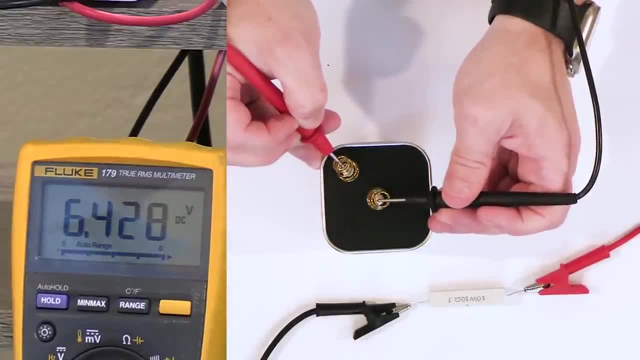 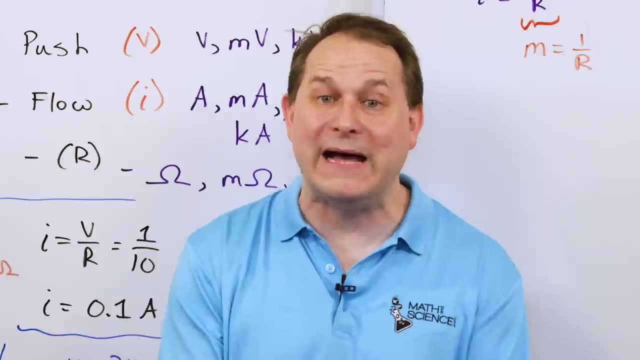 If you look over there, it's 6.427 volts right Now. this is a six volt battery. This is another theory versus reality thing. It's printed on here that this is a six volt battery, but when it's fully charged, like 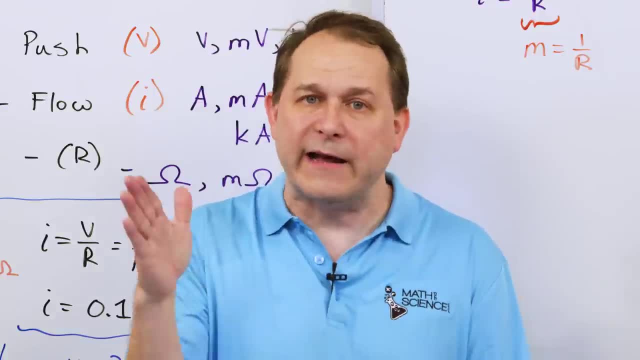 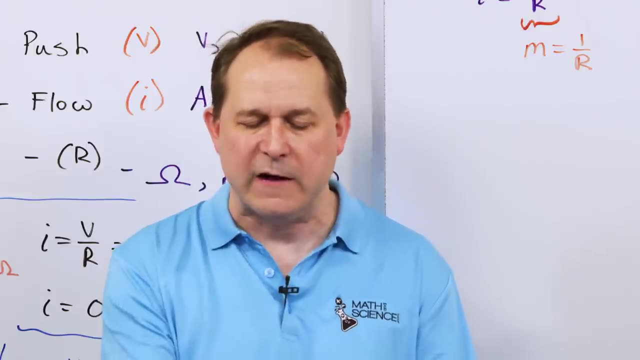 this it's a little bit more than six volts. as it is depleted, That voltage is going to come down and down and down, But usually these things are about a little bit more than their stated voltage when they're fresh out of the box like this. So this is what we would call a six volt battery. 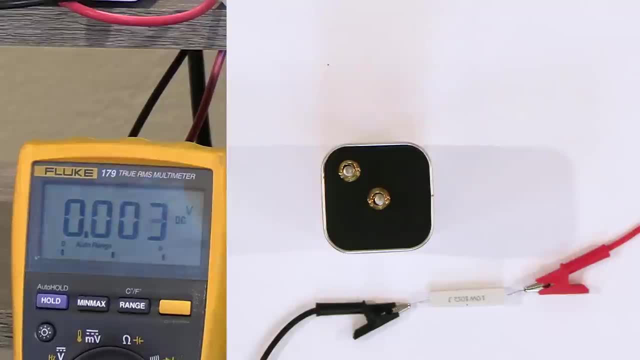 even though it's a little bit more than that. Now let's go down stream a little bit. We'll put the six volt battery off to the side. And then we're going to go down stream a little bit. We'll put the six volt battery off to the side, and I want to talk to you about these things. These are called. 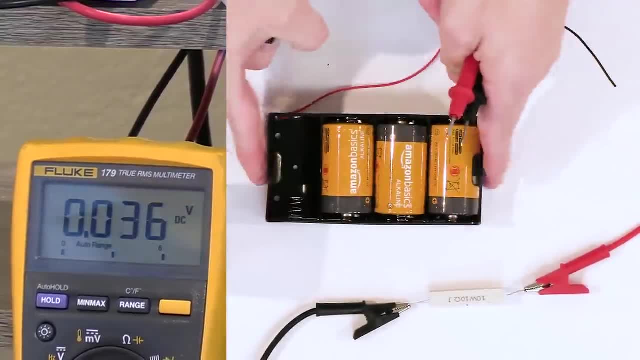 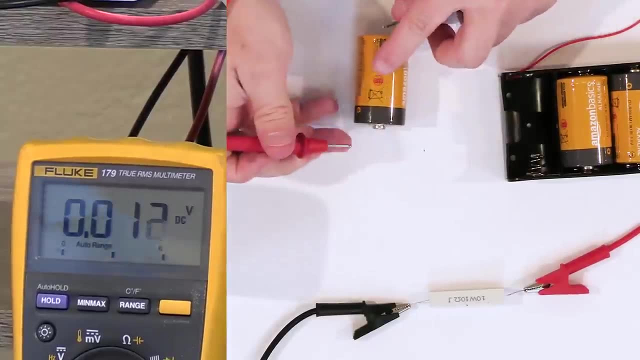 D size batteries or D cell batteries. I'm going to take one of them out. right? If you read the fine print on this thing, it says that it's one and a half volts. Let's see. So what I will do is I will. 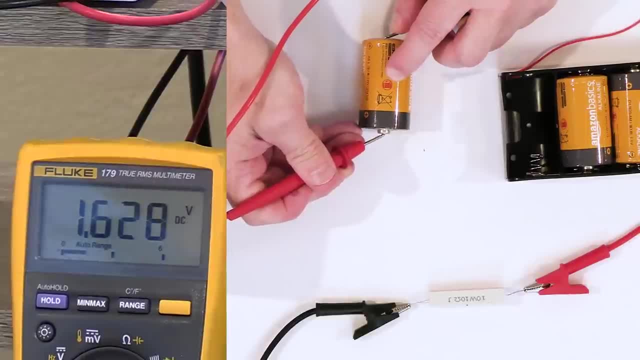 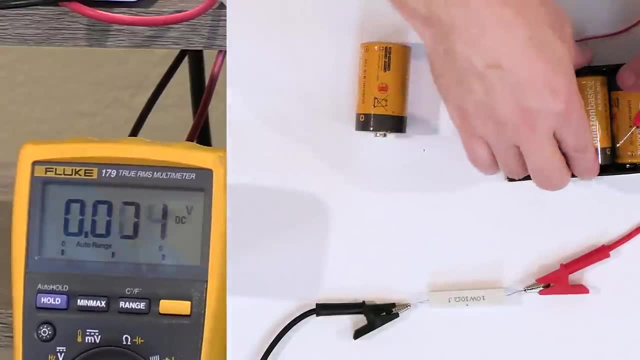 connect my meter across the top like this And again notice it's not 1.5 volts, That's what's printed. It's a little bit more than that because it's fully charged. Now if you take two of these things and you connect them, you've got to again think about voltage as a mountain. This, literally. 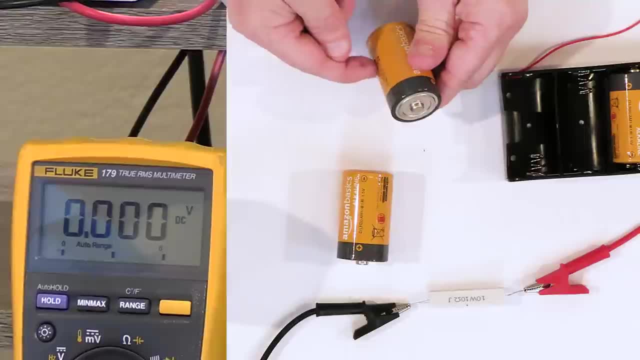 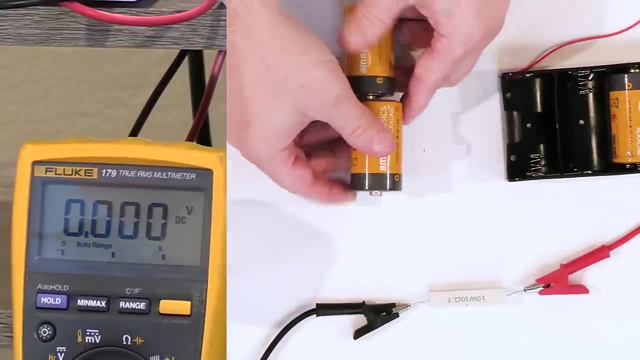 represents like the top of a mountain right And you're at the high part of the mountain when you're talking about the top terminal, compared to the bottom, If you stick two of them together, it's like stacking two mountains on top of each other. So what do you think the voltage should be? 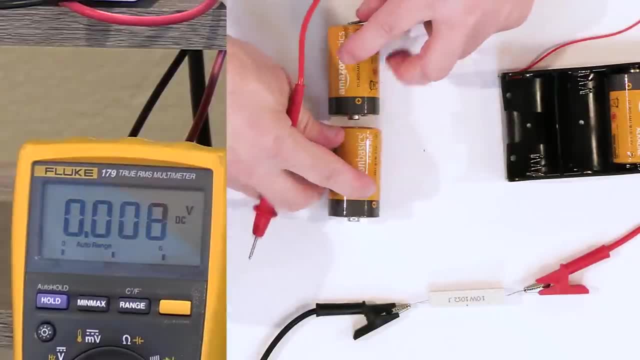 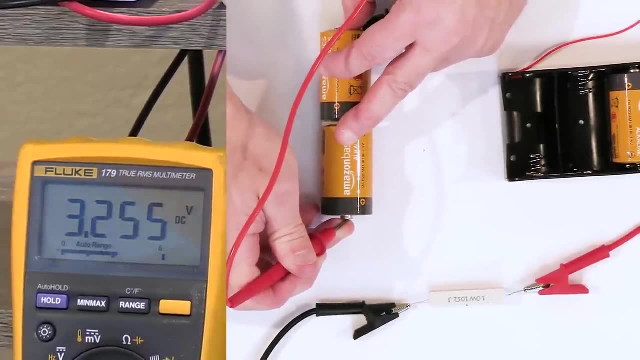 if I've got them stacked like this, Well, it should be adding the two together, because it's literally like stacking two mountains one on top of another, And if I look over there, the 1.6 plus the 1.6 is 3.2.. So that's exactly what we get. So when you see these little 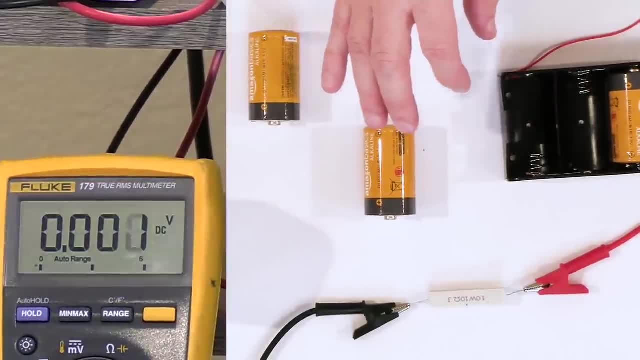 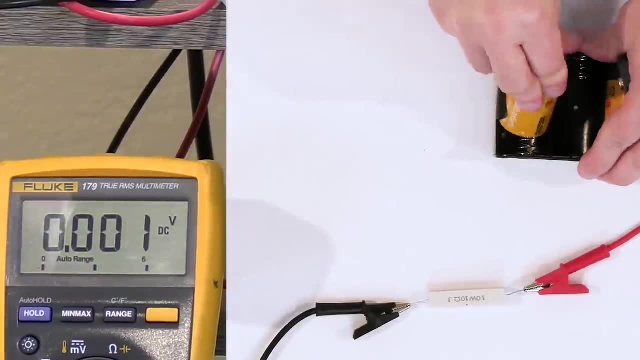 devices like this, these little battery holders like this. all that's going on is it's alternating the direction, But all that's happening is you're putting them end to end to end to end like this. So if I put the flat part on the spring right here and then the flat part on the spring right here, 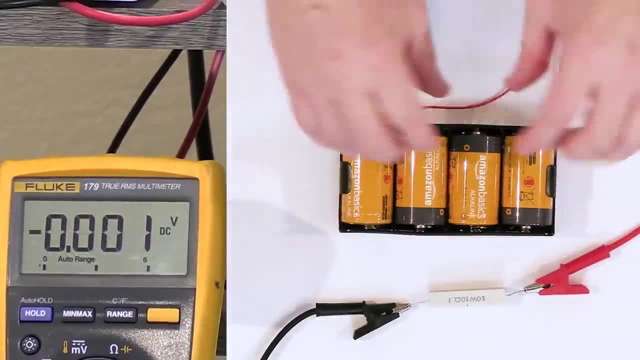 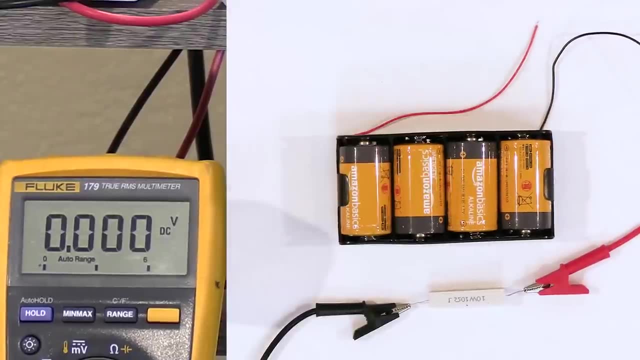 like this. and then these are oriented the same way. all I've done is, instead of stretching them out in a line, I've folded them up, but they're still end to end like this. So if I take a look at this, then I know it's about one and a half times four. So it's going to be about one and a. 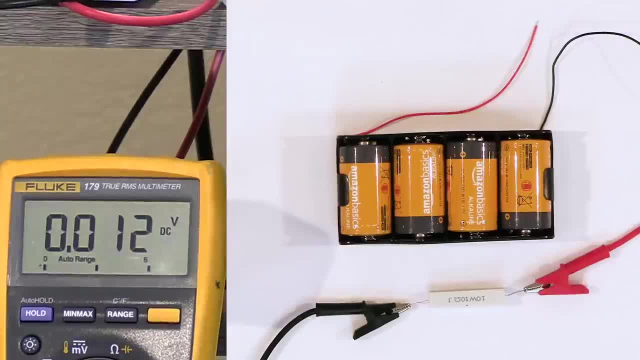 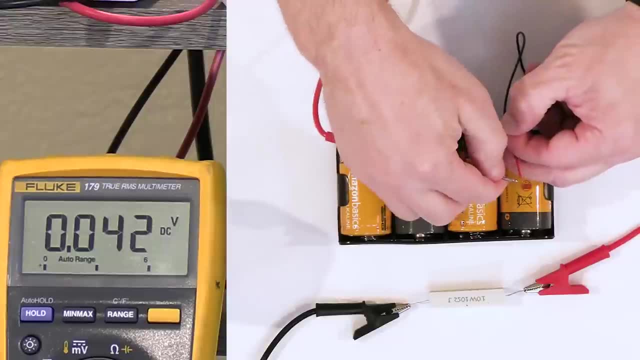 half times four, So it should be about six volts. Let's see what the actual voltage is. So I'm going to hold this side of the wire right here And then the red side. I'm going to hold with this one right here And we'll read the meter over there. 6.5 volts is what I get here For reference. 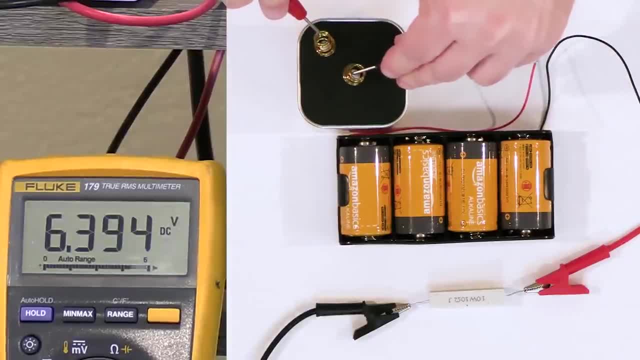 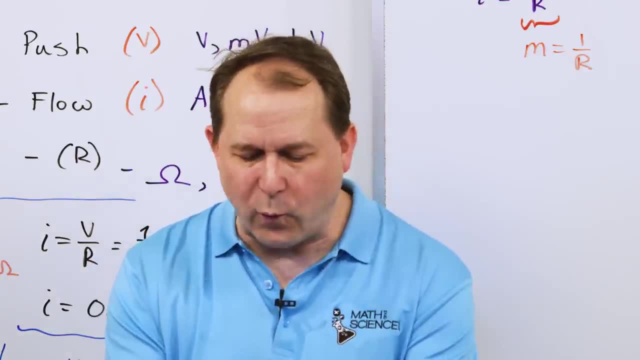 remember that this one was about the same 6.4.. So the question I have for you and that what we're going to answer is: if this is about six volts- and this is about six volts- why do we have these different size batteries, right? 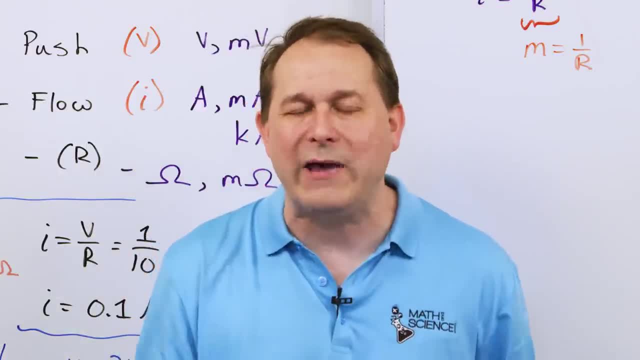 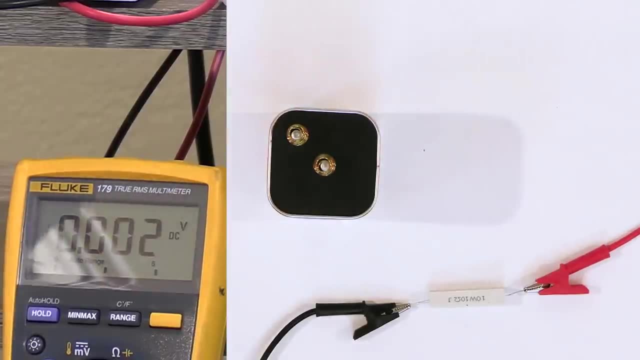 So, to go through the different sizes I have, I'm going to give you the punchline and tell you why we have them, And then we're going to do a little experiment to show you why what I'm telling you is correct. right, So let's put these away. These are the D cell batteries. Now these are the C cell. 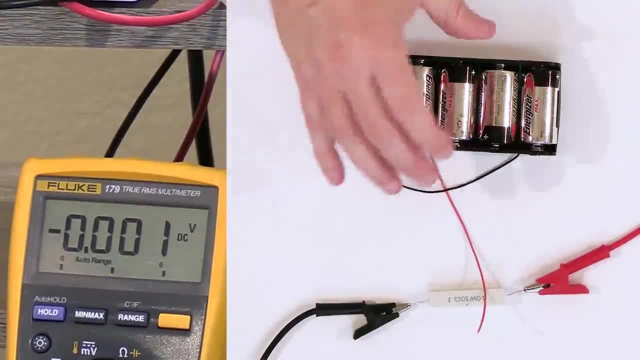 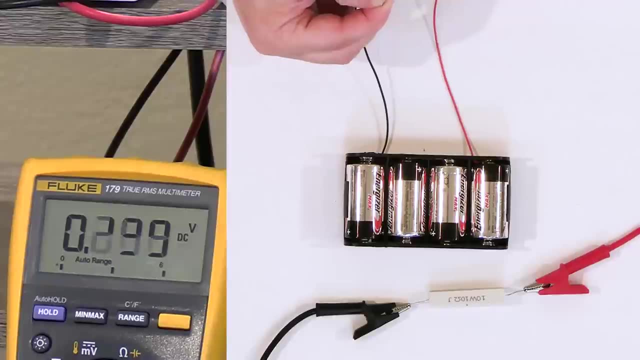 batteries. If you read the package on these very carefully, this package will also say that each of these batteries is about one and a half volts. So once they're end to end like this same kind of deal, I'm going to hold it like this Again: you're going to get just a little bit over six volts. 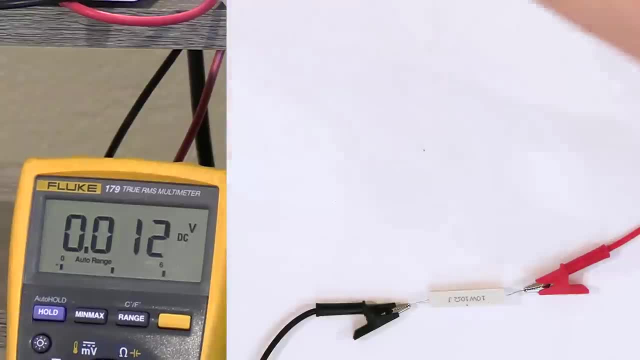 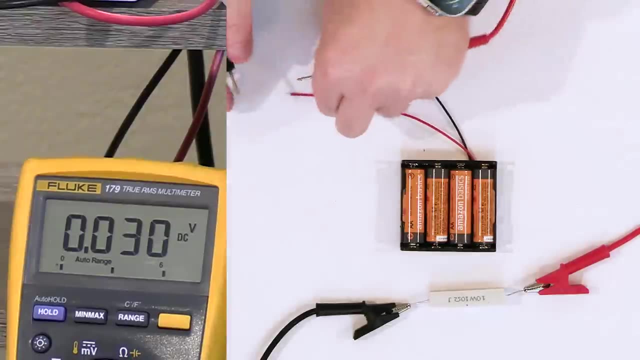 Notice they're all coming out to about 6.4 volts once you stack them together. These are called AA batteries. If you read the package, each one is one and a half volts. What do you think we're going to get if we stack them together, end to end, like this, and measure the voltage That one's a. 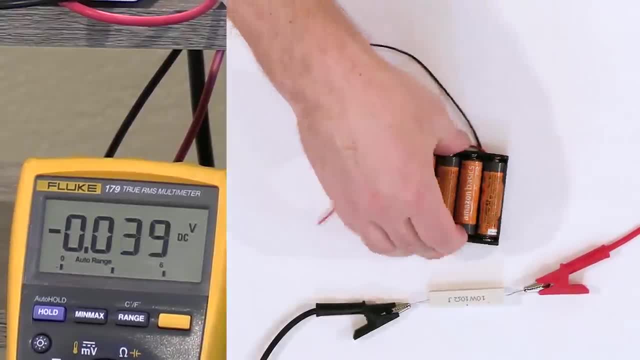 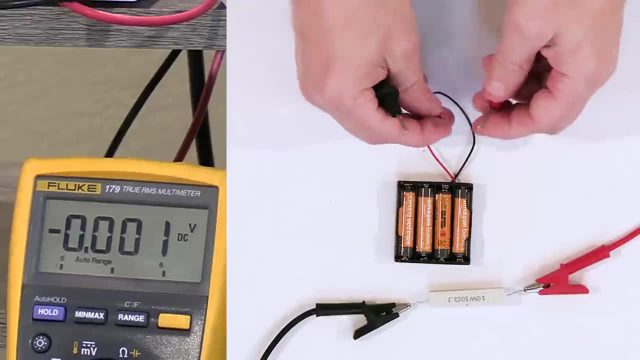 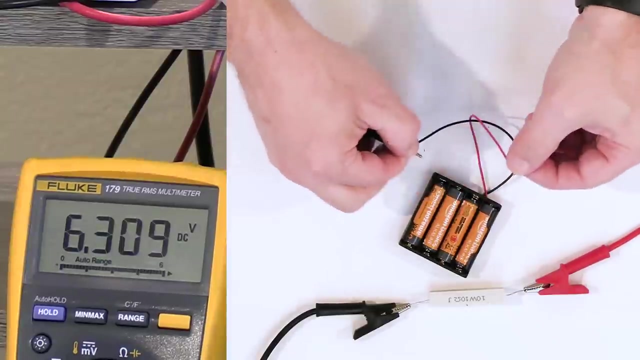 little bit higher, 6.5 volts, but still in the same range, right. This one over here is even smaller. It's called a triple A battery And the triple A battery, if we do it correctly, should measure the exact same thing. So we're going to this wire's flopping around over here. We got them. 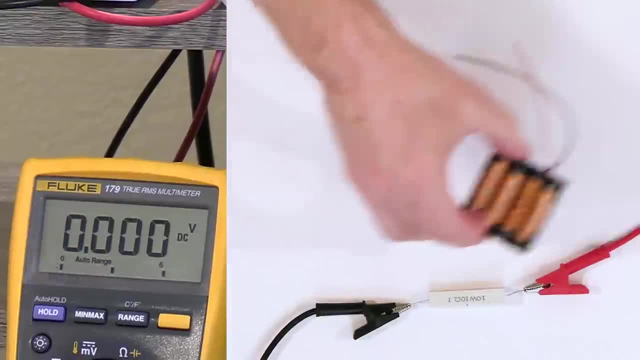 end to end over there a little bit lower, 6.3 volts, but you get the idea: same range. And then, finally, these little batteries. let me get them out here and put them out in front here. These little batteries are used in very small devices, right, Calculators and things like this. Each one. 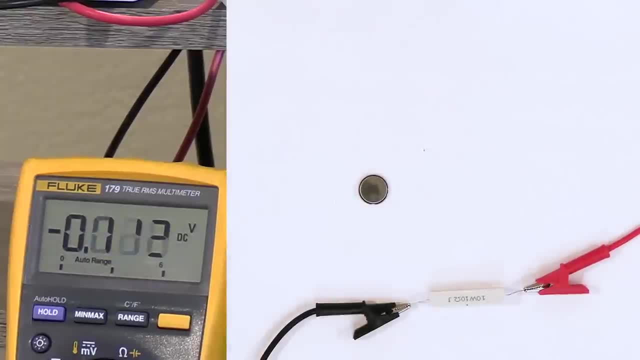 of these is not one and a half volts. Each one is three volts. So what I'll do is I'll just put one side on one and the other side here and we'll see it's just a little bit over three volts. So if we 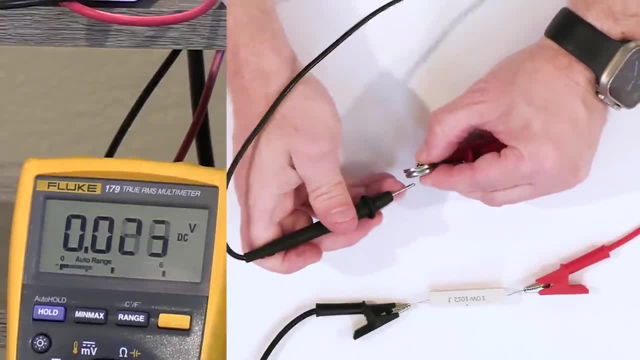 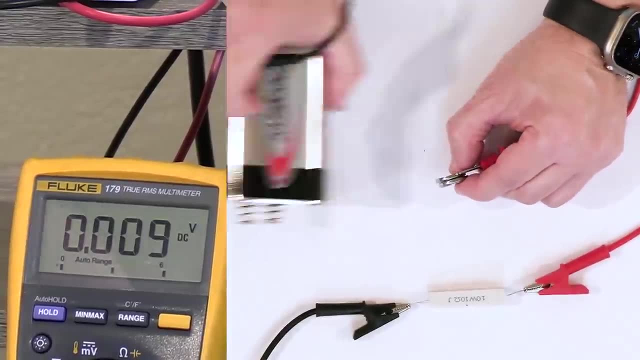 stack two of them end to end, just like this. we're stacking the mountains together And what did we get? Just a little bit over six volts. So these two batteries stacked together is six volts. This gigantic battery here is also six volts. Why in the heck do we have all of these different? 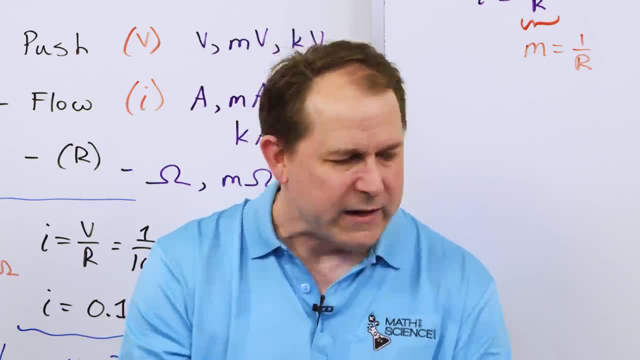 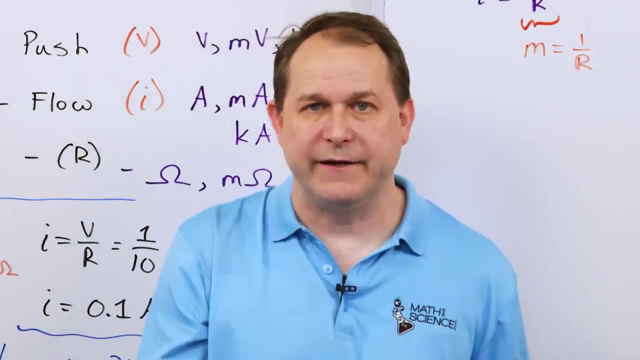 sizes when the voltage is the same. What I'm going to do is tell you the punchline, all right, But then I have to prove to you that the punchline is correct, and we're going to prove it by building stuff. So let me tell you the punchline. We learned that we have Ohm's law, which is the: 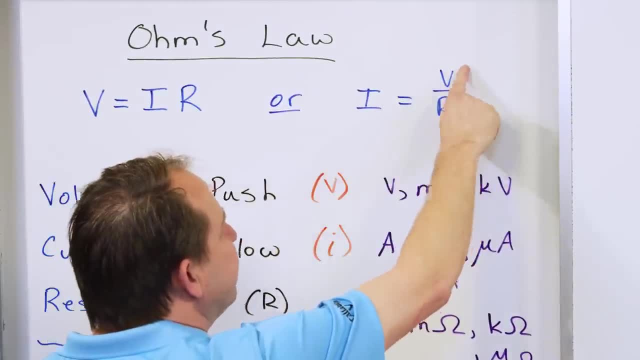 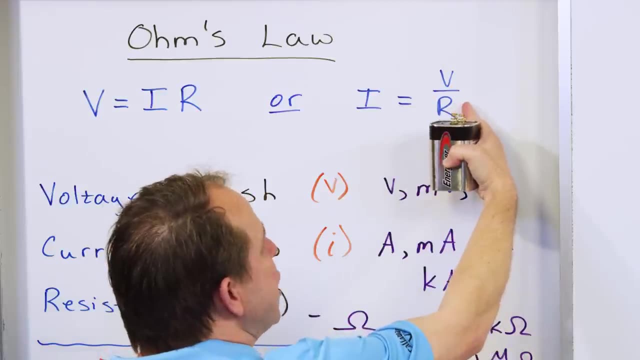 Ohm's law that tells you how much current you will get when you put the voltage in and you get the resistance. So you think that if you put six volts into here divided by whatever the resistance is, let's say it's a 10 Ohm resistor. We already did that calculation: Six divided by 10,. 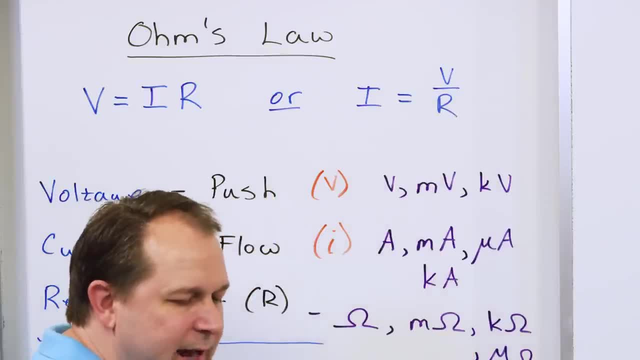 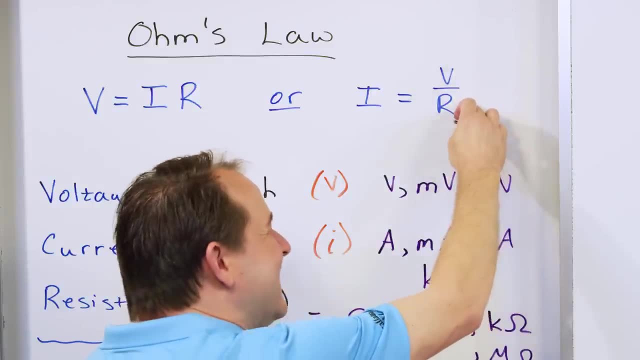 we should get 0.6 of an amp. That's what we should get. But we also know that these two little batteries, when you add them together, is also six volts. So six divided by if we do a 10 Ohm. 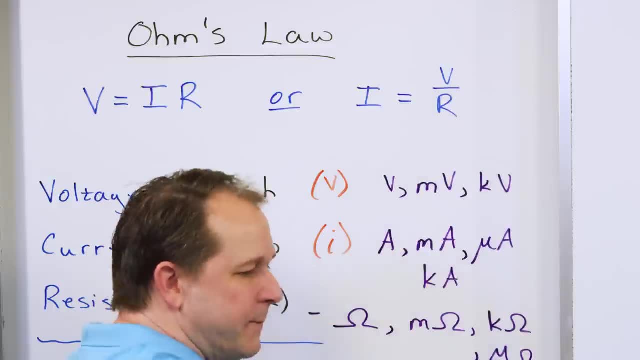 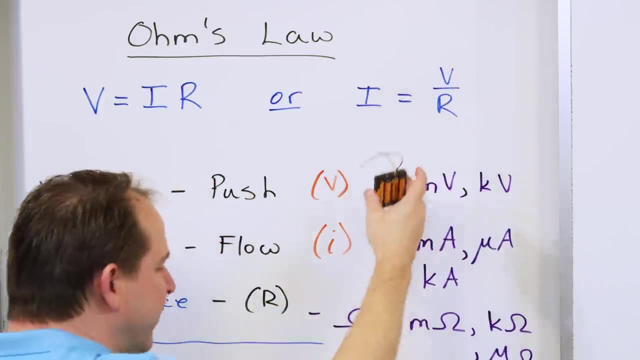 resistor. we should get again 0.6 amps supplied by this. 0.6 amps supplied by this. You can pick any of these others that we have used. This is about six volts, Six divided by again 10 Ohms. we should get the same thing, 0.6 amps, No matter what batteries we use. 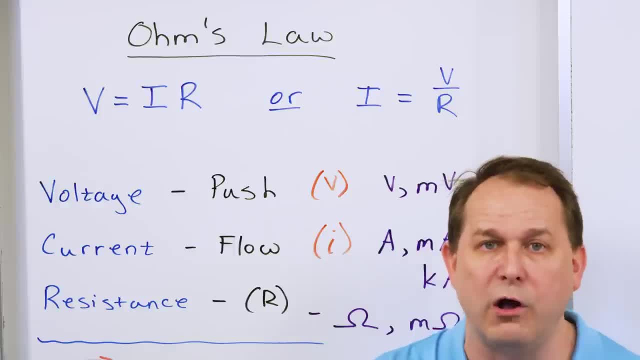 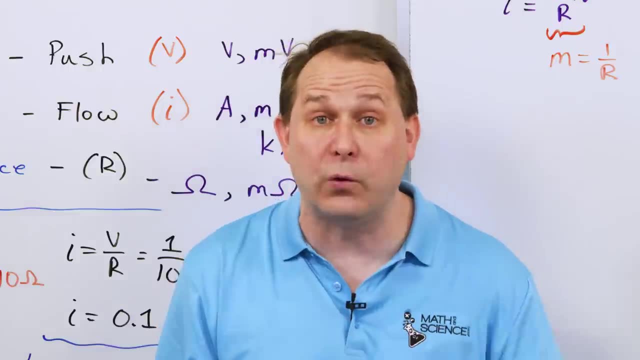 because the voltage is six volts. I've arranged them so they're all six volts. if I hook them up across this 10 Ohm resistor, we expect to get exactly what we already got before. But we're not going to get exactly what we got before. What we're going to find out. 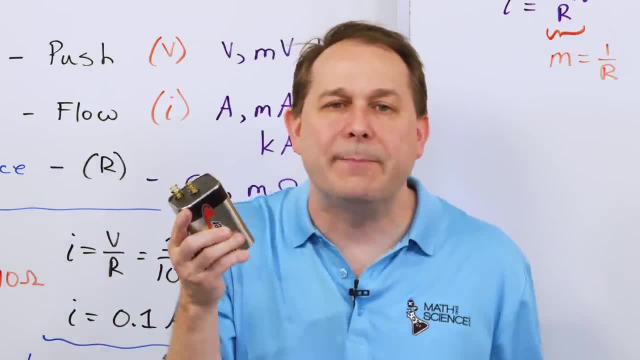 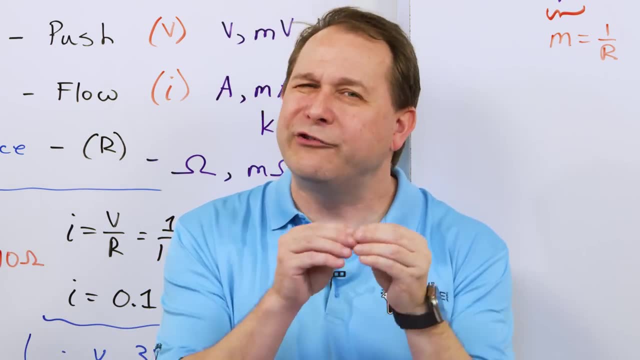 is that the physically large battery can generally keep up and supply the correct amount of current as predicted by Ohm's law. But the small batteries are going to try but they're not going to be able to physically source the amount of electricity that Ohm's law. 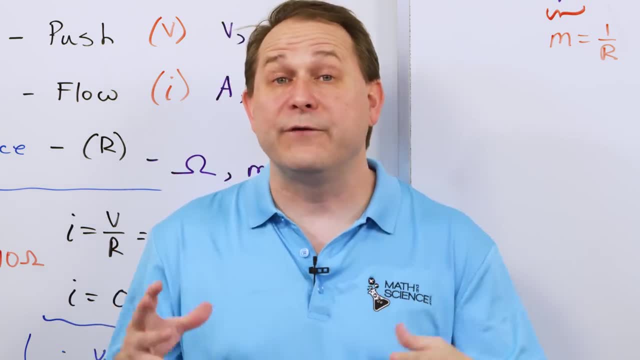 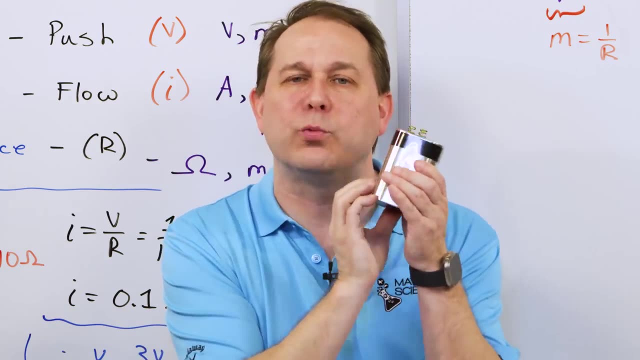 is calculating that you should get. So again, this is the difference between theory and reality. Ohm's law will tell you what you should get, But in reality, inside this battery is a chemical reaction, And I don't feel like drawing a picture because I think it'll distract us from the main. 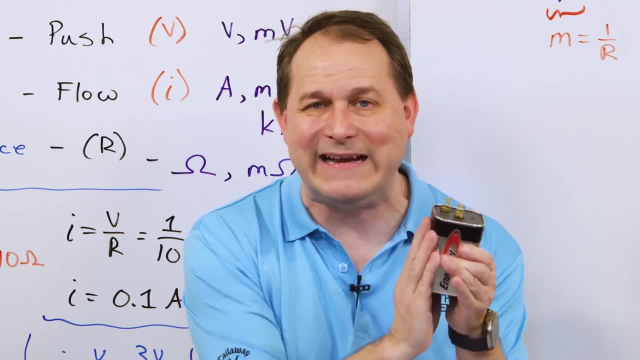 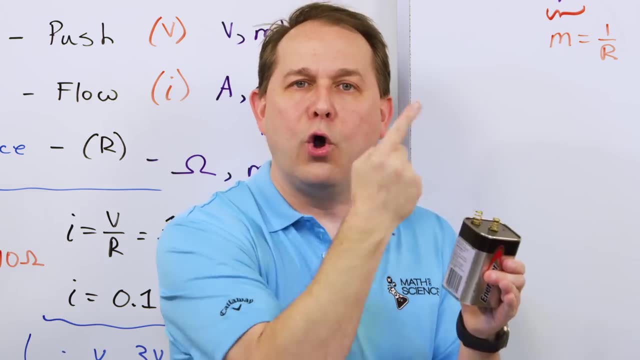 point. But in a chemistry class we would draw the picture of what's inside And I'll describe it. You have two conductors which are separated by an insulator so they're not touching, And they're rolled up like a gigantic jelly roll inside of this thing. 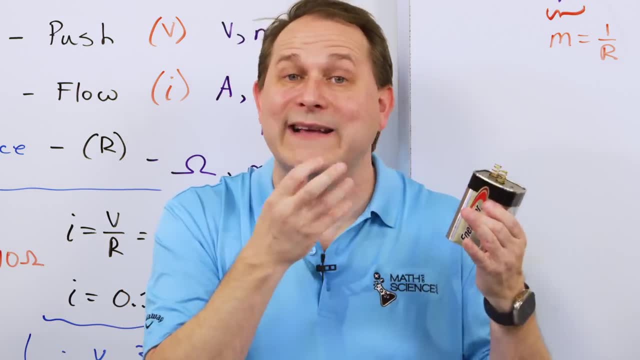 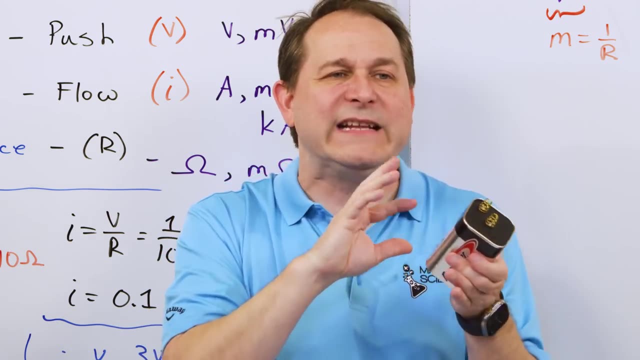 And there are chemicals inside of here that when you select the correct chemicals and the correct metals for the ribbons that are inside of here, they basically lose and gain electrons from the chemical reaction and the electrons want to come out once. one terminal of the battery. 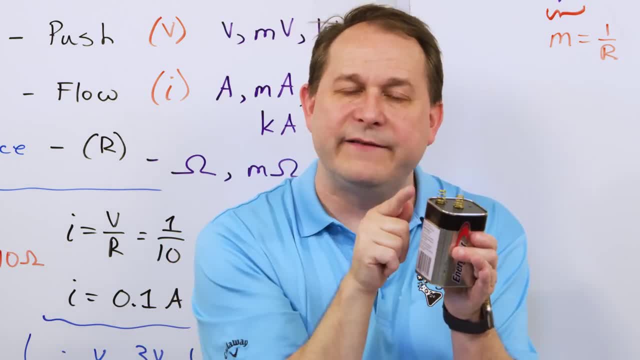 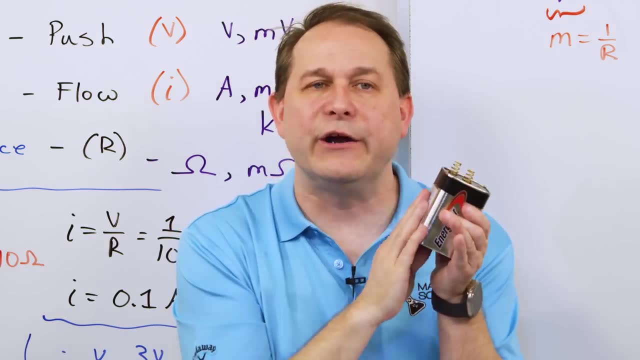 go through and then back into the other terminal. When the electrons get into the other terminal they go back through the battery and it's like going over and over again. But eventually the reactants that are in here get depleted and the chemical reaction cannot be sustained. 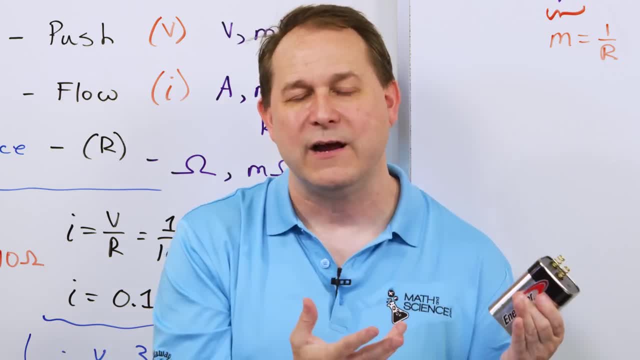 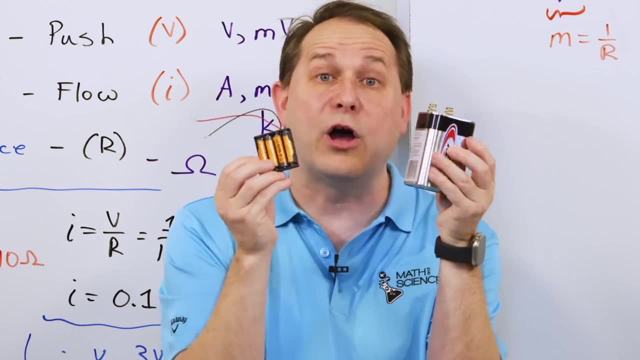 And so the battery dies. That's what we say, that the battery is now dead, right. But even though this is six volts and even though these two things are over here, this here is also six volts. There's a huge difference between them. The main difference. 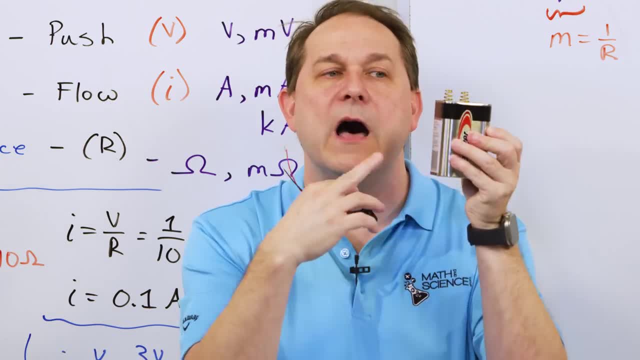 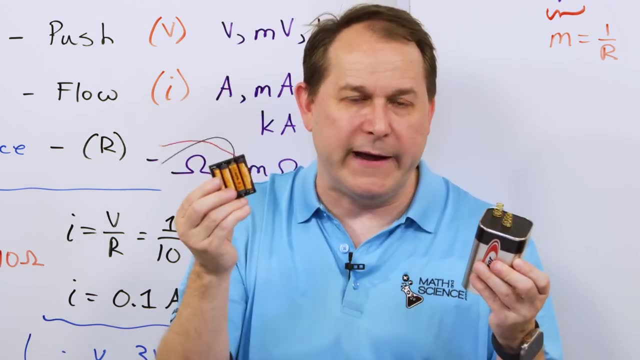 is that inside of here there's a large surface area of contact area for the chemical reaction, The reaction to take place inside of here. It's constructed in the same way or in a similar way, but there's a very much smaller amount of surface area for this chemical reaction to happen. 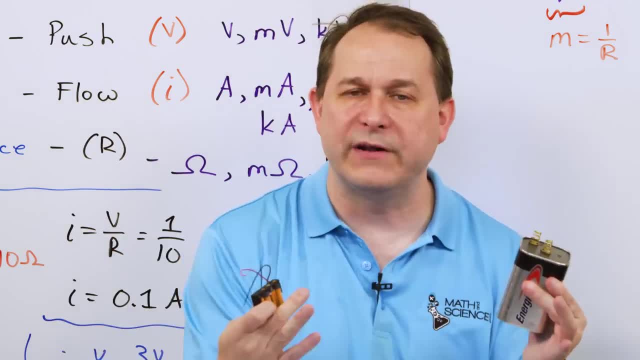 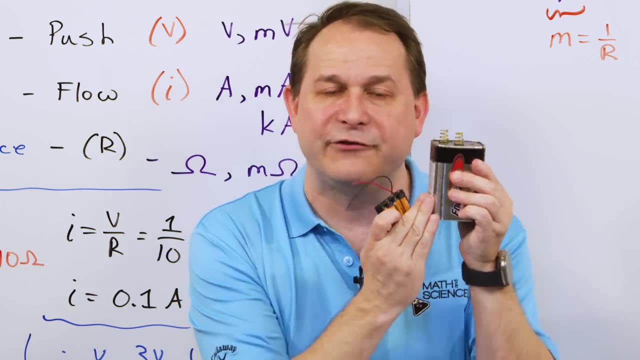 So we're going to learn that electric current is the flow of electrons per second, because inside of this thing there's a large surface area for a large amount of the chemical reaction to happen. It can physically supply the amount of electrons that Ohm's loss says. 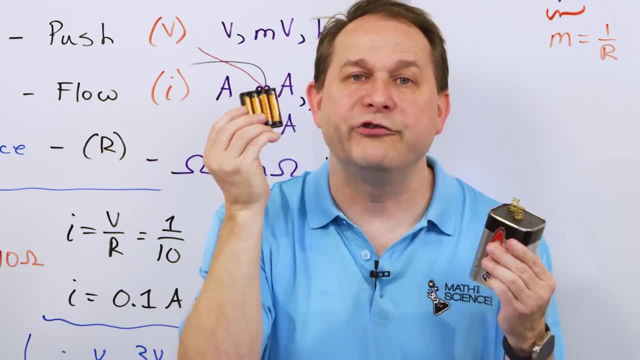 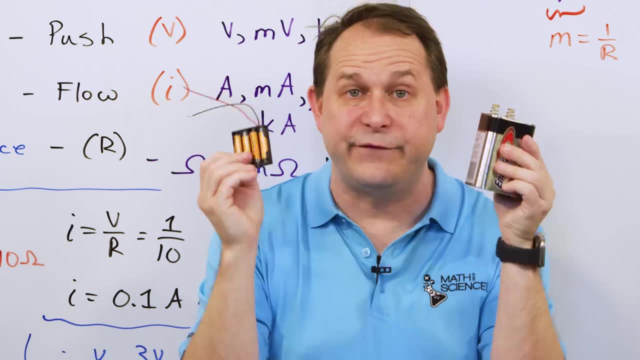 that should come out of it. But in here there is not a large enough surface area to physically produce the amount of electrons that Ohm's law would predict. So even though these are both six volts, if I hook this up to a load and I hook this up to the same, 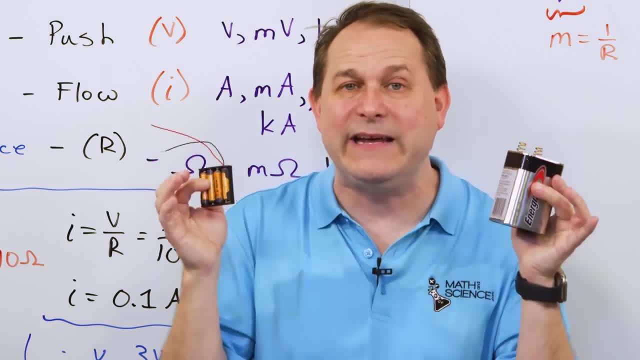 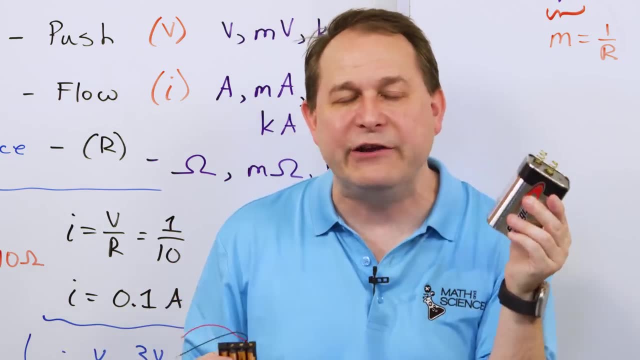 load. depending on what the load is, we might not get the correct amount of current that we predict ahead of time. So these physically larger batteries are going to be used in applications when we require a high current, And these small, tiny batteries are going to be used in applications. 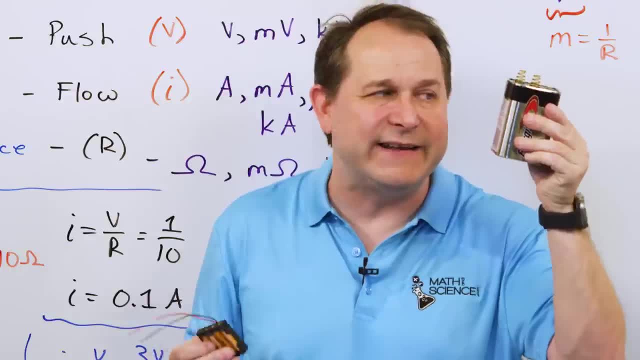 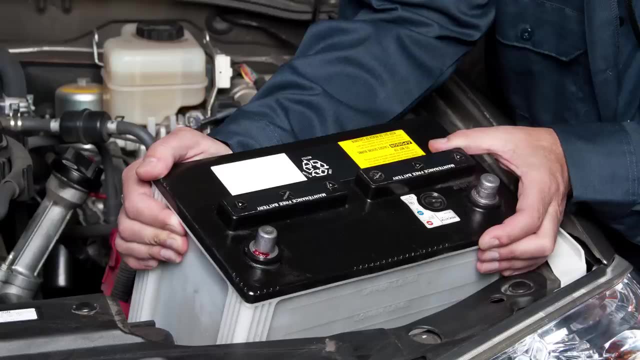 when we don't require a large current- For instance this in a lantern- to supply a very large amount of light, or a car battery- You've seen car batteries, big rectangular thing. It's used to supply many, many amps. to start an engine It has to supply a. 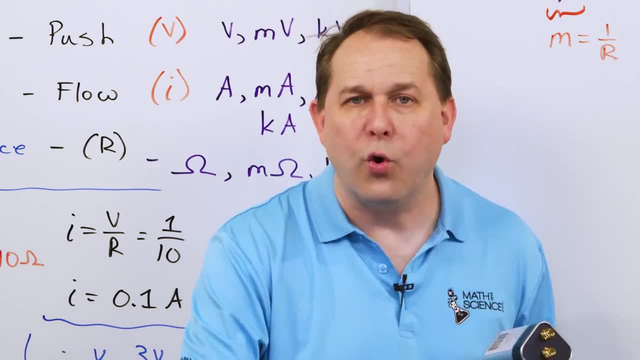 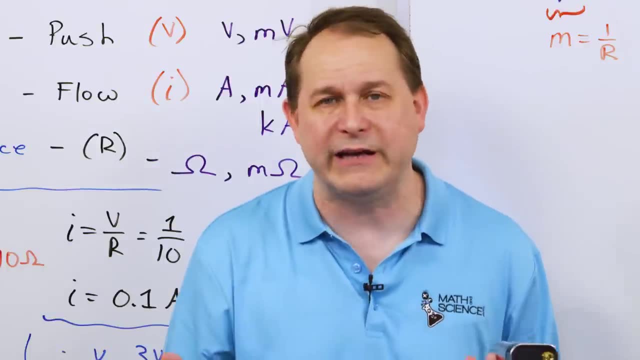 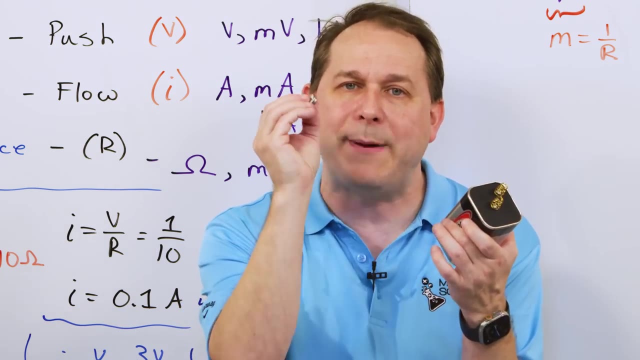 large current to be able to function. But these little batteries, or these little batteries, they're not used to start a car. There might be used in your remote control or to power your calculator. The electronics in your calculator do not require much electric current, so it's able to function just fine. We have smaller batteries. 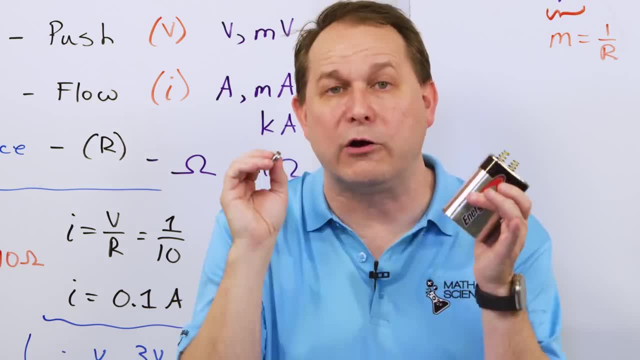 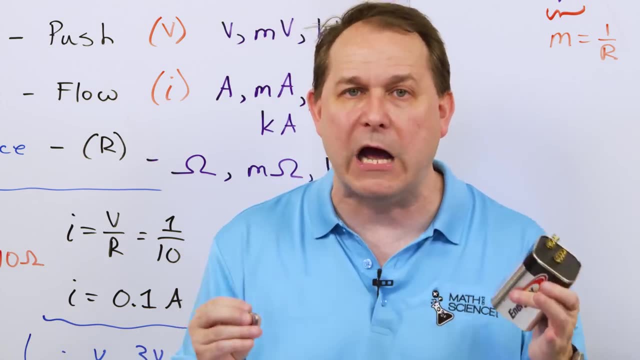 even at the same voltage, to power devices that don't require a large electric current. We have to have physically large batteries to supply current in situations where we need very high or higher electric current. Now that is the reason, And we can talk about the resistance of the batteries. 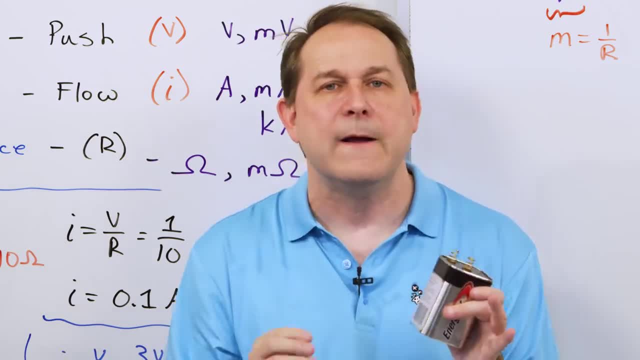 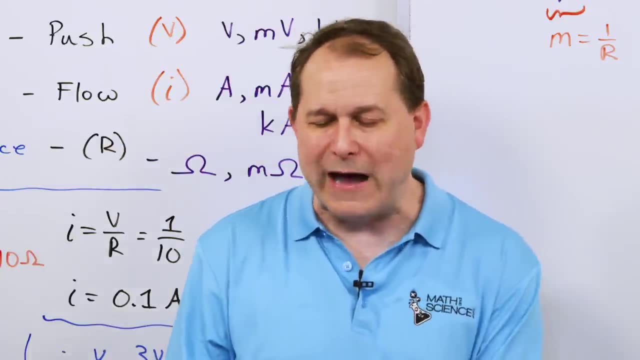 and I'll talk about that a little bit later, because you can think about it different ways- But ultimately, that is the reason. But before I discuss it any further, I want to show you that what I'm saying is correct. And in order to show you, I've devised a little experiment and I want 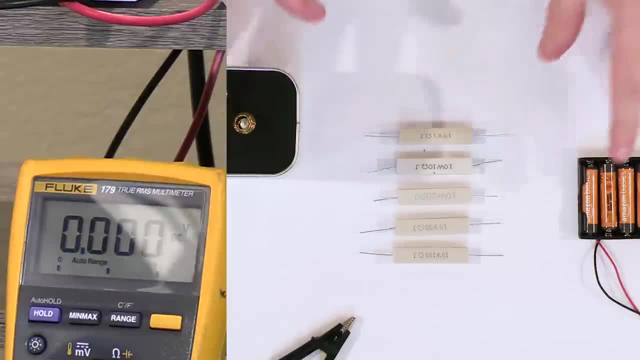 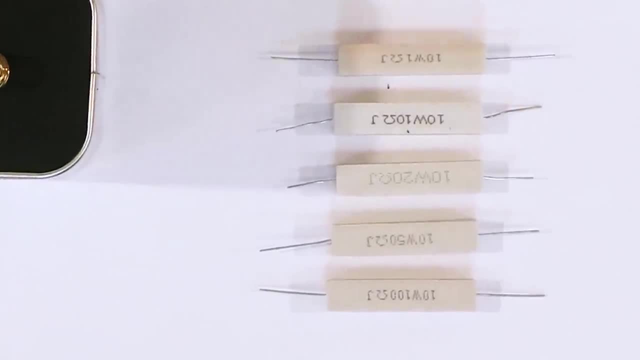 to describe that to you right now. What I want to do now is describe what we're going to do Here. I have five different resistors. They're all 10 watts, which means they can take a lot of power without burning out. I just chose large ones to not run into any problems with burning anything. 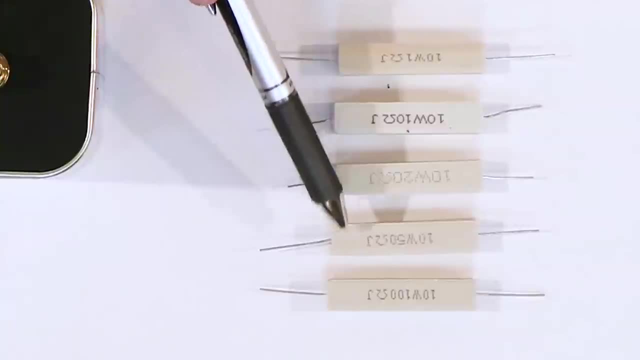 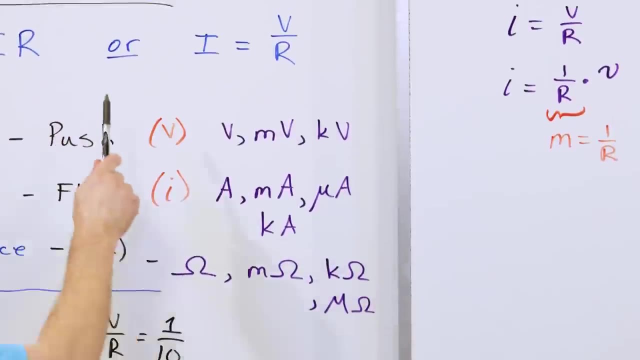 up, The top one is 100 ohms, Then we have 50 ohms, Then we have 20 ohms, Then we have 10 ohms, Then we have 1 ohm In general. what happens as you reduce the resistance? Well, according to Ohm's- 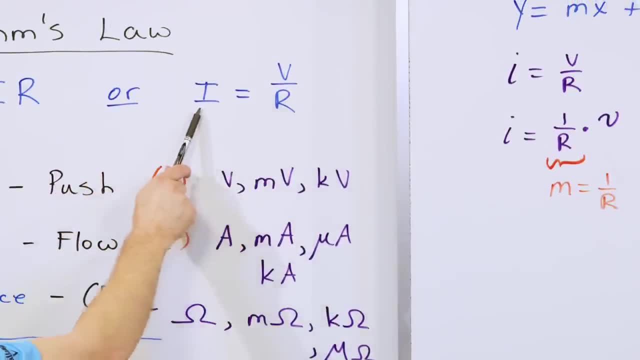 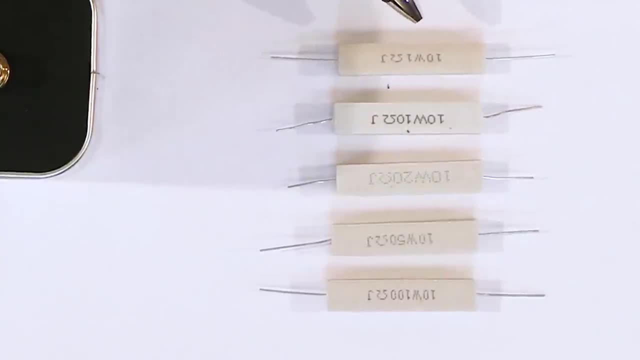 law, as the resistor gets smaller and smaller and smaller, the electric current goes up and up and up. So as we decrease the resistance in the circuit- if it's the only element in there- we expect the current to go higher and higher. What I'm telling you is that this physically 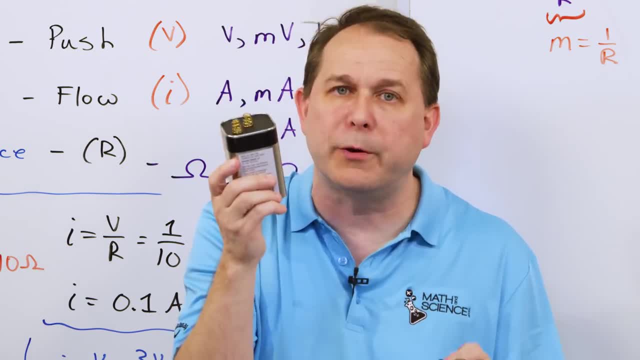 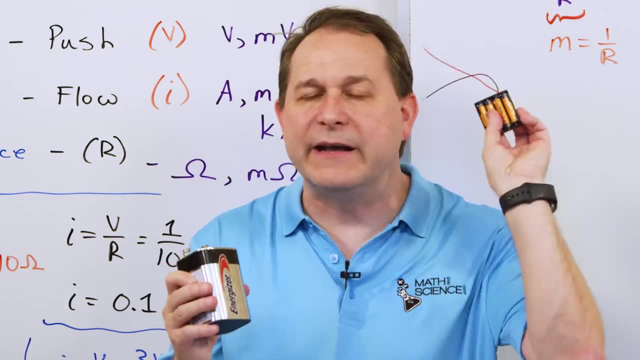 large battery is going to be able to supply more current for a longer period of time than these little batteries because they're physically smaller, Even though in theory you would think they would do the same thing. they can't because this one is just not large enough to supply the 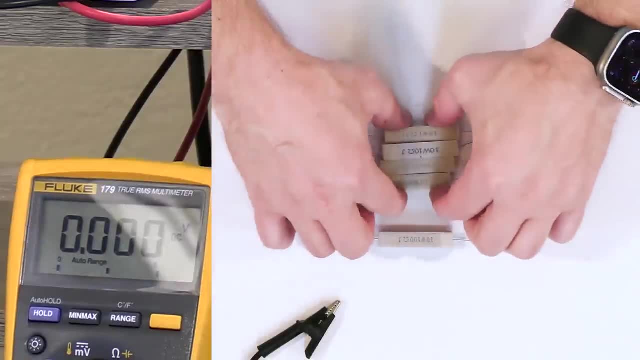 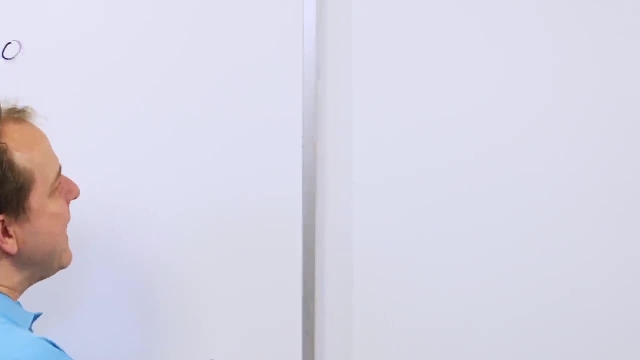 required amount of current. So what we're going to do is we're going to start off with only the 100 ohm resistor, And we're going to start off with the 100 ohm resistor And we're going to hook it up to a battery. here It's a 6 volt battery And I have a table on the board that. 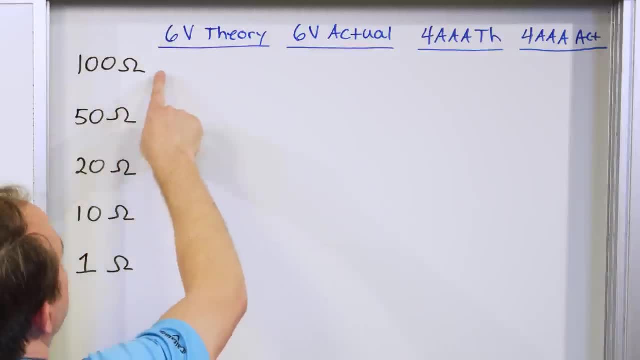 we're going to fill out. The first resistor in the list is 100 ohms, And we're going to, in theory, calculate what the current should be in this case. What should the current be For 6 volts and 100? 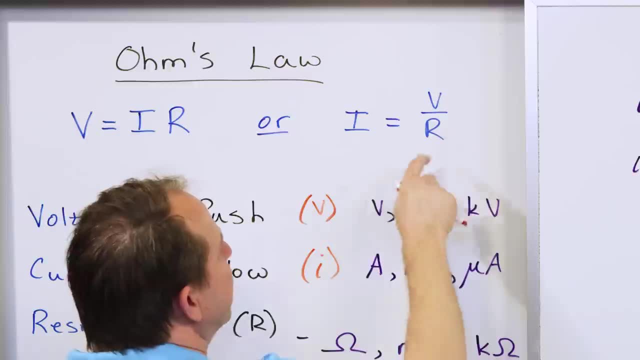 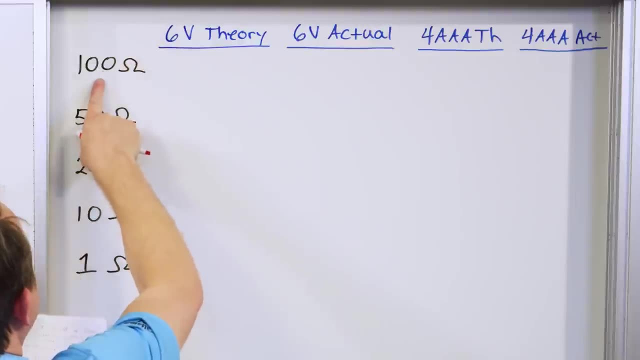 ohms, how do we find the current? According to Ohm's law, I is equal to V over R. You need to say that 50 times I is equal to V over R. I is equal to V over R. So 6 divided by 100, V over R. 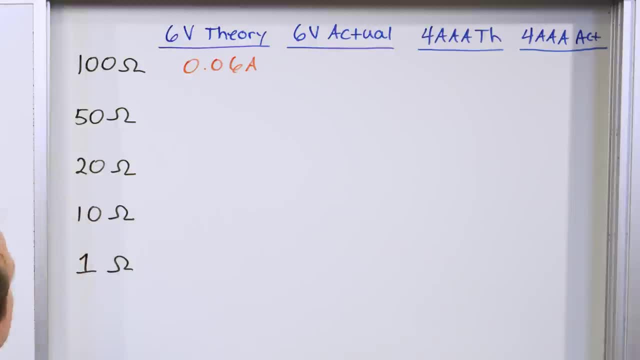 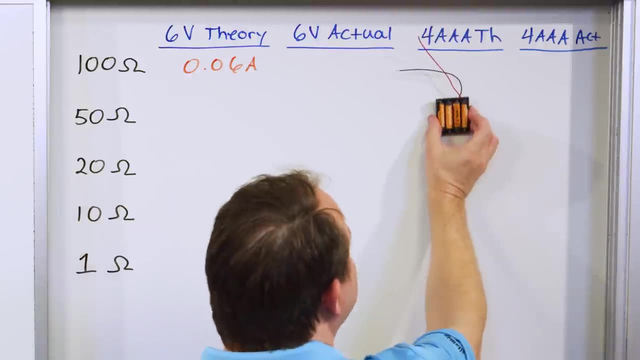 should be 0.06 amps. Now we already said that- four AAA batteries, which is what I was holding up right here. this is also about 6 volts. Yes, I know it's a little more than 6 volts, but I'm. 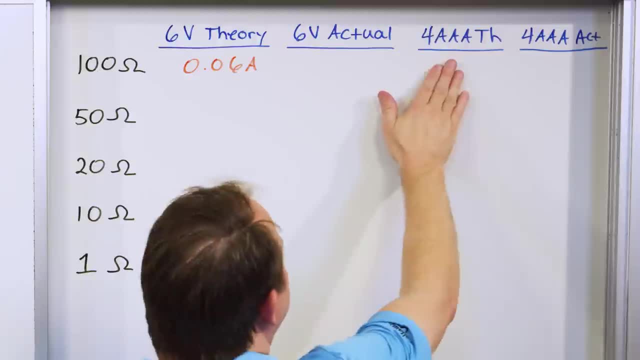 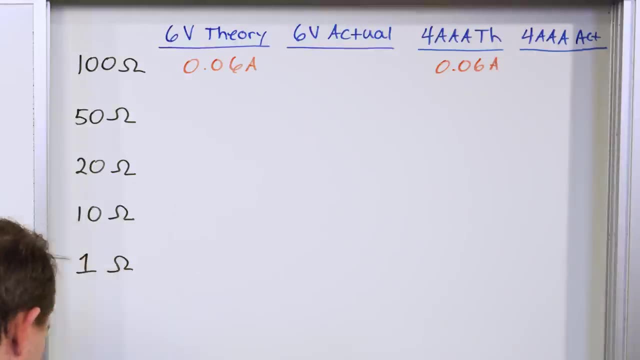 rounding to make the math a little easier. But this is supplying about 6 volts, So in theory that's what the TH is. in theory it should supply also 0.06 amps. What's going to happen when I change the resistance and cut the resistance in half? Well, 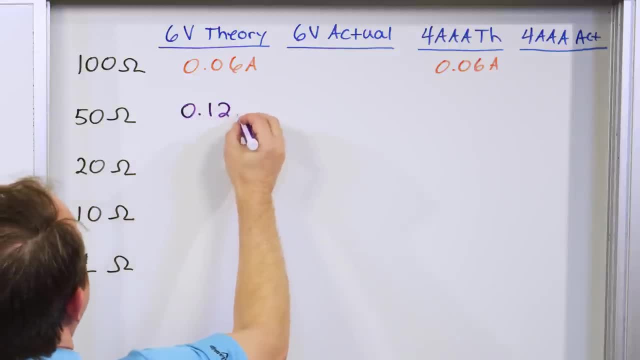 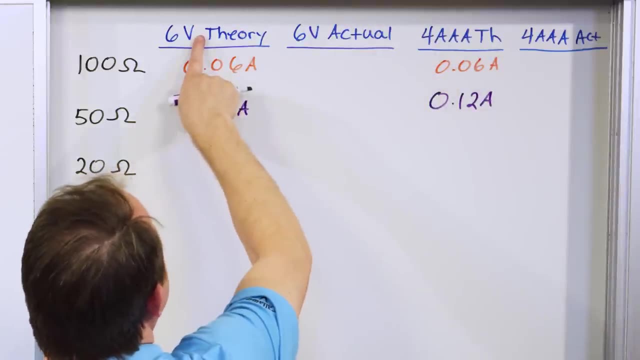 I'm going to get 6 divided by 50, and I'm going to get 0.12 amps as my theoretical current 0.12 amps as well. The reason it's the same is because this is a 6-volt battery and this is. 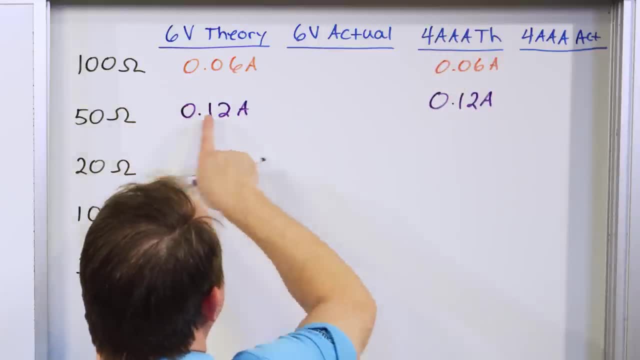 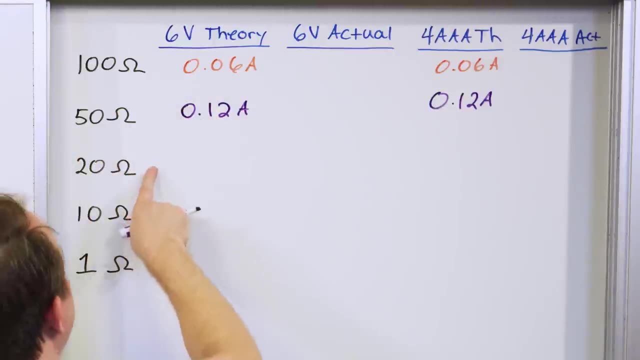 for AAAs, which is also 6 volts. So across the same resistor it's going to give you the same thing. Notice: this current is exactly double this because I cut the resistor in half. What happens when I get to 20 ohms, 6 divided by 20, 0.3 amps, And over here, the exact thing. 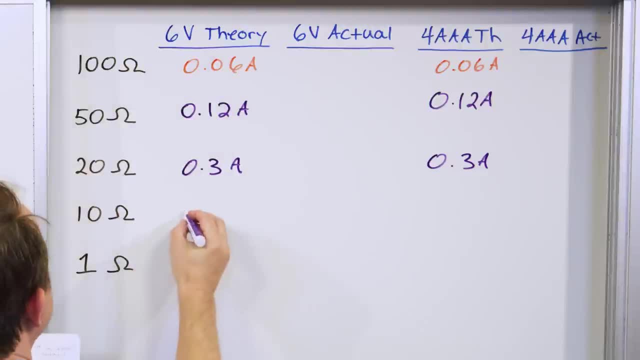 0.6 amps. What happens when I get to 10 ohms? 6 divided by 10, 0.6 amps And over here, 0.6 amps. What happens? over here? 6 divided by 1 is 6 amps, And over here what happens? It's going to be also. 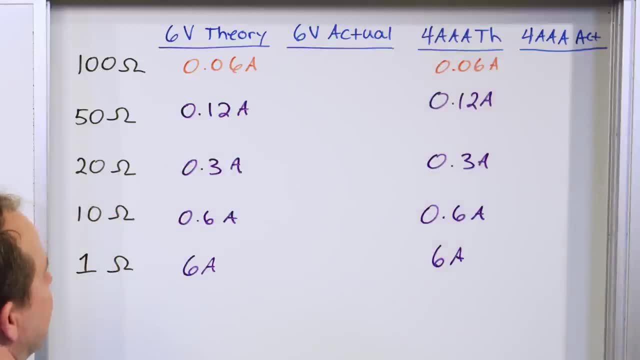 6 amps. I can tell you right now, these little AAA batteries are never going to be able to give you 6 amps. In fact, I'd be very surprised if this large battery could even do it, because you need a physically large battery to supply that many electrons per second to keep up with what Ohm's law is telling you should be. 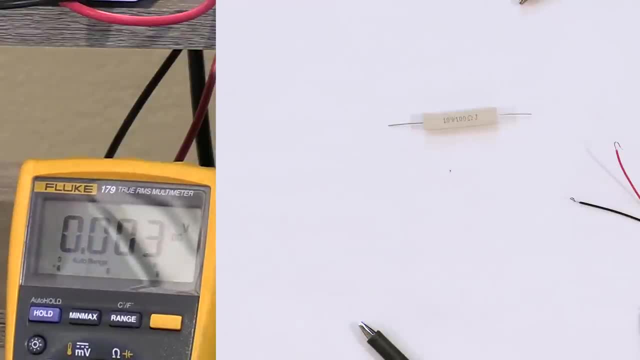 be happening All right. so let's go ahead and do our little experiment. What we're going to do is use the 100 ohm resistor and we're going to hook up this battery to it and we're going to measure the. 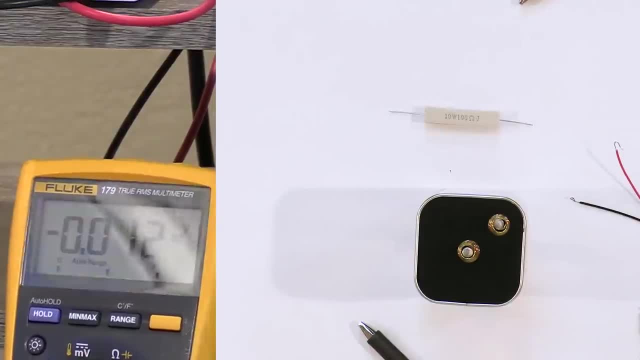 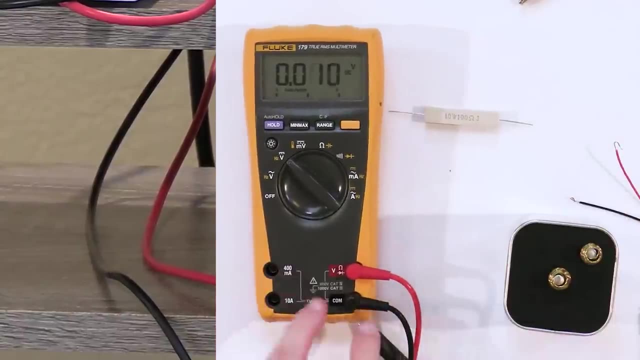 electric current. Now we have to learn how to measure current. The way I have this meter set up right now is as a voltmeter. So your meter, whatever meter you have, might be a little different, but you can see that to measure voltage with a V right here, you have to have it over here To measure. 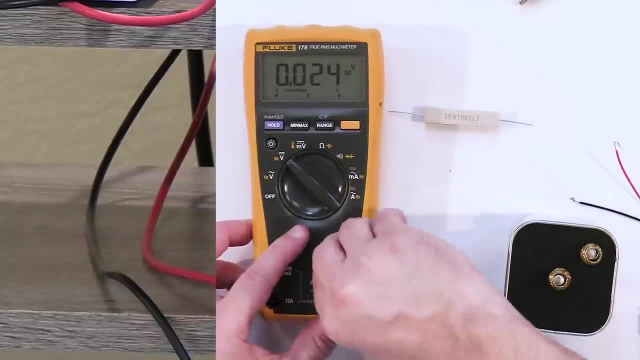 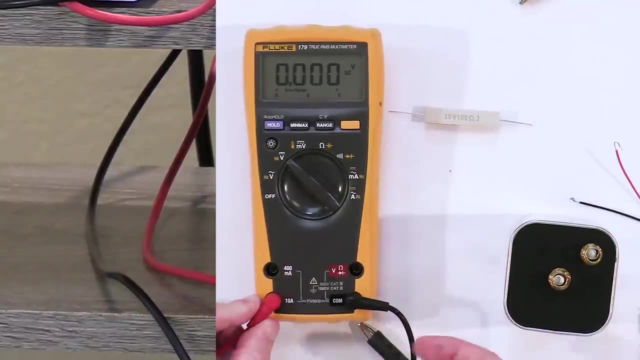 electric current. the electrons have to flow through the device, So you can't connect it here, you need to connect it over on the other terminal. If you're measuring current, you have to push the current through the device, so it has to be connected over here. So I'm going to put 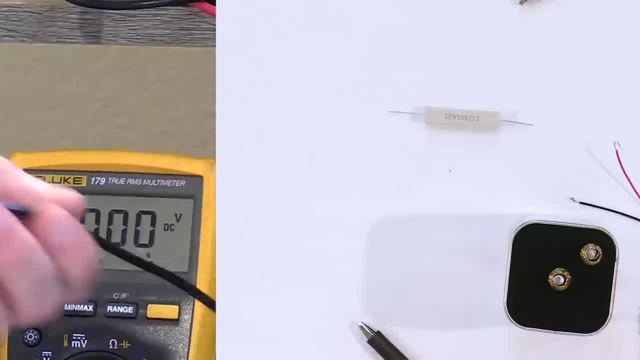 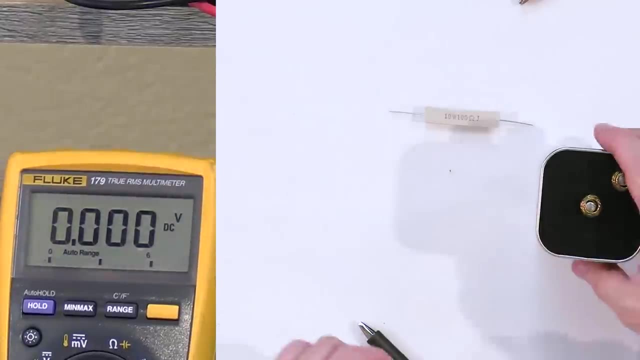 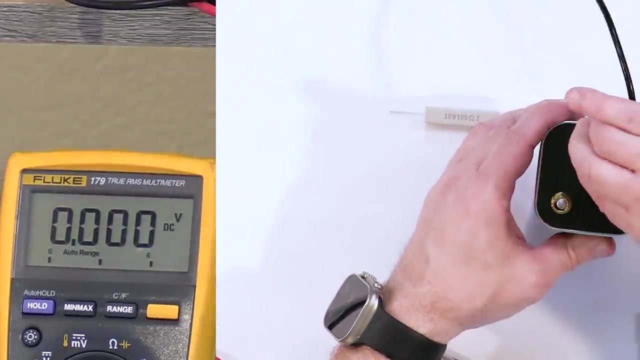 this back where it is, and what I need to do is I need to let the current flow directly through from the battery into the device there, into the measurement device and so on. So what I'll do is I'll clip this battery, I'll connect it right here. 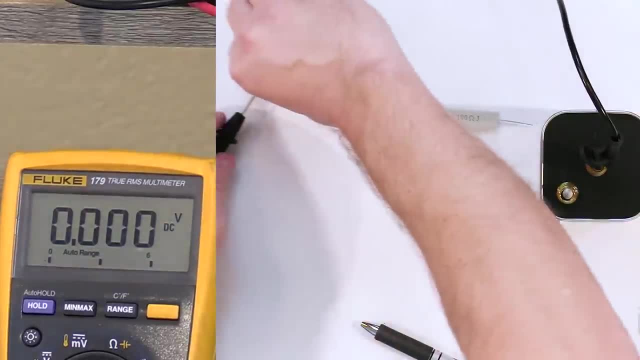 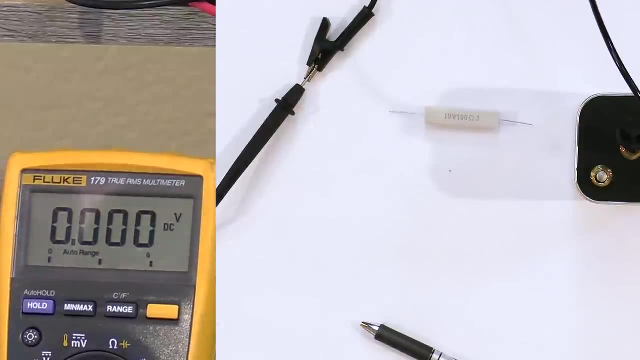 and then it will come over and I will connect it to. I'm connecting it right here to my ammeter over here measuring the electric current right, And then it's going to go through the meter and then the meter is going to come over here where I'm going to connect it. 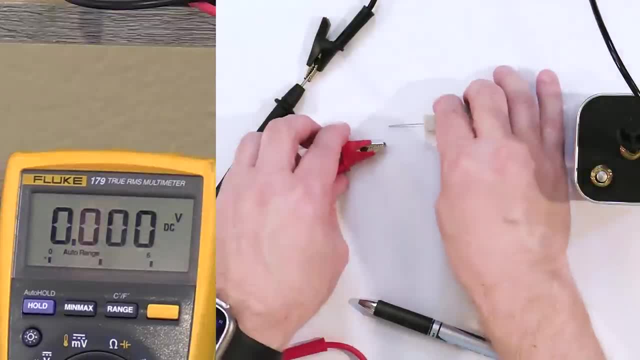 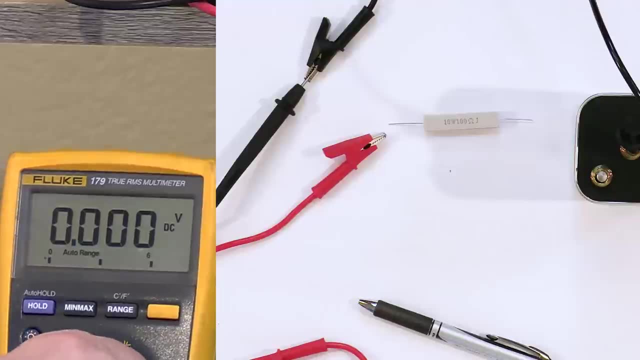 back through the resistor again. So all I've done. I'm still connecting it directly through here. I'm connecting it through here, but the current is also flowing through my meter so that I can measure. And then I got to switch it over to amps right here, And so now I'm going to 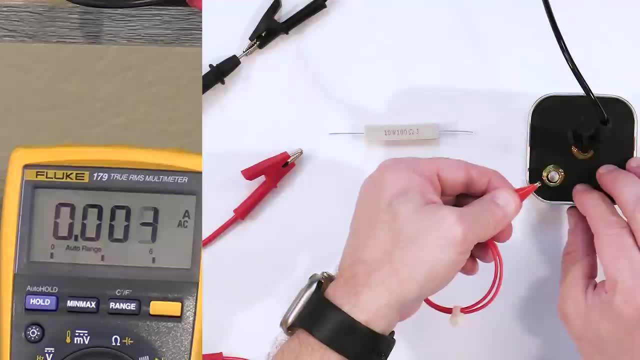 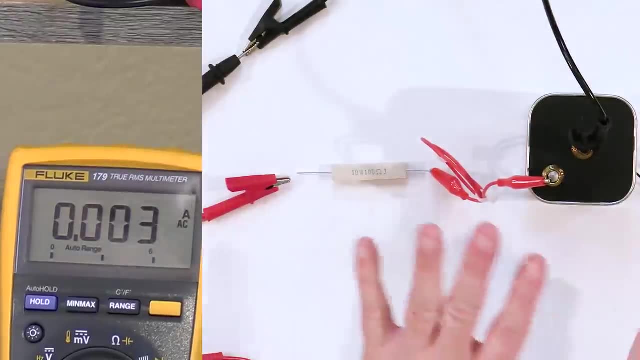 connect it to both sides, All right. so I'm going to connect this side of the battery here, I'm going to connect to the resistor right here and I'm going to connect it over here. So all I've done is connect it in series, where my meter is also in series with this resistor, and I will 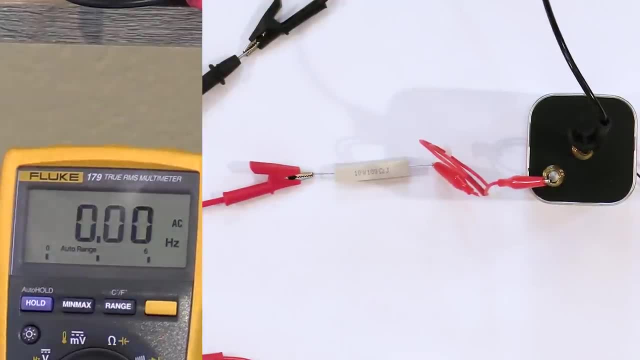 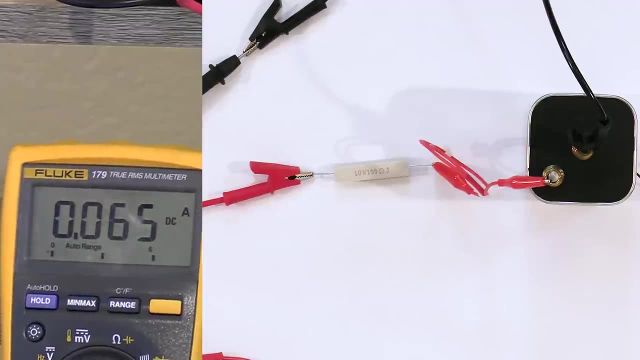 connect it right here. And I realized for this one you have to press this button right here. This is trying to measure AC current, so I need to press the button until it says DC. So now the electric current is flowing through the resistor, the 100 ohm resistor, but also through the meter, and it's telling me zero ohms. 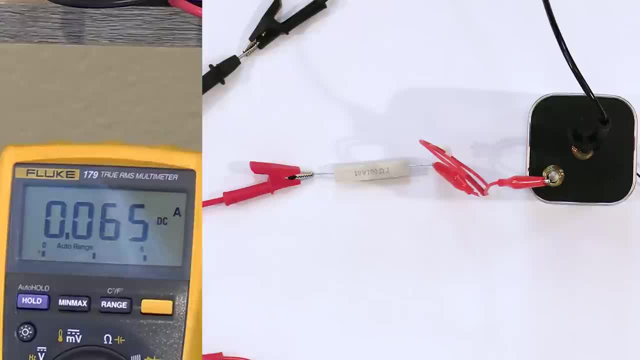 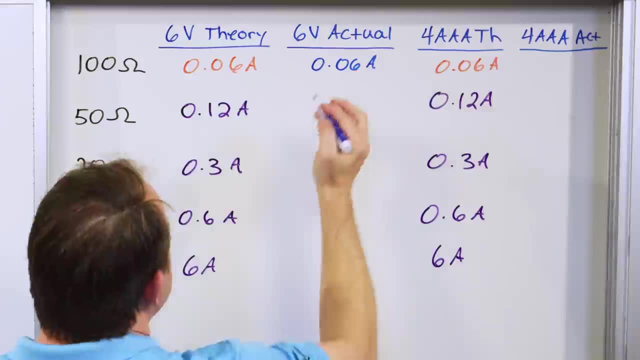 So I'm going to go over here and put 0.06, roughly- amps, which is exactly what I calculated should happen. So I'm going to go over here and put 0.06 amps there. So Ohm's law is calculating what I should. 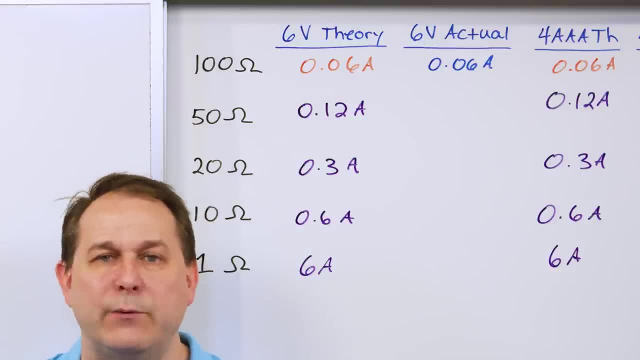 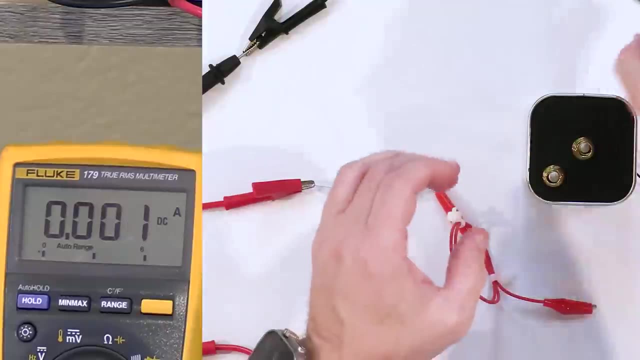 get in terms of the current. When I physically measure the current, that's exactly what I get: 0.06 amps. So let me disconnect that over here and I'm just going to disconnect the large battery. I'm going to put it to the side and now we're going to connect the small batteries to it And 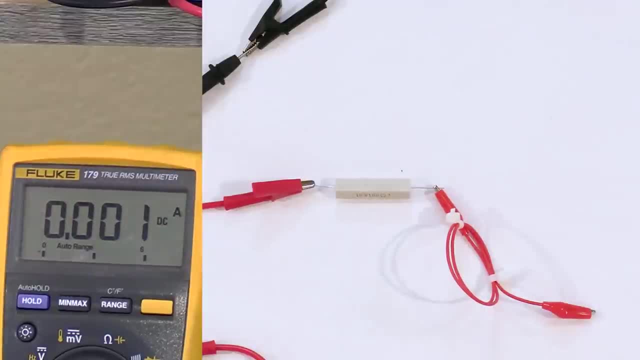 we can use either these. Just to make it a little more interesting, let me grab the AA versions, which I think are a little bit fresher. I haven't used them at all. So here are the AAA batteries. Again. adds up to 6 volts. We already verified that, measured that. So what I'll do is I'll connect. 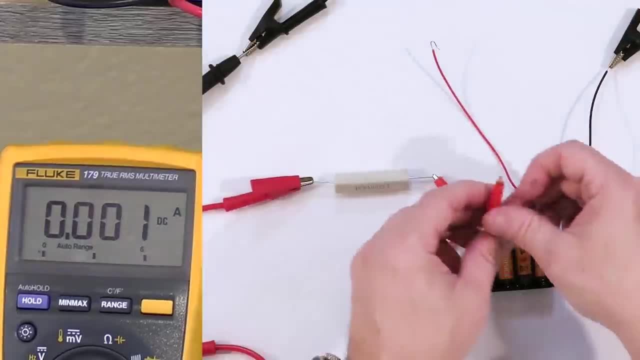 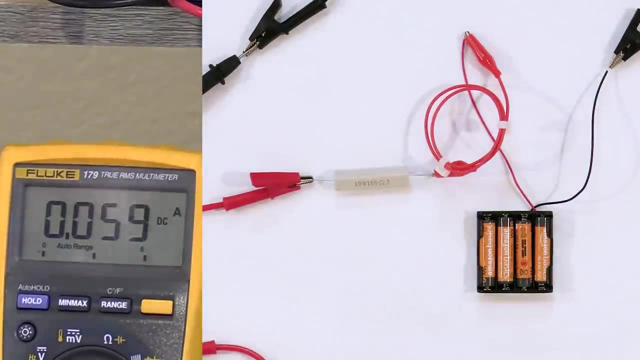 one side over here, right, And then the other side. all I've done is replace the battery and we're going to measure over here what's going on. What did we get? 0.059 amps, 0.059.. 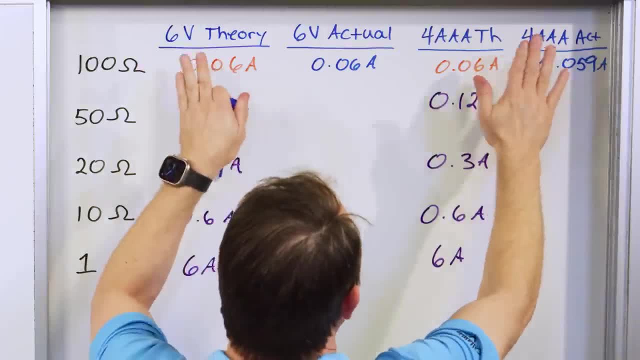 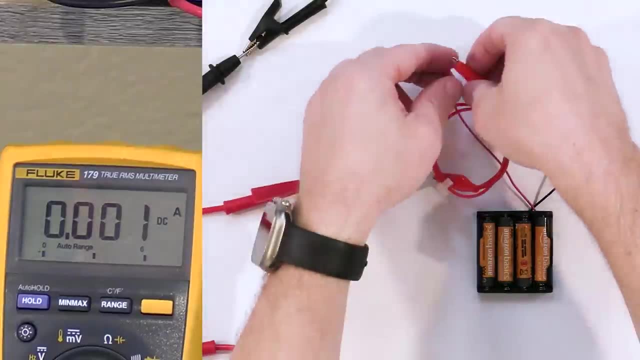 Amps, which is very close to 0.06, and the voltage of the batteries is not quite the same. So it's basically agreeing with theory perfectly. So I'm going to take this off before we drain our batteries. I don't want to drain the battery, So when we are not asking the circuit to provide, 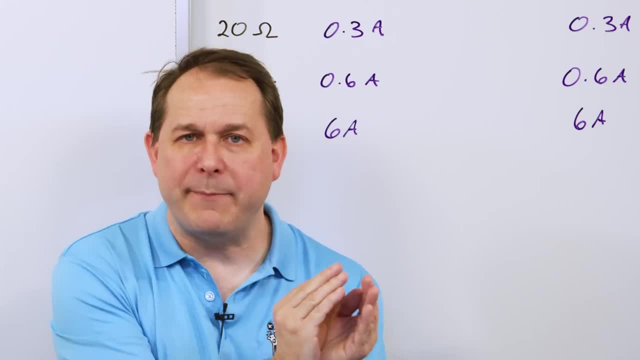 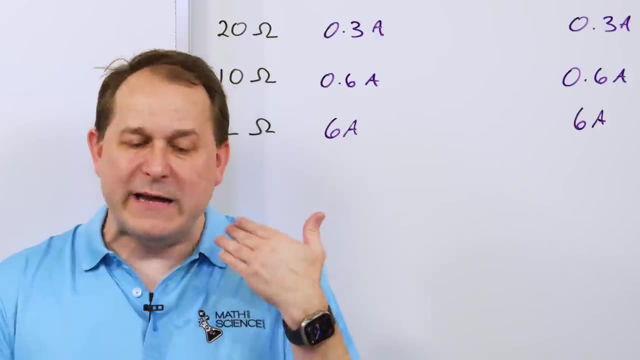 very much current. both the large battery and the small battery are able to keep up. There's enough surface area and chemical reaction in this little bitty battery to enable to supply this many amps through the circuit, And so that's what I'm going to do. So I'm going to take this off and I'm going 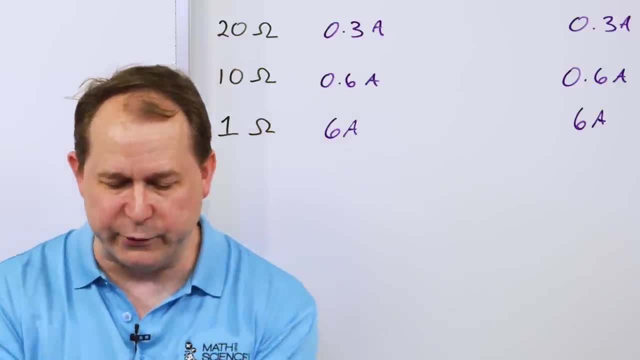 to put it aside, so I don't accidentally use it. And that's why it agreed with theory and there was really no difference. So now what we're going to do is we're going to take this resistor out, which was 100 ohms, I'm going to put it aside, so I don't accidentally use it, And I'm going to go. 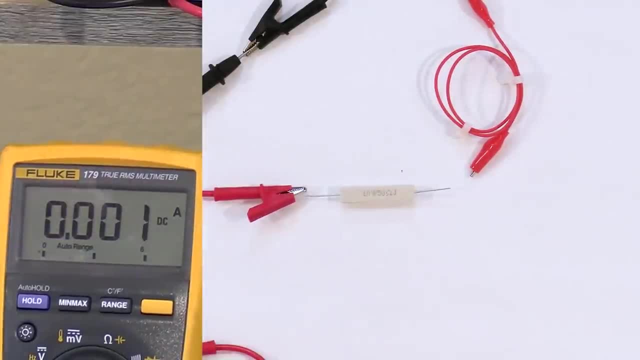 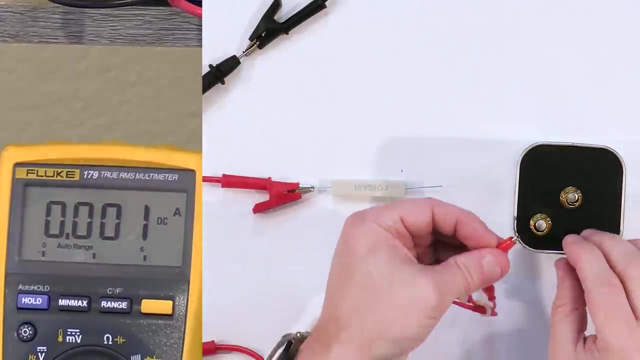 down to my next resistor. This is half the resistance which is going to double the current there, And this is a 50-ohm resistor. So we said for 50 ohms we expect the current to exactly be doubled, 0.12 amps. So what I'll do is I'll connect this guy over here and we'll see. 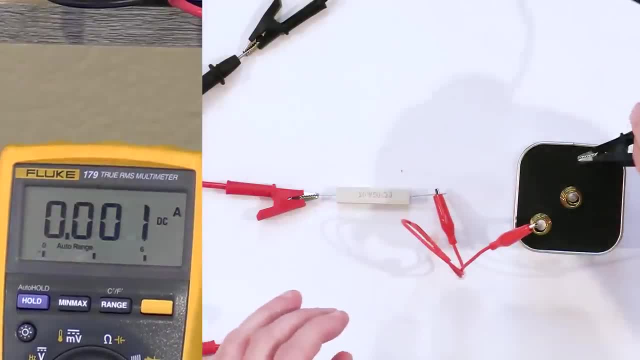 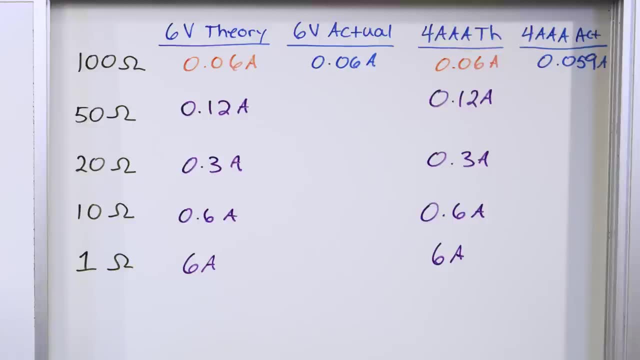 exactly what it measures right here. Let me connect it like this. What do we have? 0.125 amps. That's what we're measuring- 0.125.. So I'll put 0.125 amps. It's bingo right on the money. 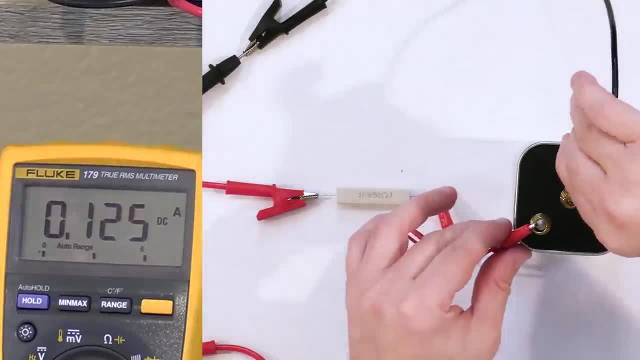 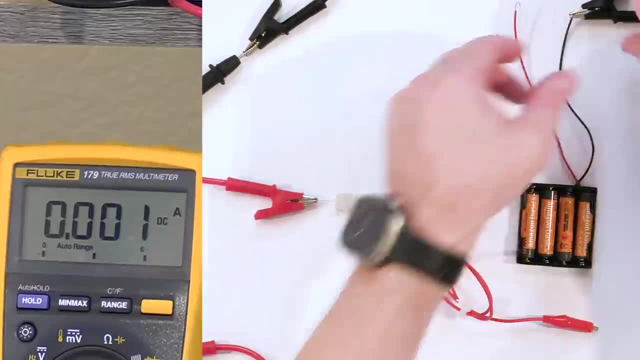 able to supply the amount of current as requested by the circuit. OK, so now we'll disconnect this, And now that we know what we're doing, it's going to go a lot faster. I don't have to explain every single thing. We're just going to connect these smaller batteries up to it. 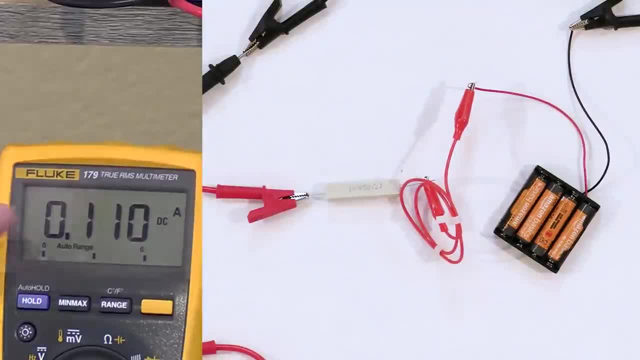 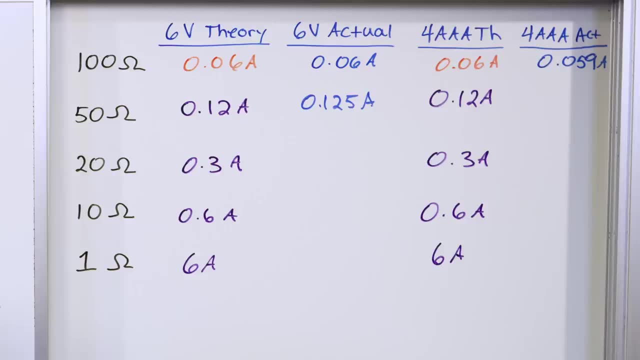 And see what we get. OK, now we get 0.110.. Let me make sure I have a good connection here, just to make sure there's no connection problem. 0.11.. Let's round up: 0.111, right, So we have. 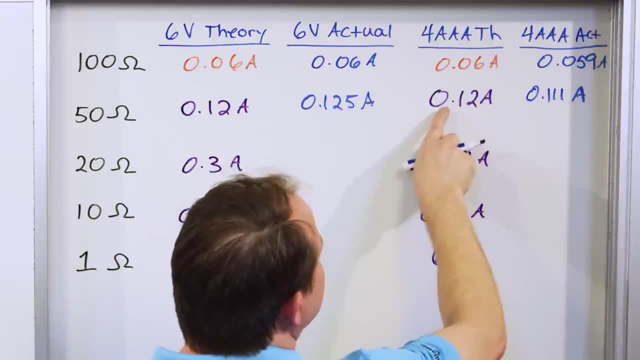 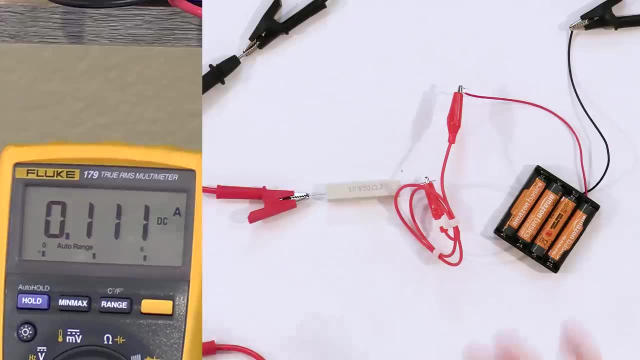 0.111 amps. This is still pretty close because it's 0.12, 0.111.. It's a little bit lower, but it's actually pretty good. I would say that that's still agreeing with that. So even asking. 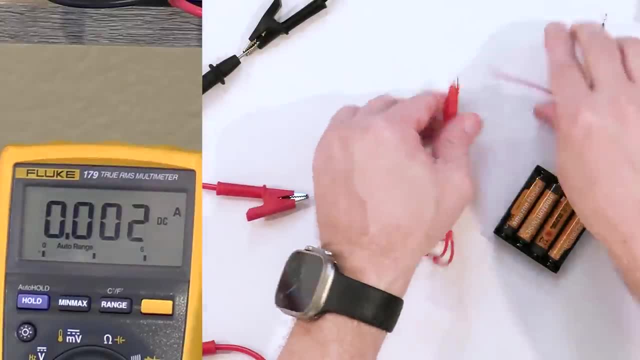 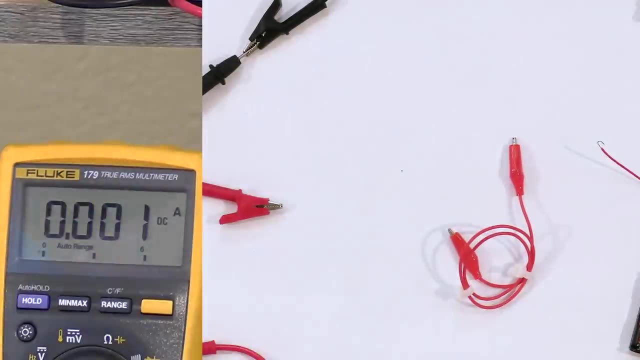 for double the current, it's able to keep up. So let me go ahead and take this apart. We're going to put this aside And I'm going to take off this 50-ohm resistor. I'm going to put it aside, And now we're going to. 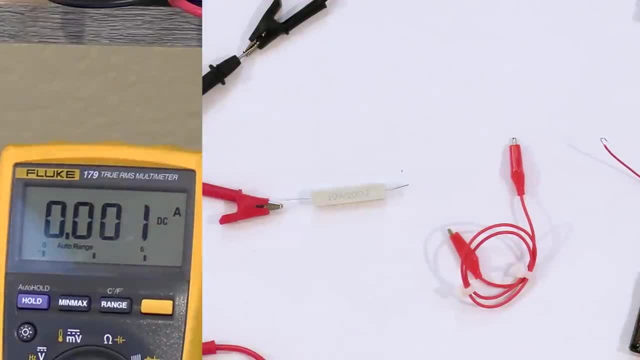 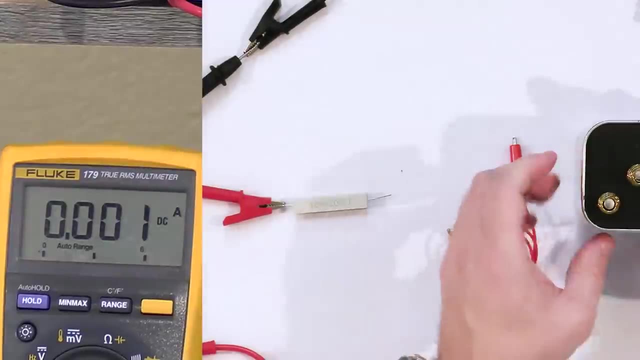 lower the resistance to 20 ohms. For 20 ohms, same voltage, we expect 0.3 amps to be able to be supplied. So I'm going to connect this here. I'm going to put the battery, connect the battery. 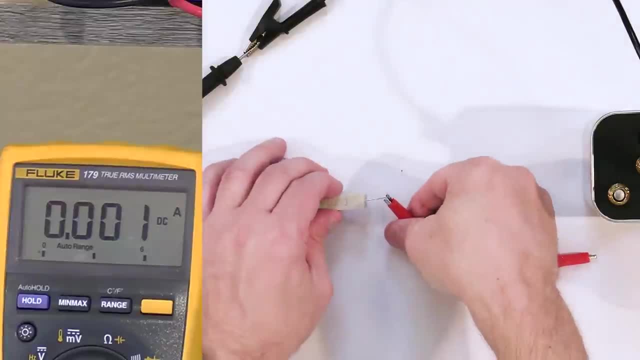 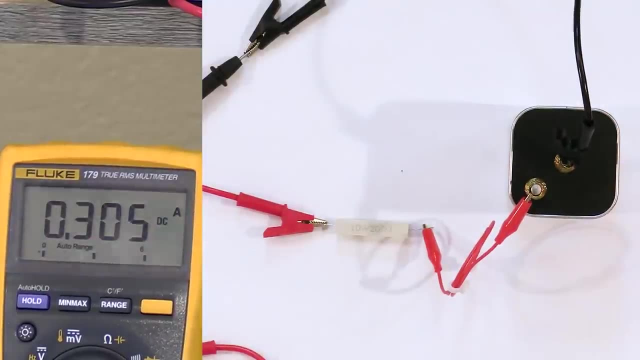 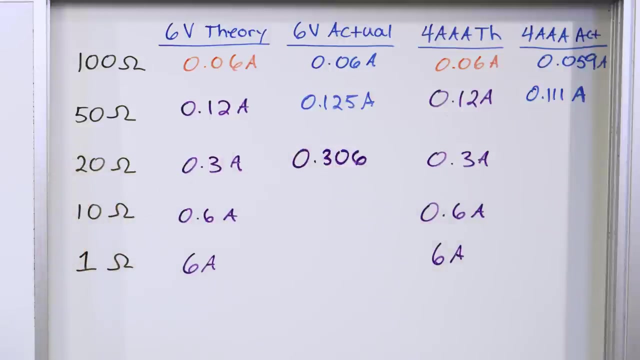 right here And I'm going to connect the other side of this resistor. This is a 20-ohm resistor here, And what does it give me? It gives me 0.306.. So 0.306 is what this guy can supply, So they match exactly. All right, Now I'm going to take 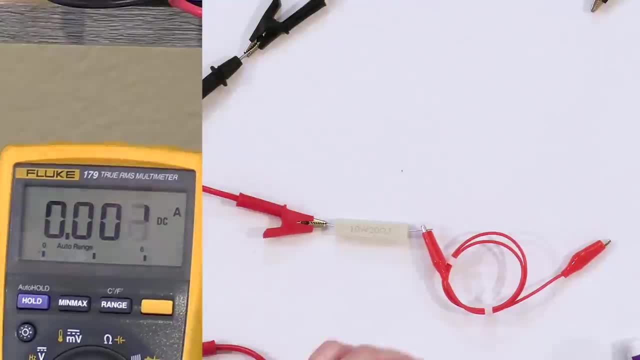 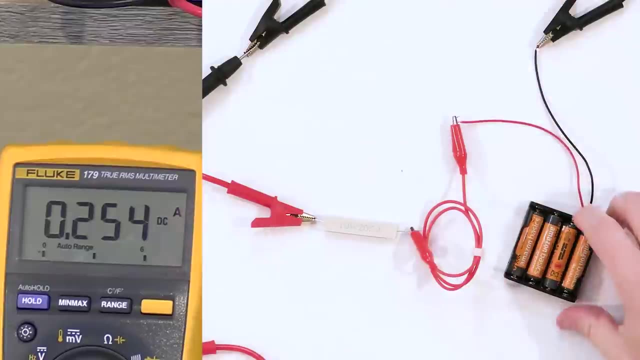 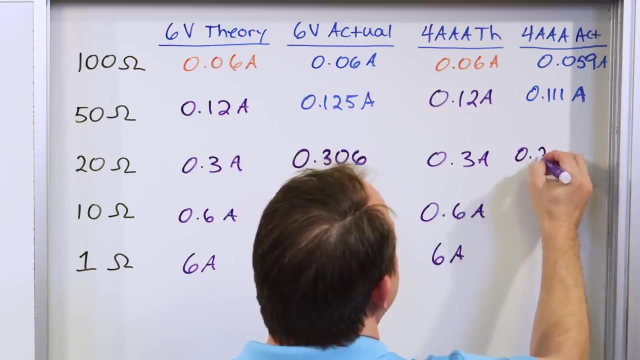 the large battery off. put it aside. I'm going to grab the smaller battery right here And we're going to see what it can supply. 0.3 amps, Let's see. Ooh, that's a little different. It's not 0.3.. 0.252.. 0.252 amps. So clearly there's. I'm going to disconnect it before I. 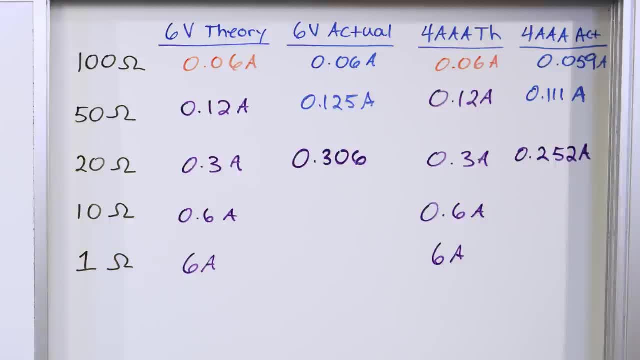 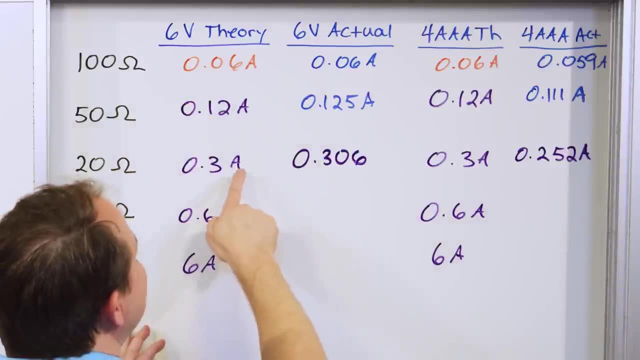 start draining the batteries down. I don't want to influence our experiment, But you can see that right here, somewhere between here and here, is when the break happened. What's going on here is this physically large battery is able to supply enough current. in accordance with Ohm's law, It's. 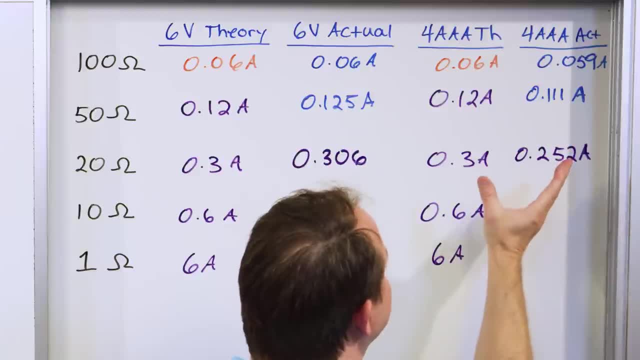 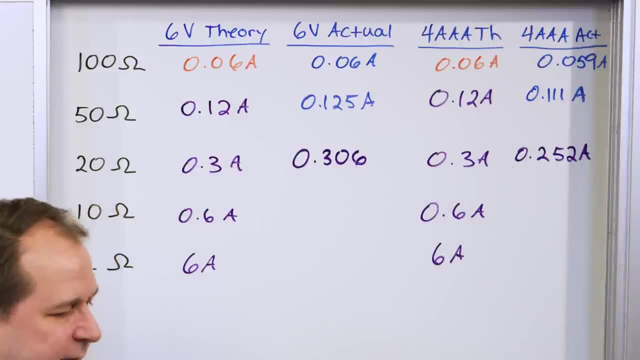 bingo right on the money. But the physically smaller battery, even at the same voltage, is really unable to do so. It's not able to keep up And you can start to see it break with what the theoretical value is. But let's keep going, because I have more resistors and I bought them. 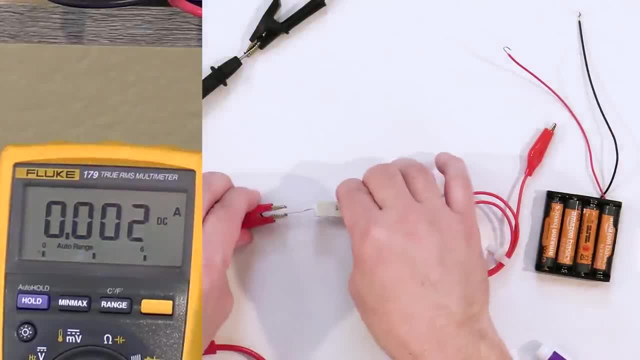 and I want to see how far we can take them. So I'm going to go ahead and turn this off. So we're going to go to 10 ohms here And I'm going to take this one away and we'll get the. 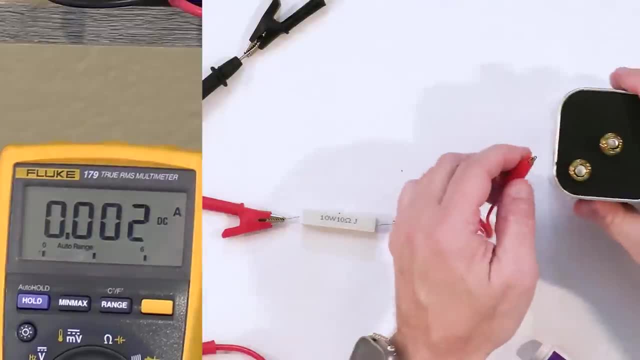 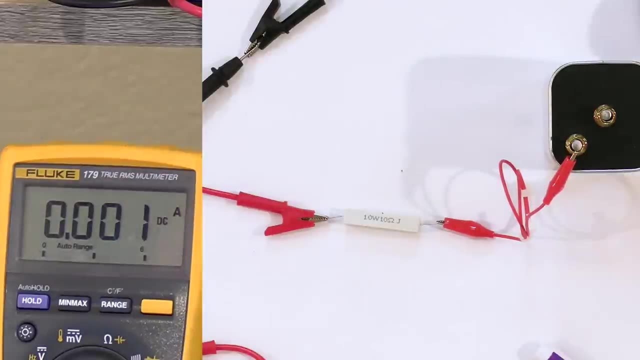 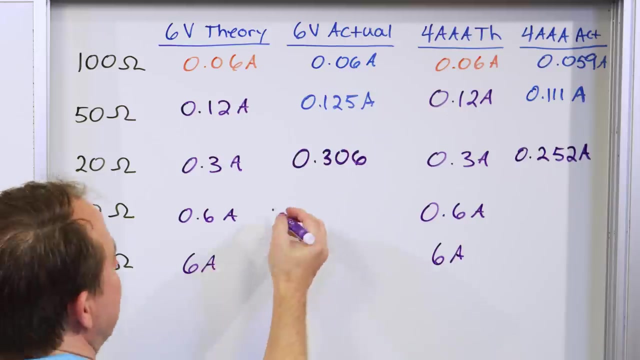 large battery, And let's see what the battery is able to supply. here The theoretical value at 10 ohms should be 0.6 amps. It's starting to actually be quite a bit of current And what we get here is 0.562 amps. So that's pretty respectable, but not quite 0.6.. 0.562. 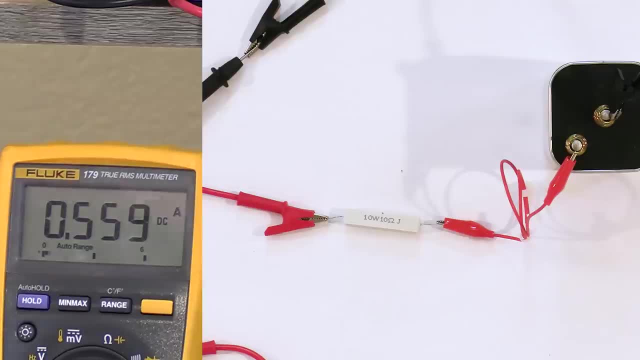 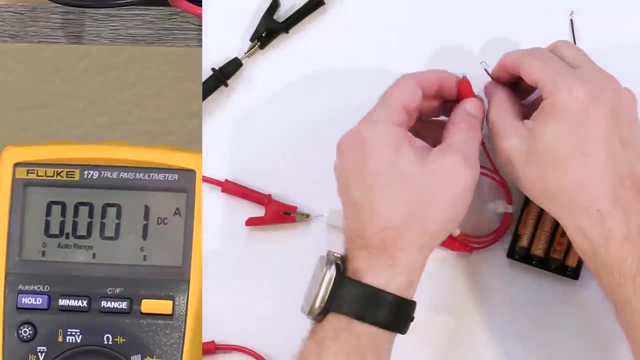 amps But it's able to supply And notice it's going down a little bit here But it's able to supply pretty close, I would say, to the theoretical value. Let's go over here and connect the smaller battery And if our theory is correct, this thing is not going to. 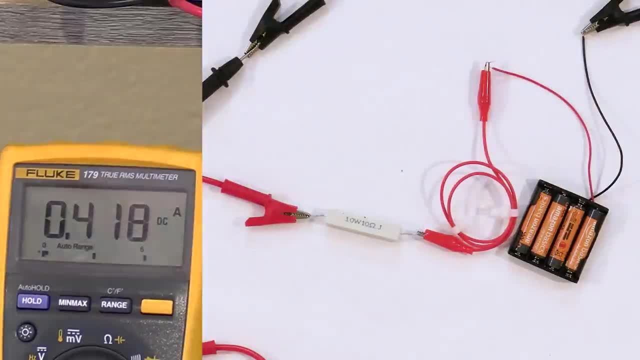 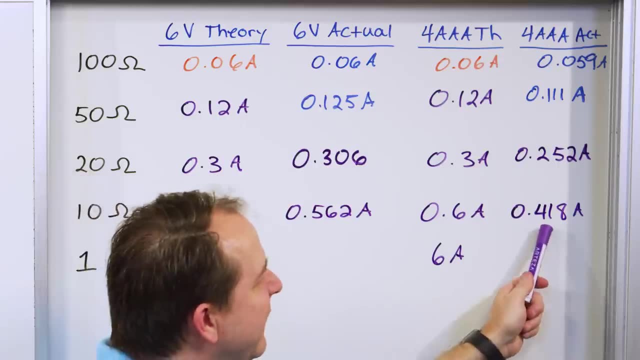 be able to keep up basically at all with this 0.418.. I'm going to disconnect it so we don't drain anything 0.418.. So the small battery was able to provide 0.418.. Now you might say: 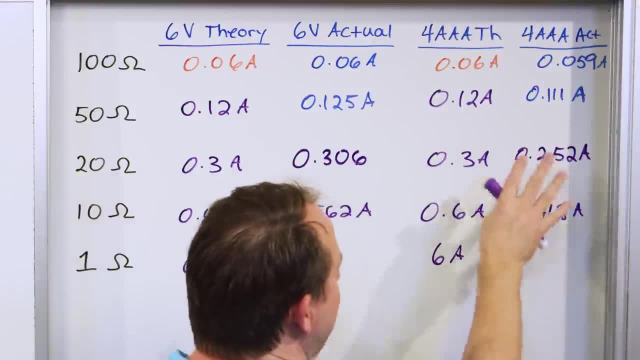 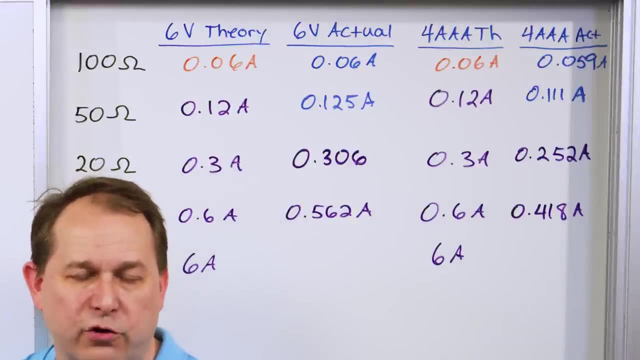 well, wait, what's going on? I thought he said there was a limit here and this battery can't go above the limit, but it's above this one right here. What's going on? What I'm saying is the resistance that's connected externally is- trying to quote- ask for a certain amount. 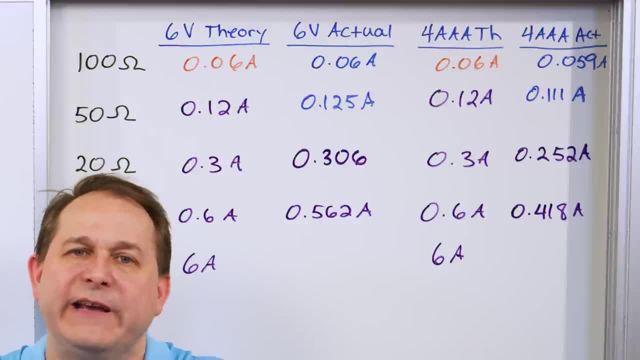 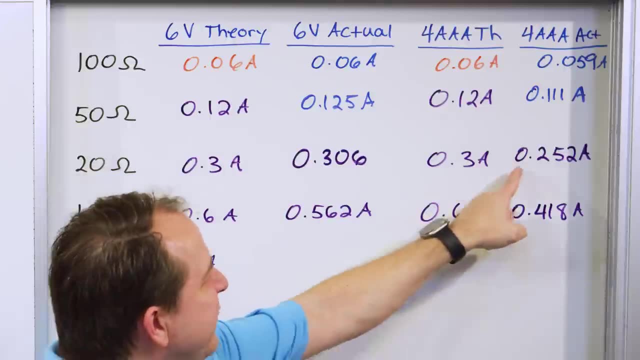 of current in accordance with Ohm's law, And it's able to get as close as it can to that. But what's happening is, as a percentage it can't get as close as it should get. Notice, the percent between here and here is pretty close. The percent difference: 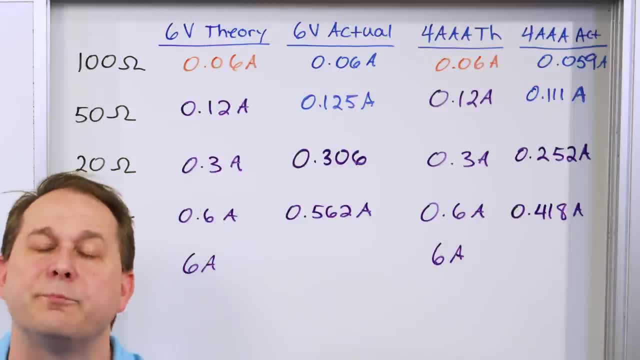 if you were to calculate it between here and here, is quite large. So the percent error in what you're able to achieve with a smaller battery is just not going to be able to keep up. It's going to get as close as it can. What's going to happen? It's going to drain faster and faster and 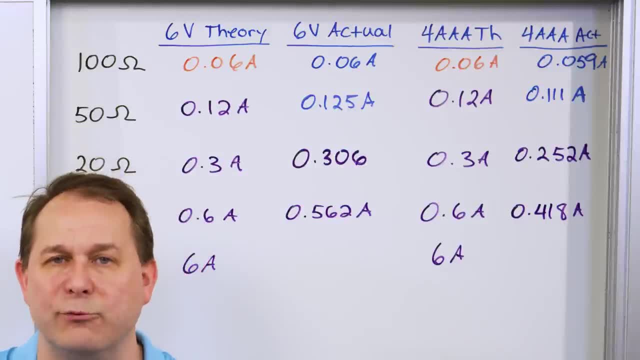 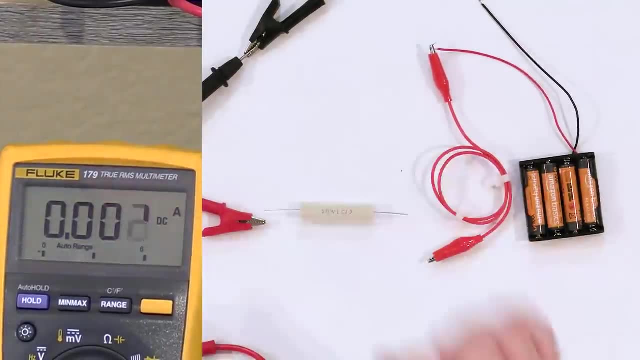 faster as you start asking for that current, because the chemical reaction will deplete faster. All right, let's go down and do our last resistor, which is a single one Ohm, one tiny little Ohm resistance. And so we're going to do that one, And we're going to find out that. 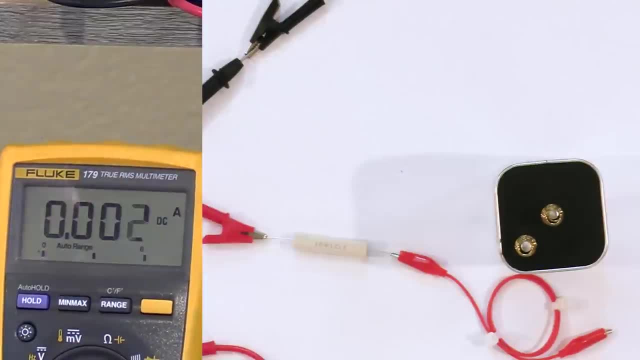 basically, neither one of these batteries is really going to be able to keep up with it. Six amps of current is a very dangerous amount of current. You have to be careful with this kind of thing. Let's see what it can supply. So here we have 2.8 amps, right? 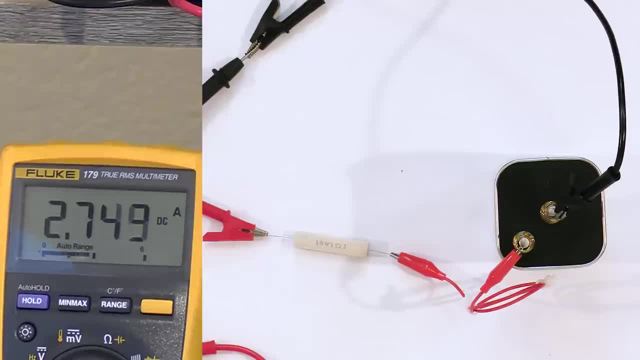 8 amps. So I'll write it down: 2.8, eight. what the two points? it's going down. Notice it's going down, down, down, down down because it's draining the battery. So I'm going to go ahead. 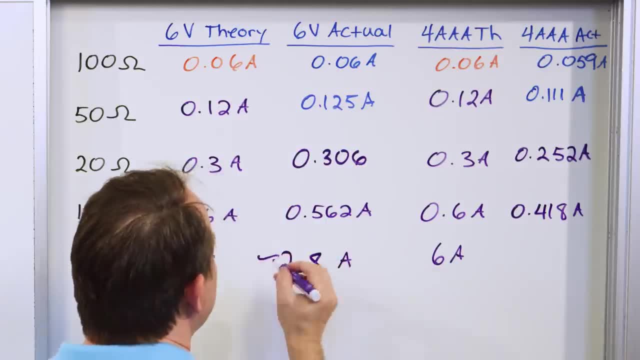 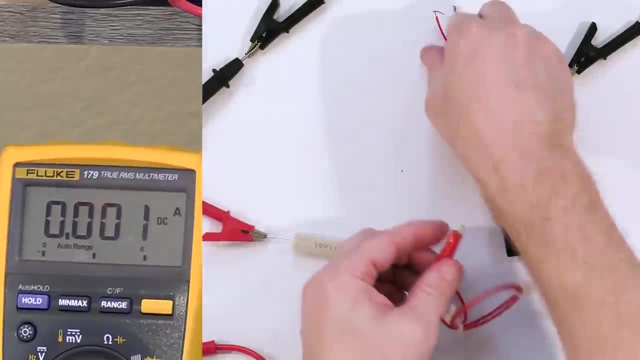 and put it. I didn't see the exact numbers. I'm going to call it 2.8 amps, roughly speaking, And let's see, let's disconnect this one and connect the small battery to it right here and see what this thing does. And I have to be really fast because it's going to drain the super super. 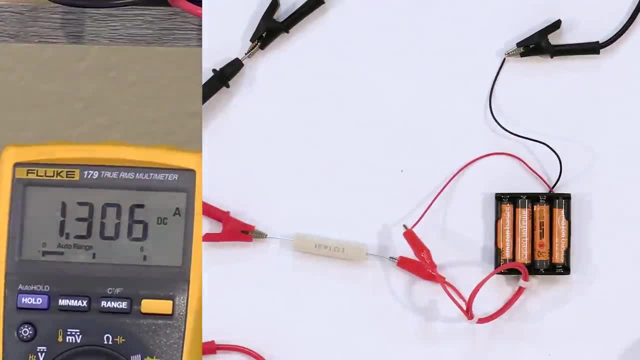 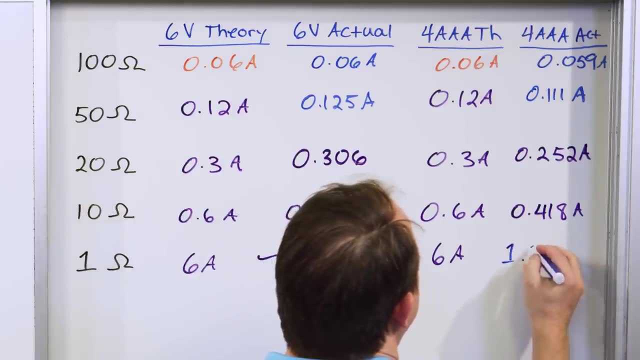 super fast. So when I connect it, 1.3, one notice is going down, down, down, down down because it's draining the battery. I'm going to call it 1.3.. One amps. So 1.3, one amps. Now notice the percent difference, right? If you look at the 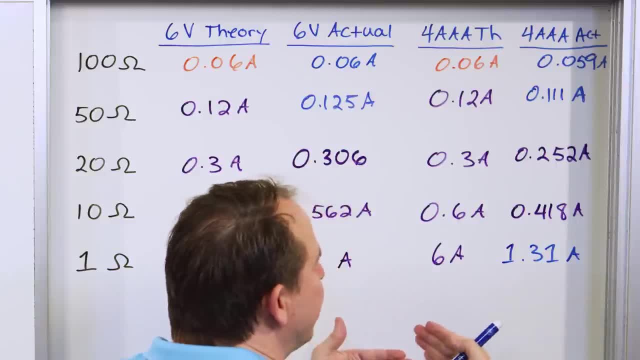 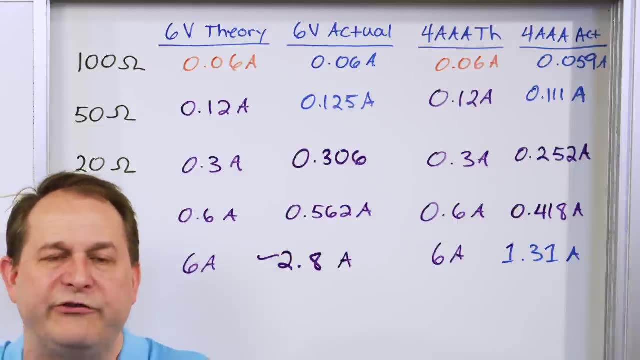 percentage between this and this. obviously, it's not able to get proportionally as close to the theoretical value as was able to get here. So it's not like there's this like hard barrier beyond which the batteries can't. Well, there is always a physical barrier, but what I'm trying 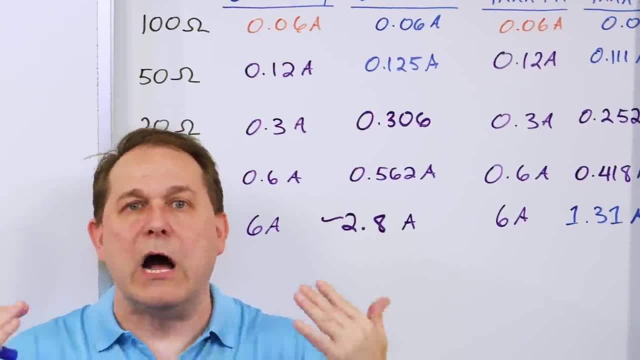 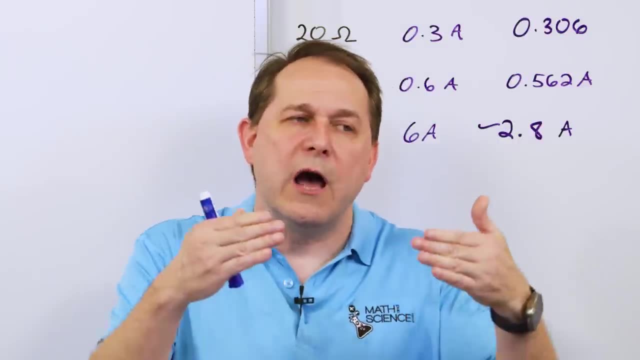 to say is: the point of this experiment wasn't trying to show you. you know, aha, there's a physical barrier beyond which these barriers, these batteries, can't go. What I'm saying is that as you hook a load of a lower and lower resistance, then the battery is going to try to. 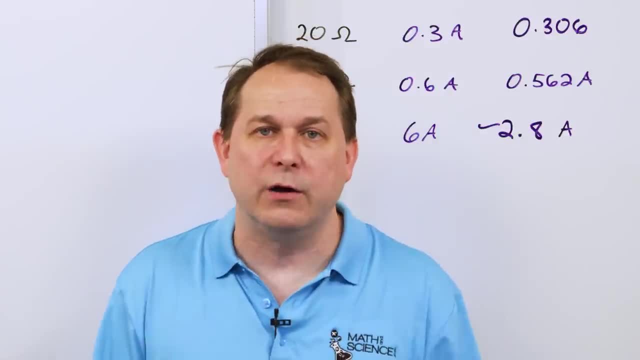 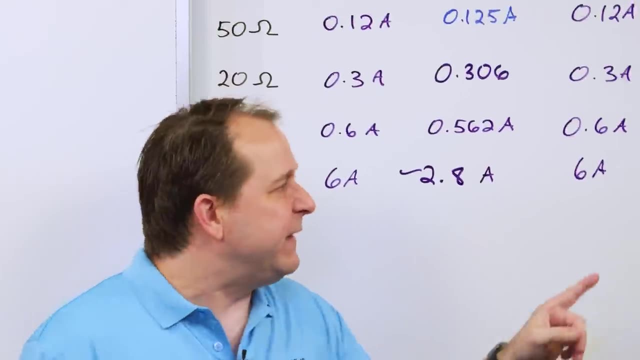 push as much current out as it can to satisfy Ohm's law with that load. But what happens is that as it asks for more and more and more current, it can't keep up with what is demanded. So these small batteries, even though they have the same voltage, a six volt source. 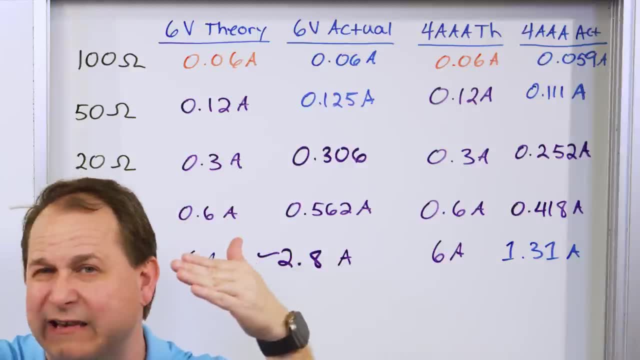 they cannot supply a high enough current and notice that the current was literally bleeding down the whole time because you're literally depleting the chemical reaction in the process And so it's not able to keep up. The large battery was not only able to keep notice, the breakpoint was here for this battery. 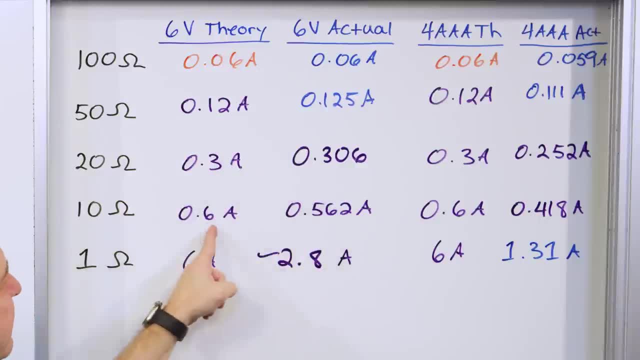 It was able to keep up longer, but also even when it started to diverge. notice this is pretty close still, but when we got it to here is when we we saw a huge divergence. but even this is almost able to supply half the current requested. This is not even close. So the larger batteries can. 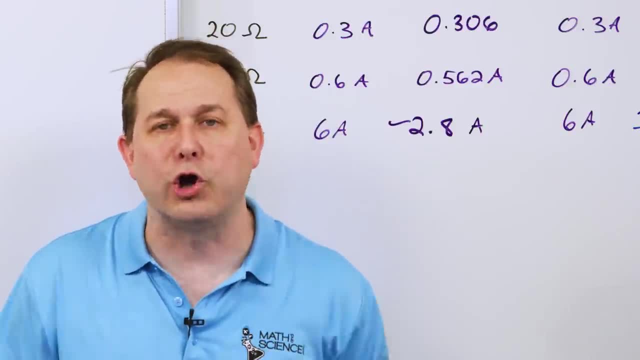 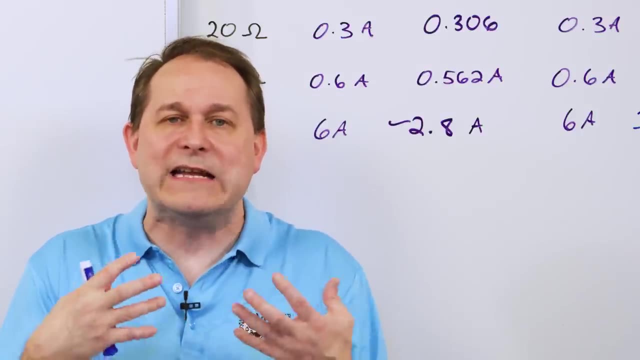 get closer to supplying the theoretical amount of current for a longer period of time, And of course, they'll take longer to deplete as well, because there's more reactants than inside, And so they can not only do that, but they can supply the current for a longer period of. time. So you use large batteries when you need a higher current source or if you just need to supply current for a longer period of time. physically, larger battery can supply current for a longer period of time. You use these tiny batteries for very low current applications. 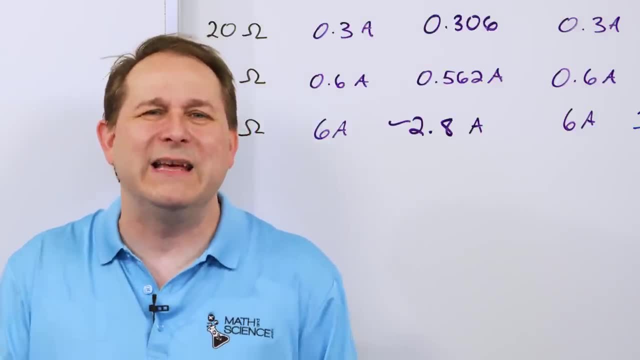 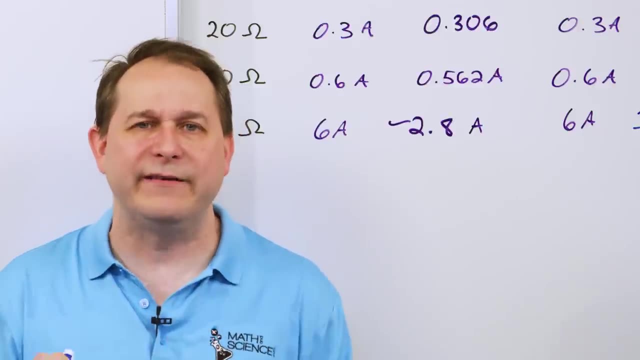 like a remote control. a remote control and a television might take a milliamp or even a micro amp It's. it's just not going to require very many electrons to to to power those little transistors Inside your remote control. So a small battery is sufficient and you can even get away with these. 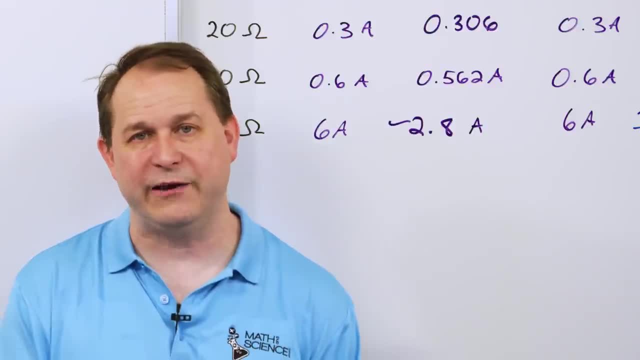 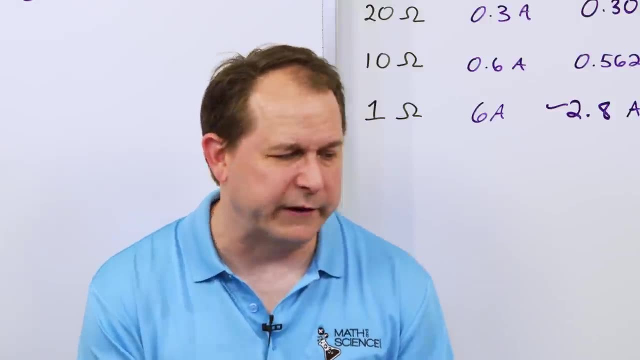 very tiny batteries for these very low current applications. Now there's one more thing I'm going to talk about here. That usually is: is we save it for a little bit later, when we get more detail with circuits? but another way of thinking about this- I think I've described it in terms of how 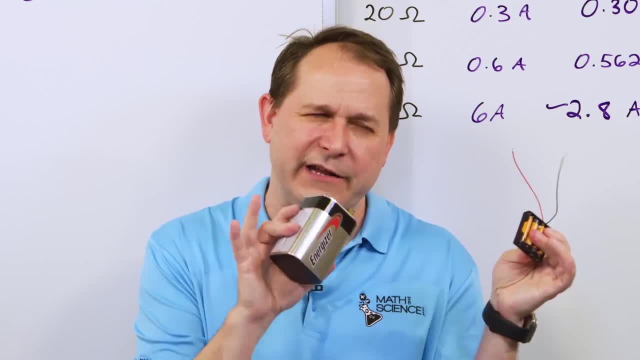 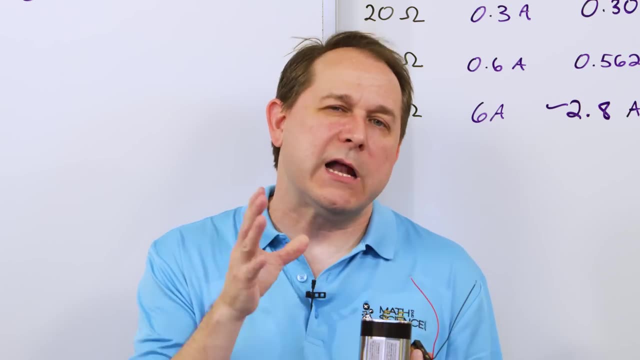 many electrons it can supply. but actually if you- I don't want to get into it now cause it's a little bit too early, but if you draw the kind of the circuit equivalent of an actual battery, you'll see a lot more detail about it. If you only have a bunch of these kinds of batteries. 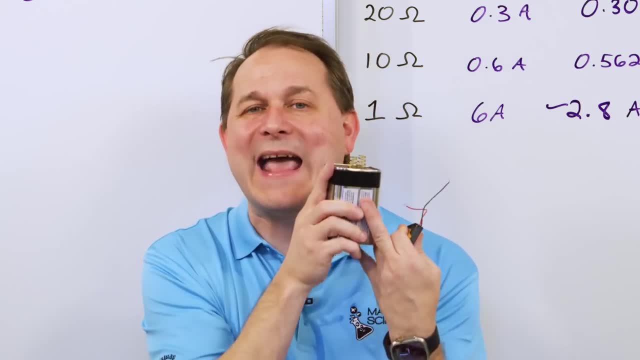 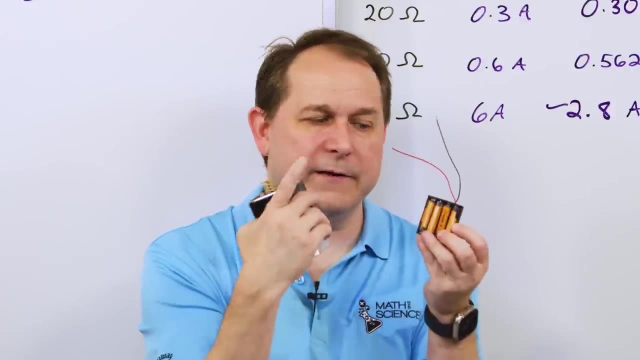 you'll see an ribbed circuit board. that's kind of the invested into it And that's what that's the thing I'm talking about here. The way that you're going to define the distance between the two of these devices is it's going to be, it's going to be written into. 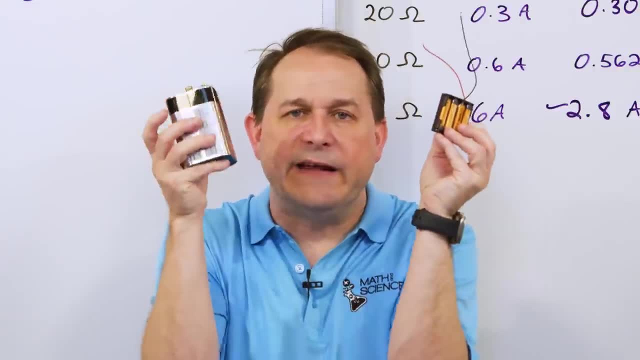 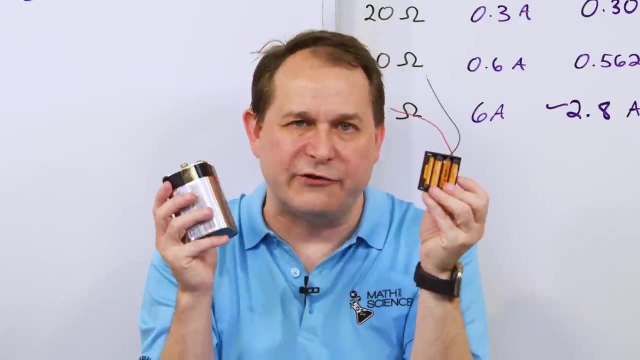 a into a circuit board over the range of a 50 feet voltage or less, And this is another way to think about it. Here's the problem. So there's going to be- this is a very high resistance and it's going to be really really low voltage and it's really almost impossible to handle it as a 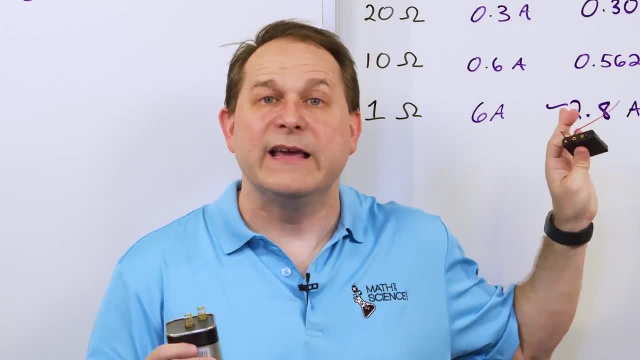 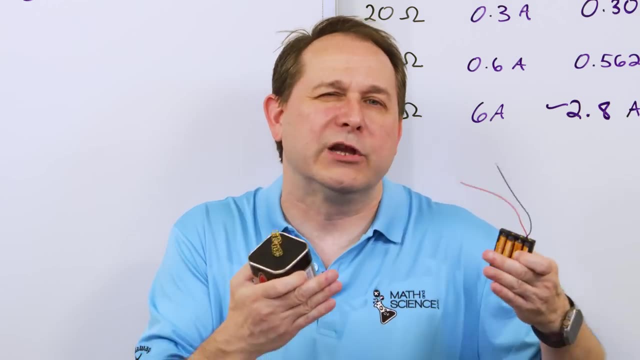 This thing has a lower resistance, So some of this effect can be described in terms of the resistance of the batteries. I'm actually gonna do a lesson later on that process, but we have to get a little farther beyond Ohm's law to understand how that predicts what we're doing here. 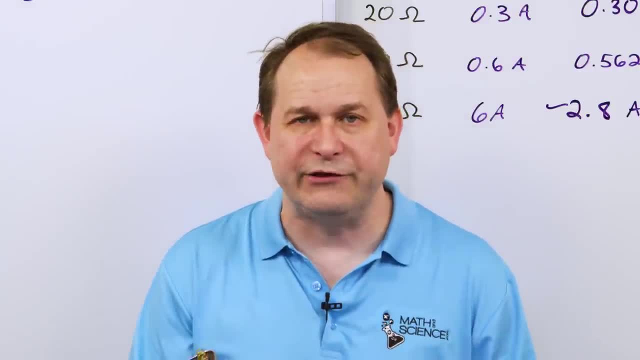 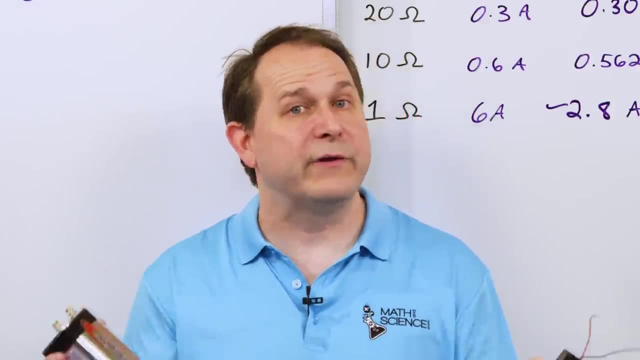 But for now I just wanna say that Ohm's law is a linear relationship between the voltage and the current, given a resistor as the low, which is a linear circuit element right, Different than transistors and diodes- we'll get to later- which are nonlinear. 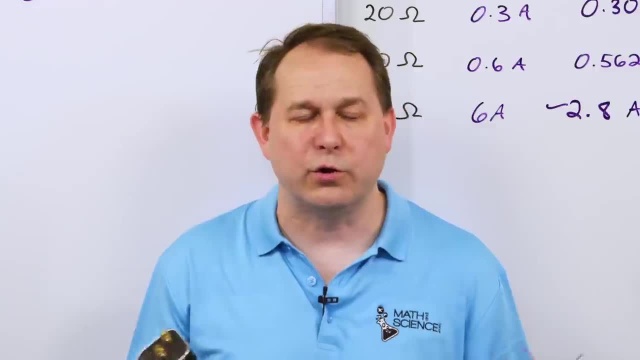 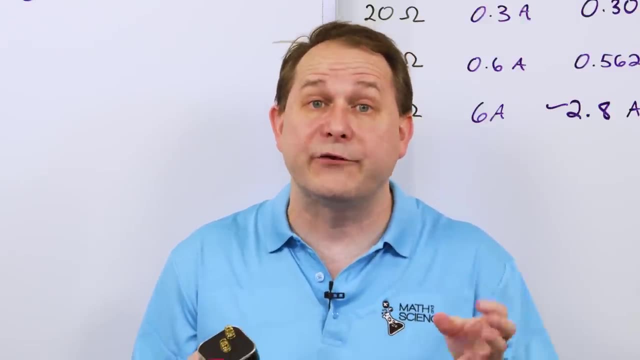 Right, and Ohm's law calculates the theory, the theoretical. The power supply that I'm using over here can supply enough current. It can adjust itself to supply enough current, depending on whatever is asked of it, because it's coming from the wall electricity. 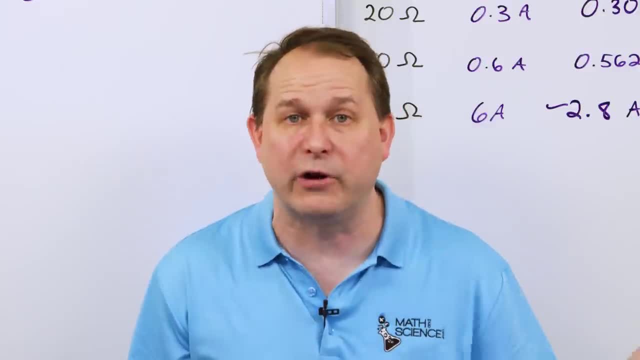 And there's a limit to that as well. I can't have a megawatt of power coming out of this thing, but for anything I'm doing on the bench it's gonna be able to supply enough current in accordance with Ohm's law. 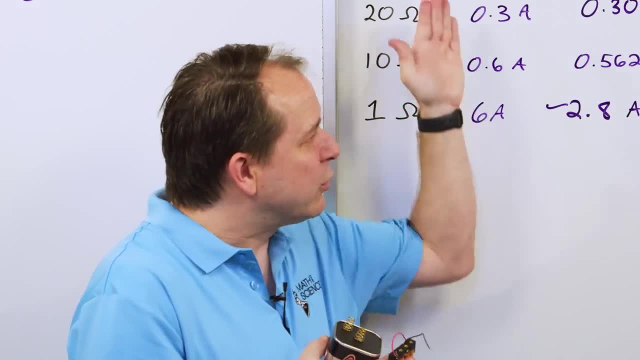 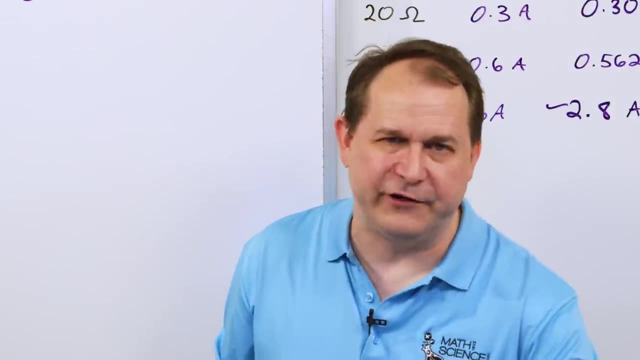 Even though this is six volts, and this is six volts, the theoretical currents that are requested are not always able to be honored, for lack of a better word, So we have to ask ourself the question. okay, if it's true that Ohm's law is always true, 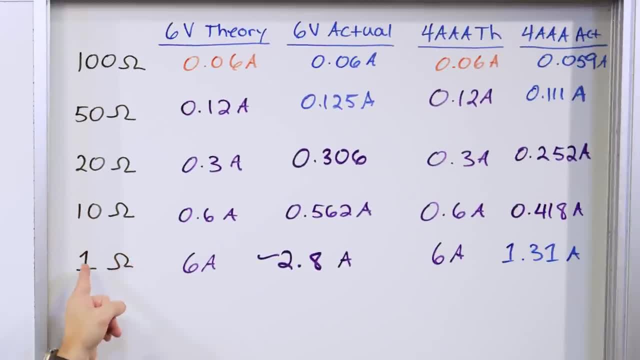 then what's actually going on? If I'm supplying six volts as a source and I'm doing it across a one Ohm resistor, right then I'm calculating six amps. This is what Ohm's law tells me, but I'm not actually getting that much current. 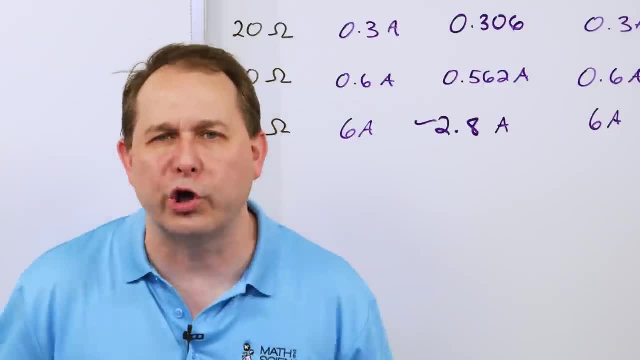 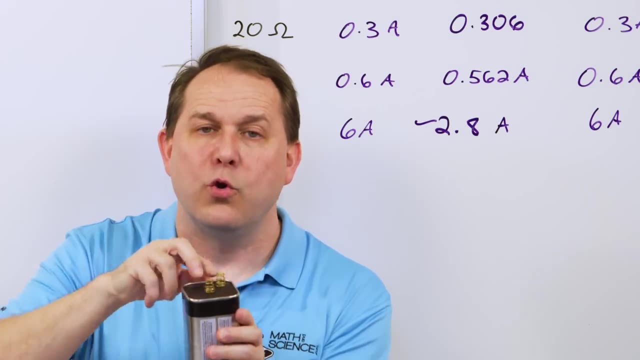 Doesn't that mean Ohm's law is violated? Doesn't that mean Ohm's law doesn't work? sometimes The answer is no. What's actually happening is: if I were to measure the voltage on these terminals without anything connected, I'm gonna get the six volts. 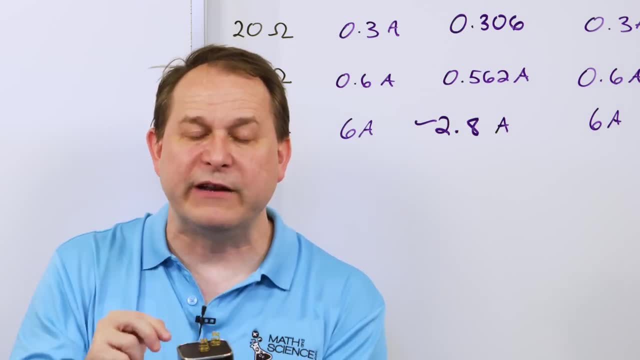 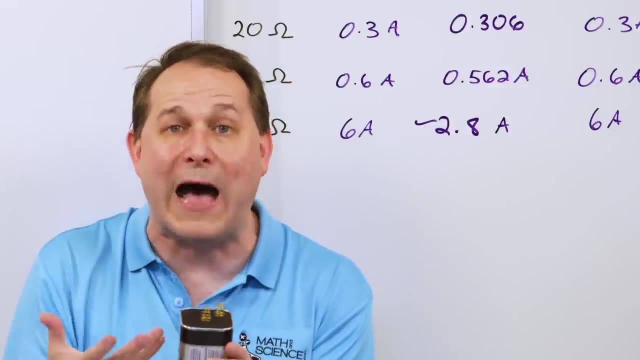 But if I'm trying to demand too much current of it and I measure the voltage while that's happening, I'm going to get something less than six volts. In other words, the voltage will be drooped or drop on this thing when it's unable to supply. 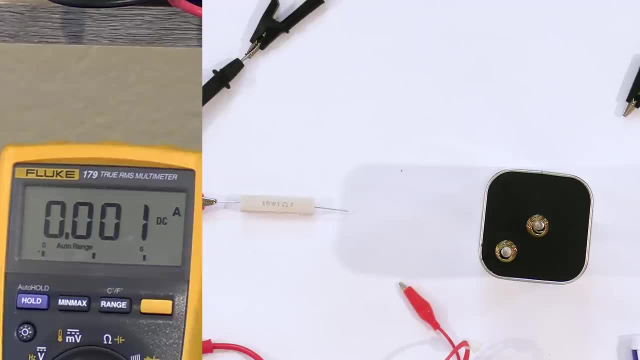 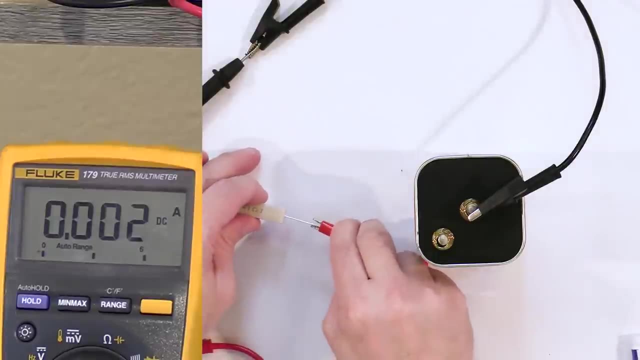 the correct amount of current. I wanna show you that right now. I think the simplest way to show you is to reconnect the six volt battery to it. So what I'm gonna do is connect this here, And we've got it going through our meter over there, right? 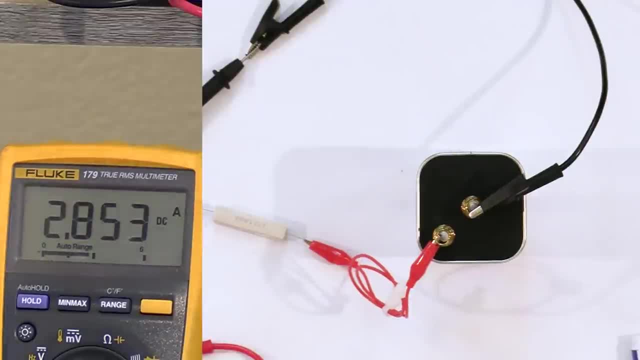 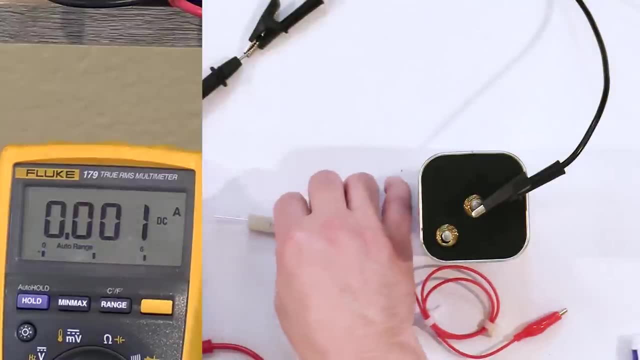 And we're gonna verify again what's going on. We're only getting a little bit less than the three volts or the six volts that we were getting a little bit less than three volts. So what I'm gonna do now is actually disconnect the probe. 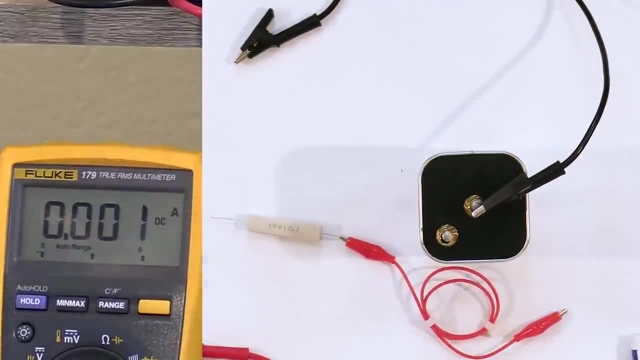 so I can actually measure the voltage while I'm gonna reconnect the circuit, but without the meter in place And I'm also gonna go here. Notice I told you I had to connect it over here to measure current. I'm gonna go back to measuring voltage. 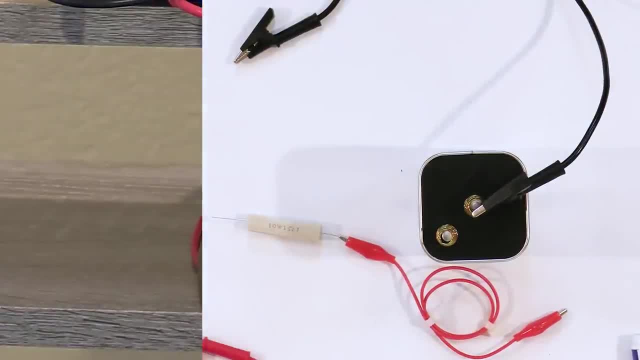 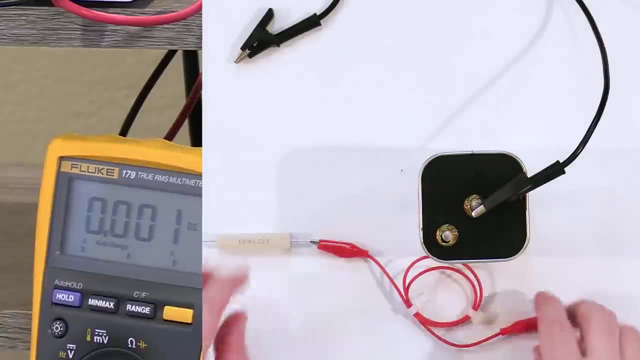 I wanna show you what the voltage on this battery is when it's in operation, So I'm gonna put this up over here, right? And then what I want to do is I wanna hook this thing up, So I don't think I'm gonna need this. 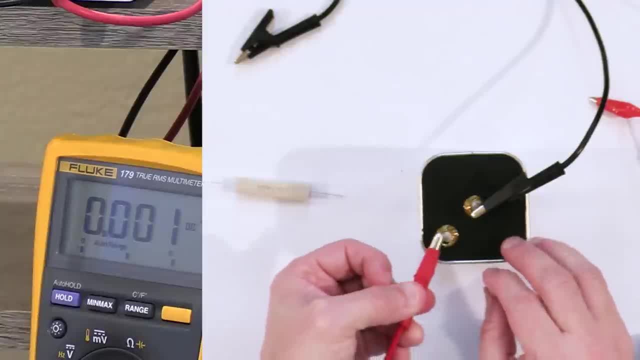 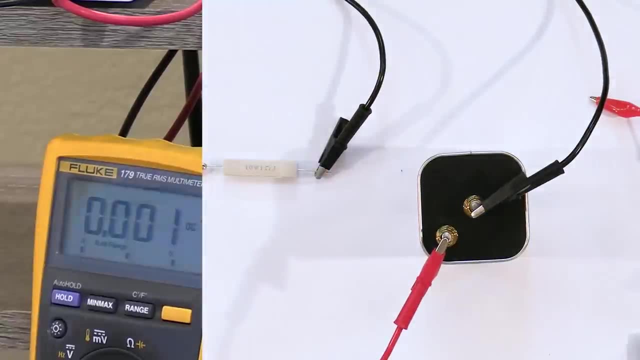 I think all I really need is to hook it across the battery, Right? So we're doing the same thing. I'm just hooking it across, And we already know it's about two, almost three amps, something like that. And now what I'm gonna do is while this thing 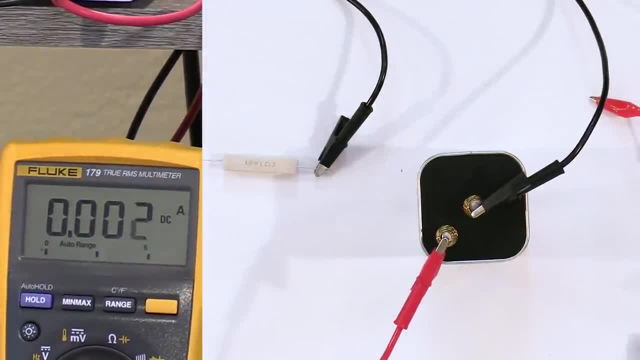 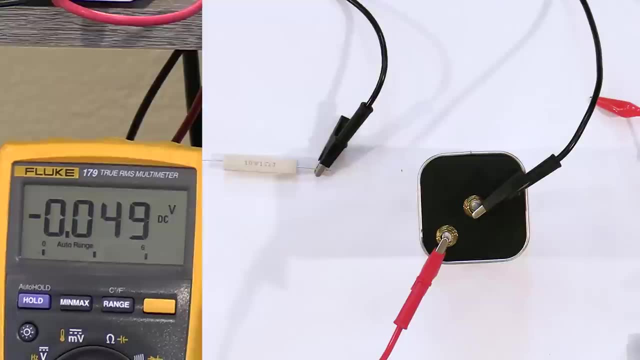 is in operation. actually, let me disconnect it While there is no current flowing. what is the voltage? What is the voltage across here The voltage is, if we look up, we're gonna switch it over back to voltage, So we're gonna go to voltage. 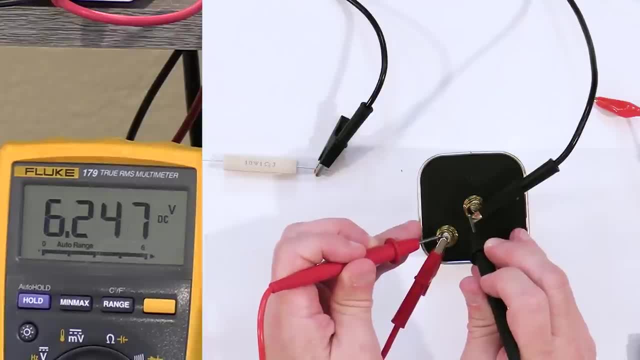 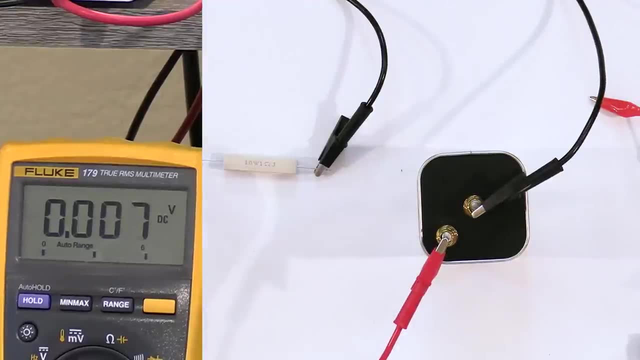 What is the voltage, The open circuit voltage, when nothing has happened? Notice it's already a little bit drained because I've been using it a lot to supply a lot of current, but it's at 6.2 volts. But when I'm unable to supply the current right. 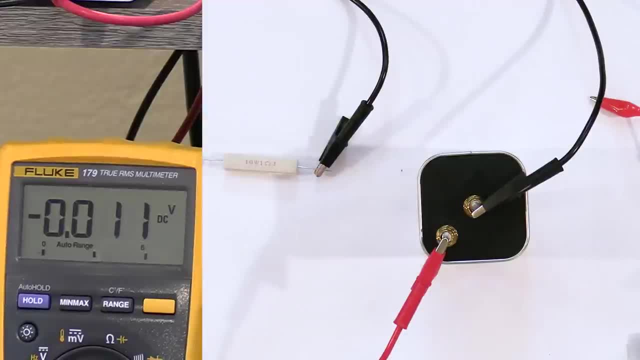 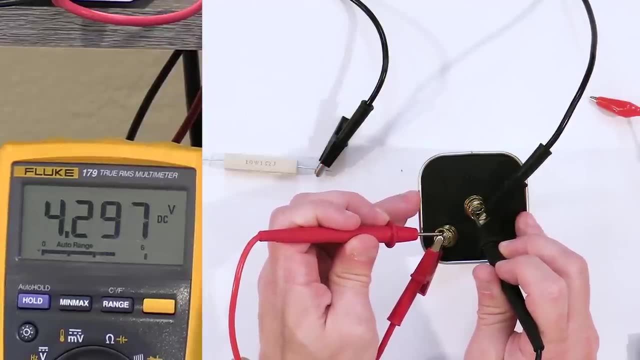 And I'm now asking: I'm getting about three amps flowing through that. What is the voltage? right now? The voltage is not six volts anymore, It's dropped to 4.3 volts and it's dropping even more. So let me disconnect that. 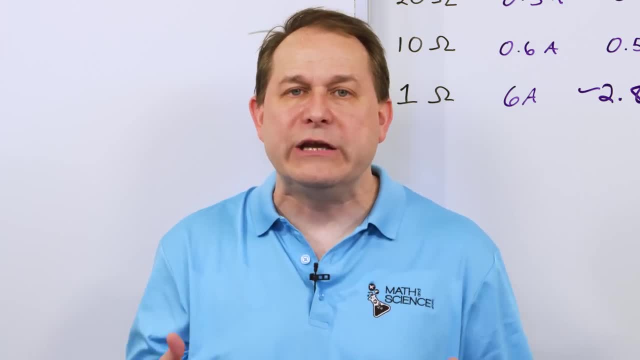 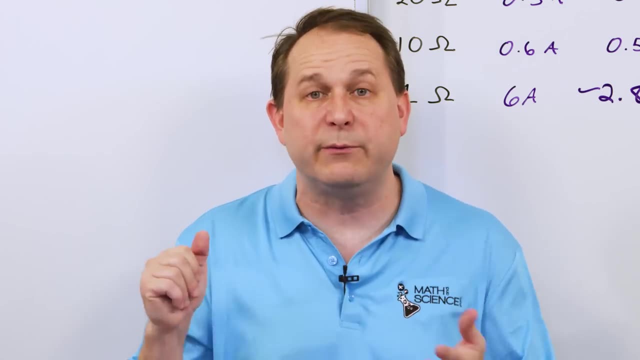 Let me explain that. When you have a battery not connected to anything, you have what's called the open circuit voltage. We saw that it was a little bit over six volts. We were using the battery a little bit, So originally it was 6.4, but then it was just 6.2. 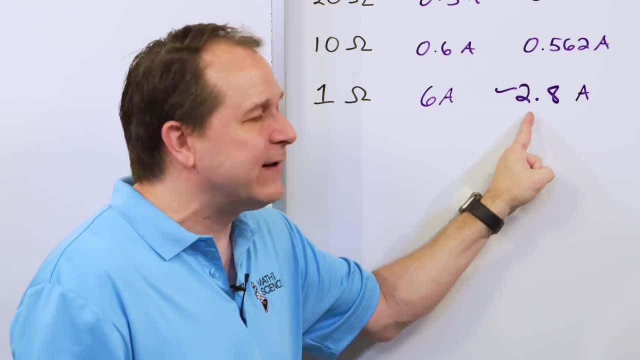 When I'm asking the battery give me six amps And it's like I can't. this is all I can give you. You think it's violating Ohm's law because it should give you this, but it's not. It's giving you something lower. 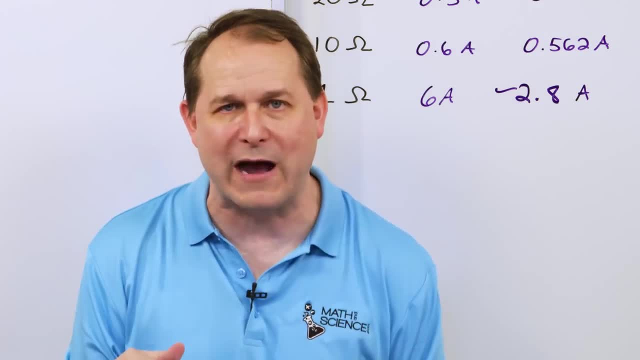 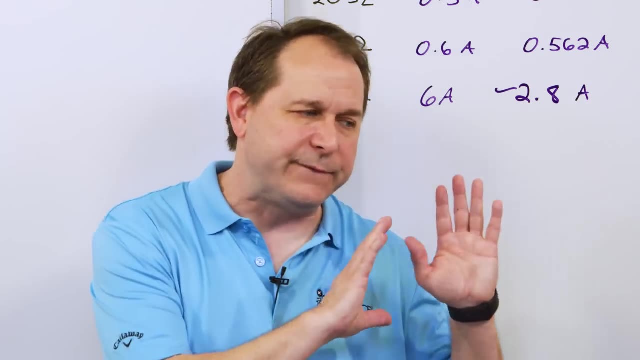 And what happens is the voltage across the battery terminals also drops. physically can't keep up, And you can also explain this in terms of the internal resistance of the battery. in a future lesson I will draw that picture for you and show it to you. 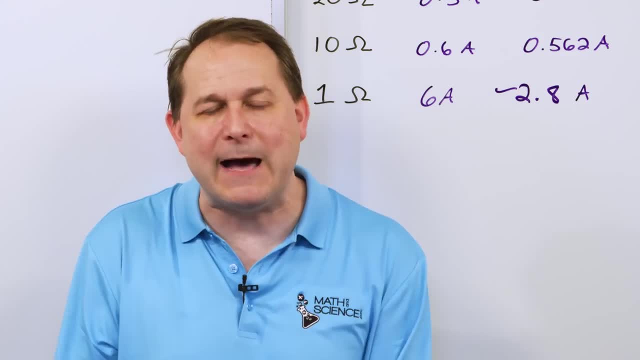 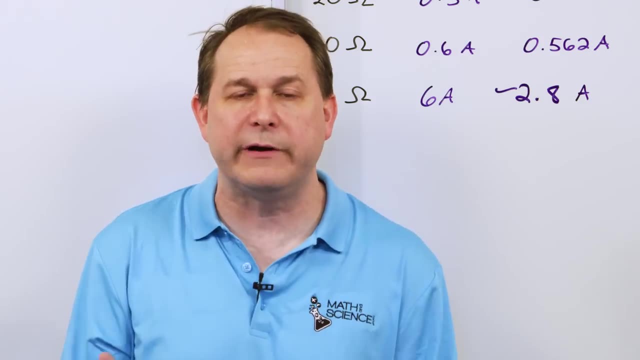 But it's sufficient just to say that when the battery can't keep up, Ohm's law is never violated. The six volts that you thought you had, you didn't really have it, because as soon as you start asking too much current of it. 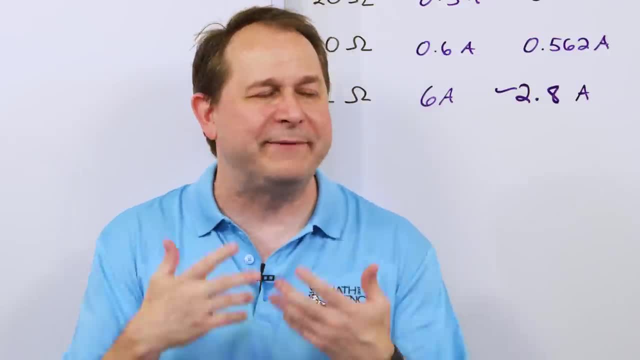 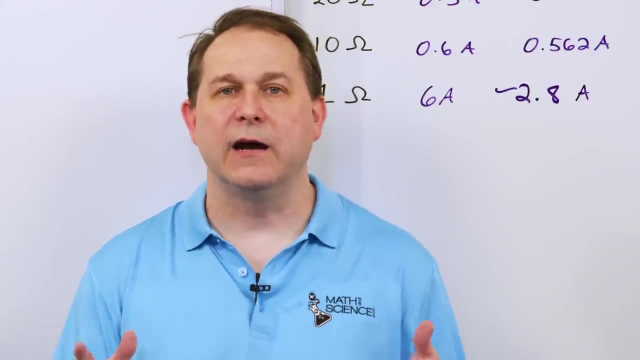 then the chemistry just can't keep up. inside The battery, voltage drops, and that's why it can't supply the correct amount of current. Now, since we're talking about voltage, I can't end the lesson without talking a little bit about AC versus DC direct current. 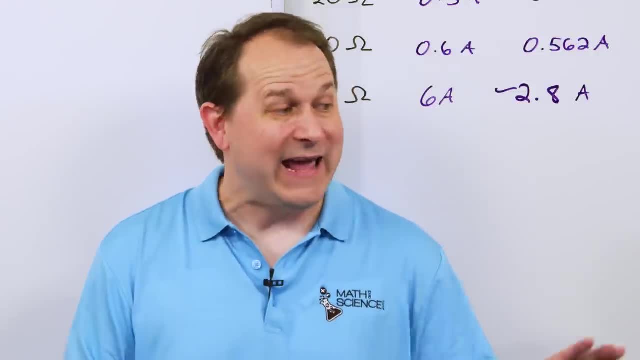 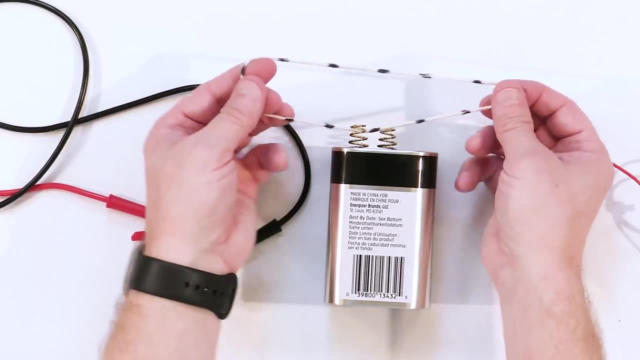 alternating current. this battery, all of these batteries, and including the supply that I'm using here, are what's called direct current. And if I were to use an analogy, if you look at this piece of string here with these lines on it, this, these little dots, are meant to: 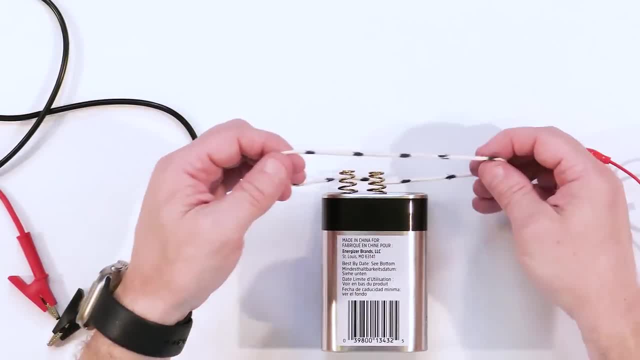 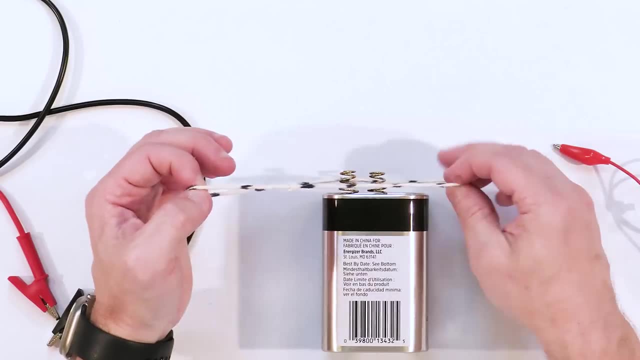 meant to be the electrons in a circuit. And so if I use my imagination and say: okay, it's connected like this, direct current is something that flows like this: It comes out of one terminal And it just goes and goes one direction, over and over and over again. 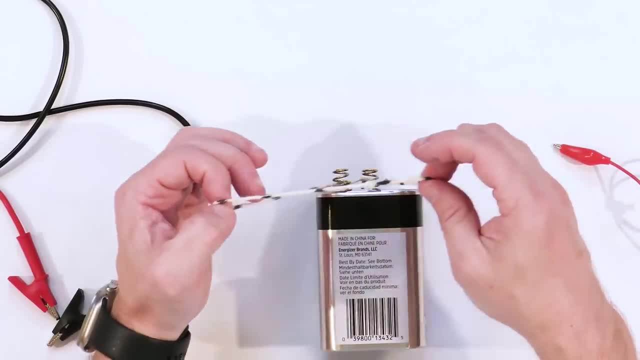 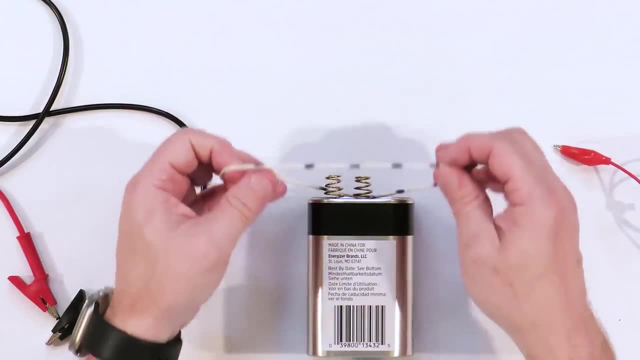 And it just keeps going. The voltage is only in one direction and the electrons are only going one way: over and over and over and over again. direct current, but in alternating current what's happening is things are alternating direction. What happens is the current might flow out of one terminal of the battery. 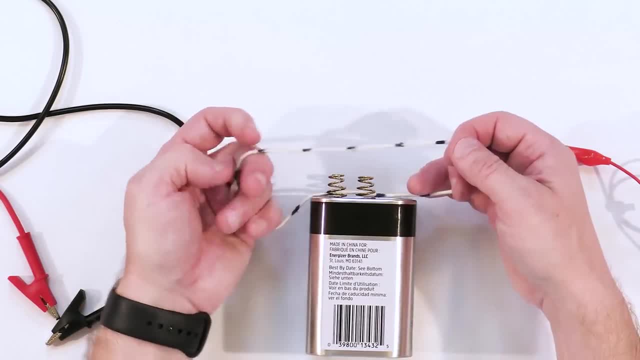 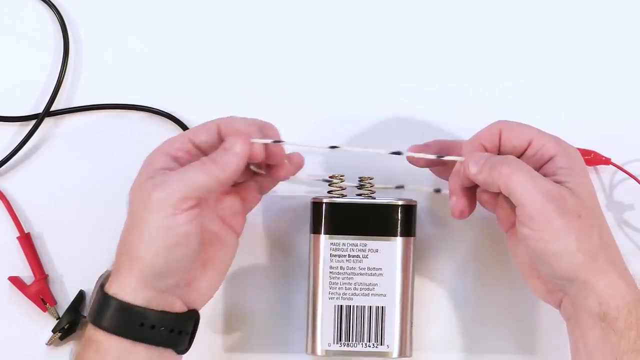 for a little bit and then switch directions and then start going the other direction- the other direction, like this, and then stop, and then switch directions and then come back the other direction, like this, And then stop and then go back the other way and then go back the other. 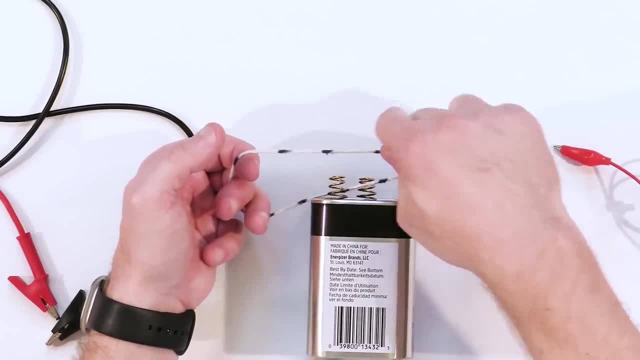 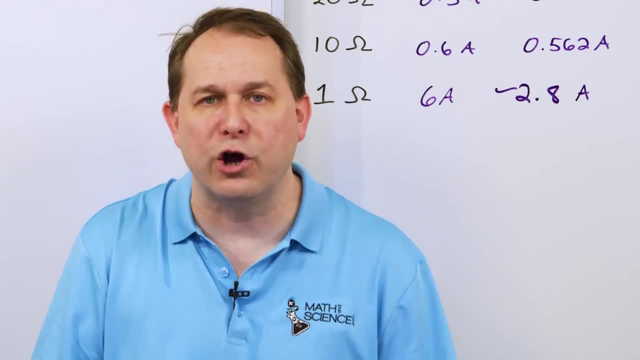 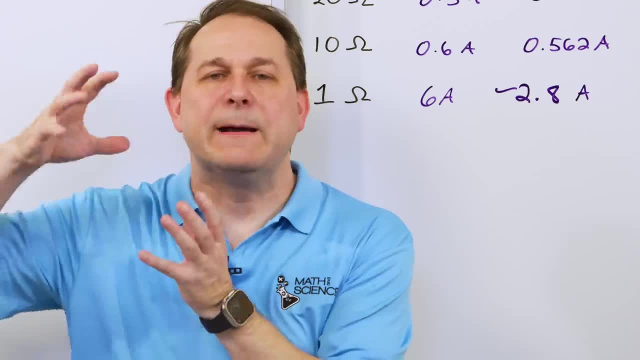 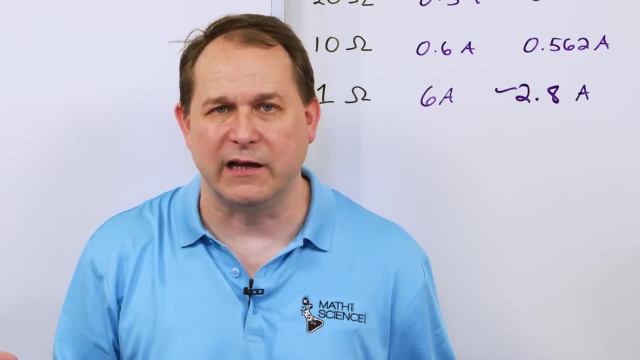 generator. The generator is a coil of wire in a magnetic field and it's rotating and because of the rotation the you get the backwards and forward motion of the electrons. I'm not going to get into it here, but it's because of the rotational. motion of the generators in the large power plants. That's really why we have AC current. Also, it's much more efficient to transmit AC electricity over long distances. If you try to do it with DC, you'll have a lot Of losses due to heat. 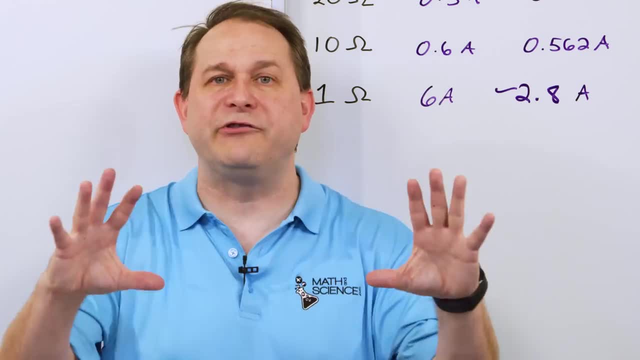 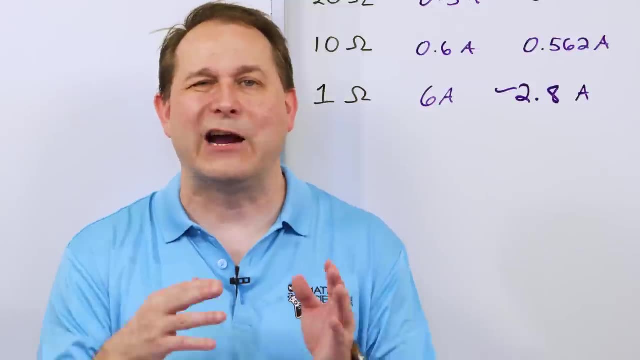 It's not very practical. So we have the generation and transmission in terms of AC. when we get it down into our walls, We also using AC coming right out of the walls, but our portable devices, like our batteries, are all what we call DC, only one direction of the. 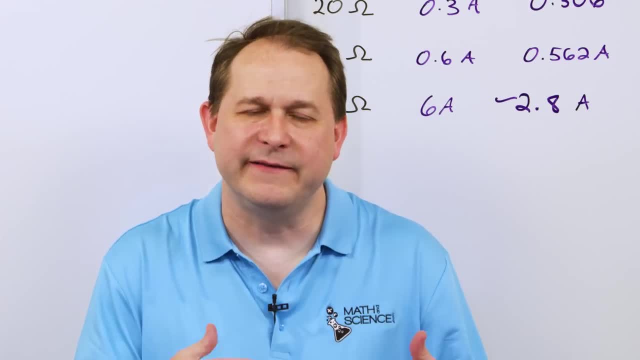 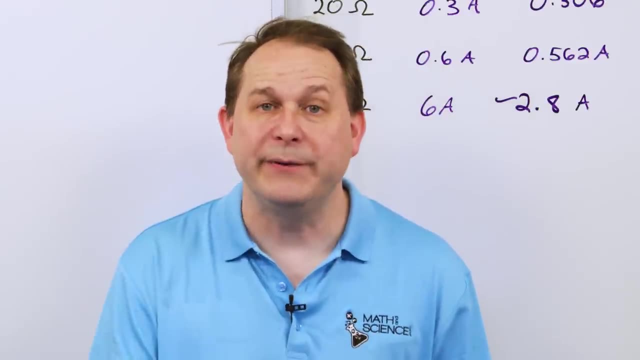 voltage and of the current flow. I hope you've enjoyed this deeper dive into the concept of voltage. I really wanted to focus on voltage, Of course using Ohm's law as well. Next lesson will be on a little deeper dive. look at current and a little 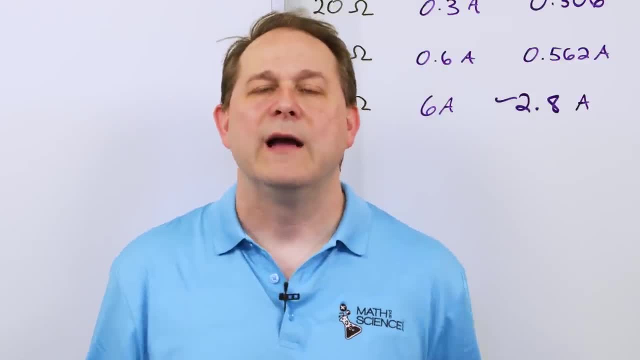 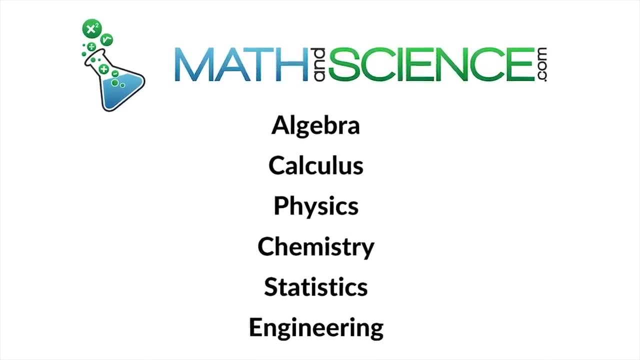 deeper dive, looking at resistance, and then we'll get into more complex circuits. So I hope you've enjoyed this. Please drop me a note, Let me know what you think. Follow me on to the next one. Learn anything at math and sciencecom. 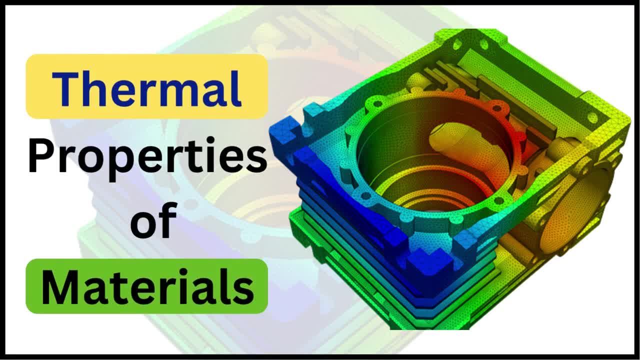 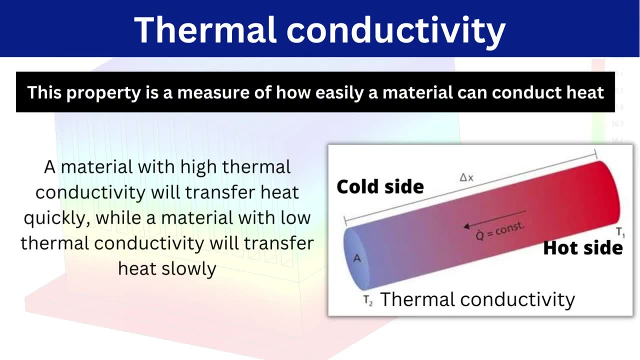 Hello friend, in last video we discussed the different mechanical properties of material and in this video we will discuss the different thermal properties of material. Okay, so let's start the video. So let's discuss with thermal conductivity. Okay, so, thermal conductivity, it is the property of material that how easily the material can conduct the heat.